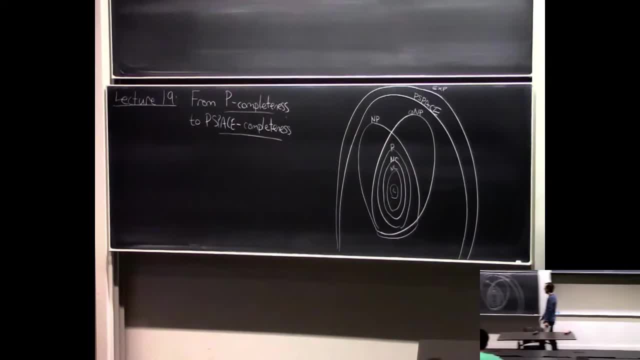 helping understand completeness, even in smaller classes like L and NL and P and so forth. So remember this is this task of finding a complete problems is kind of all about finding the hardest problem in a complexity class, or in a complexity class, the problem that's least likely to be in a smaller class. Okay, so last time, 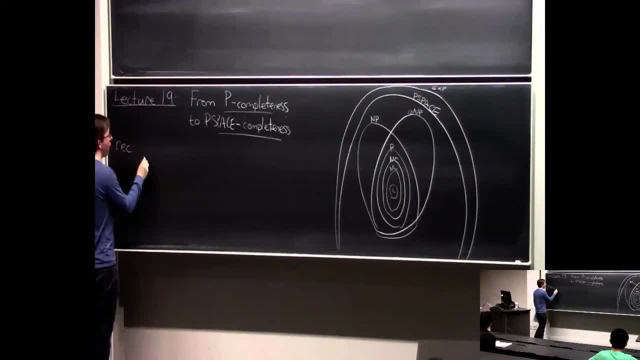 we proved one such result. we proved that this ST path problem, given a directed graph and two vertices, S and T, can you get from S to T in the graph? is NL complete? Okay, so it's like I'm saying it's in non-deterministic log space and it's the 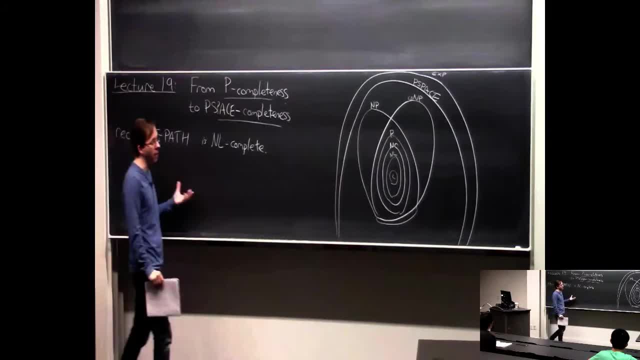 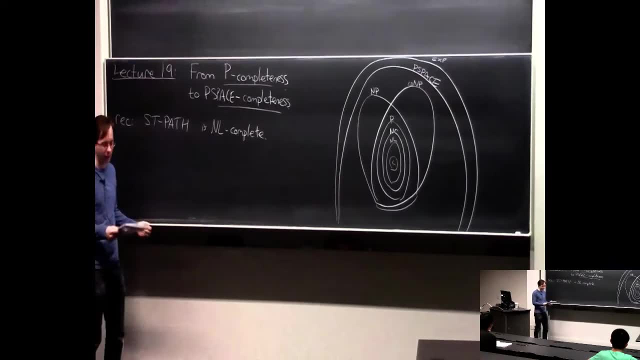 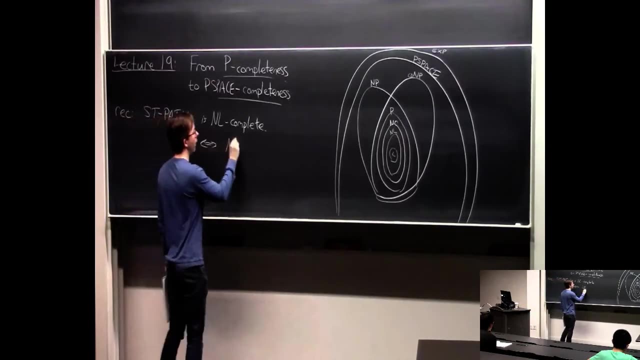 hardest problem in this class, in the sense that if any other problem is in NL is in. sorry, if this problem is in L, then every problem in NL is also in L. Okay, so let me just say that. so it's in L if, and only if, all of NL is contained in L. 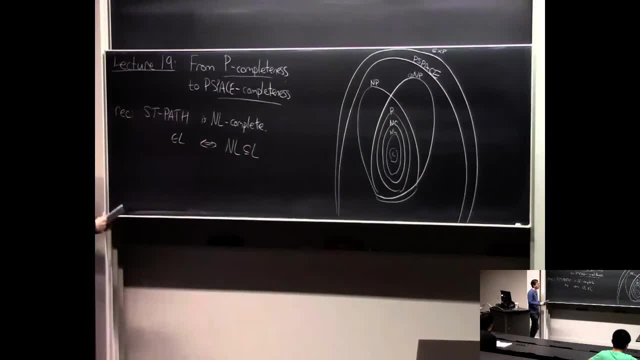 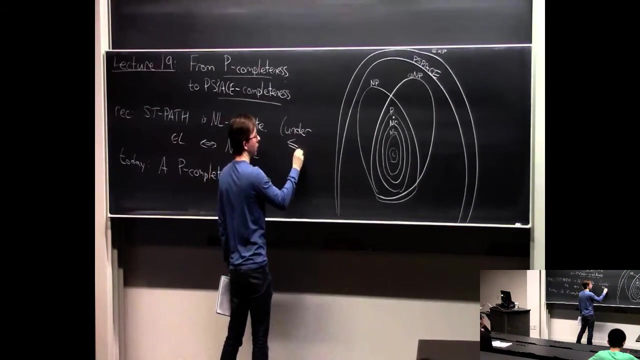 Okay, and today, one thing we're going to do is identify a problem that's here a P-complete problem. So we're going to see a P-complete problem. This will be with respect to log space reduction. So remember, this is NL, complete under log space reductions. Okay, and that's necessary to use those kinds of. 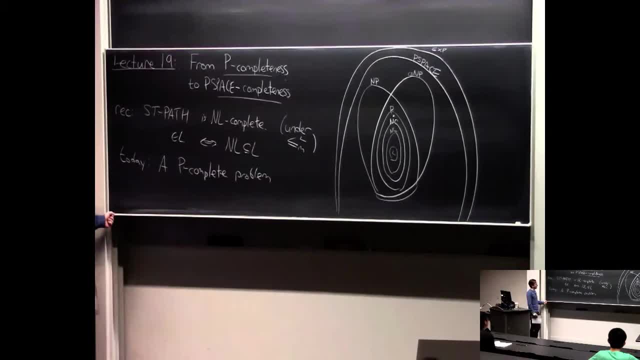 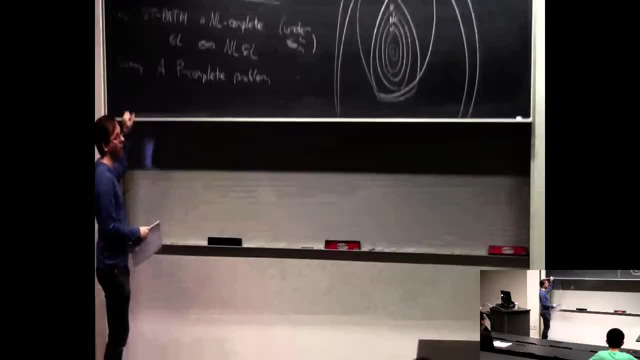 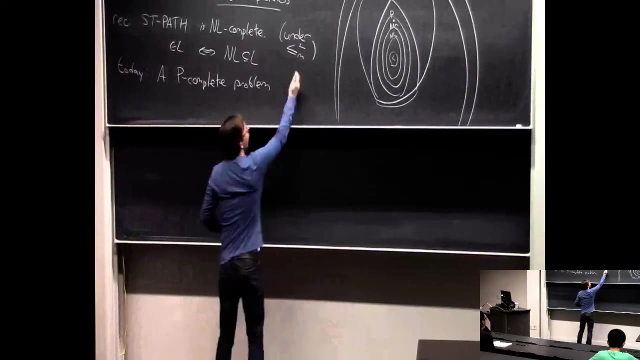 reductions. if you want to get this conclusion about showing things are in L and we're simply going to find a P-complete problem today, also under log space reductions, and that will give us the exact same kinds of conclusions, This problem will be the hardest problem. let me call it C, for now It'll be the 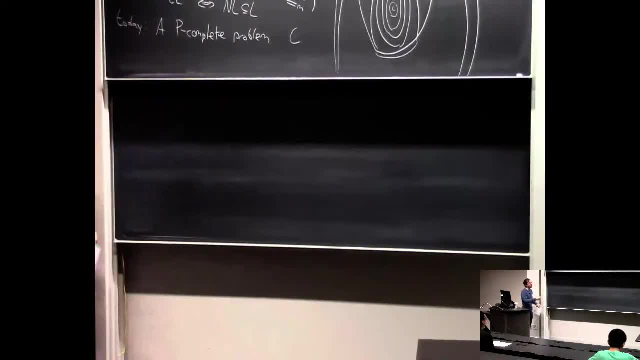 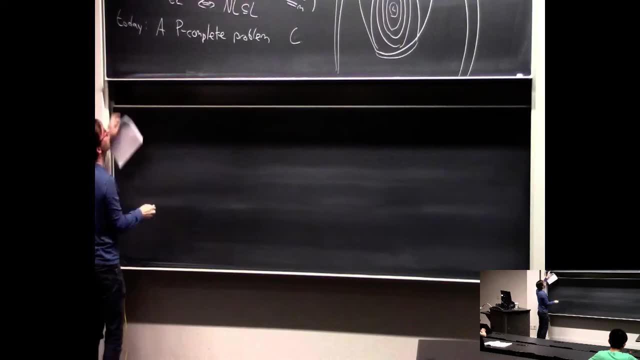 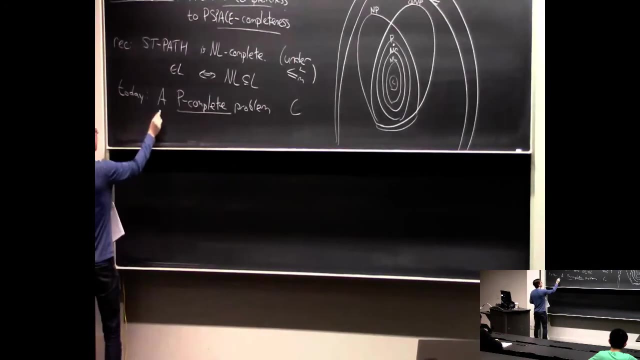 hardest problem in P from the point of view of whether or not it could be an even smaller complexity class. Okay, so this C will have the probability that. well, first of all, let me just say what this means. it means the same thing it always means. so this in particular means that the 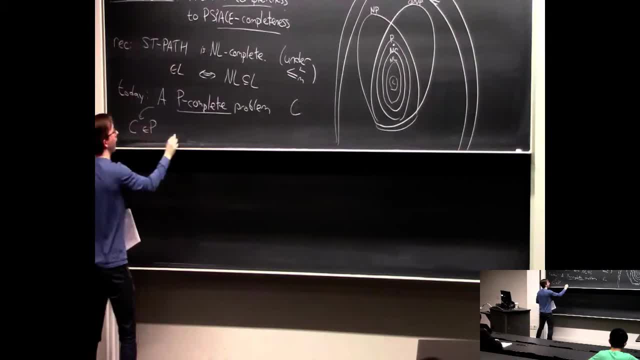 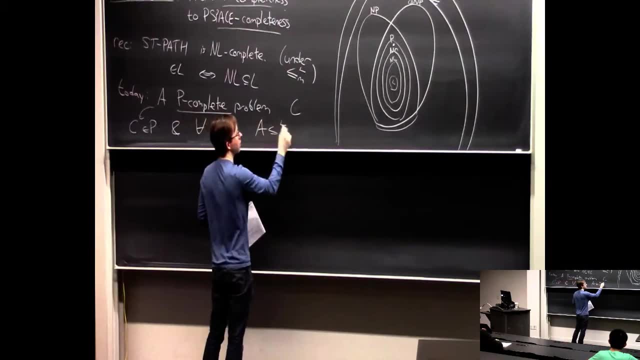 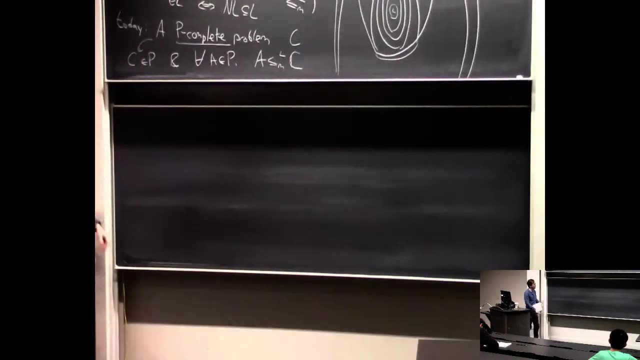 language C is in P and for all languages in P the language reduces in log space to C. Okay, so C is at least as hard as any other problem in P, and from this we can immediately conclude things like: well, C can be put into log space and. 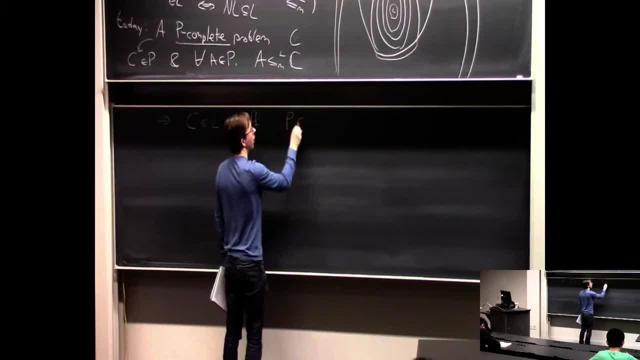 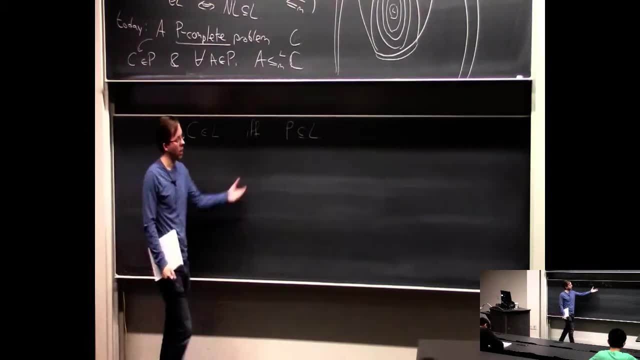 if, and only if, all problems in P can be solved with log space. That's something we actually kind of think is unlikely, that any problem you can solve in polynomial time you can solve with an algorithm that uses a constant number of variables. On the other hand, we don't know how to rule it out, but if you're 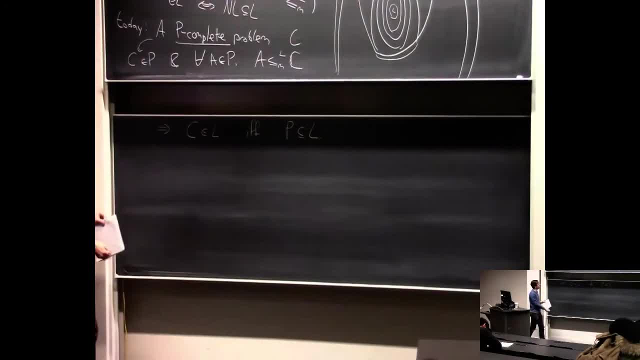 curious to you know. try to find one particular problem in polynomial time that you can't solve in log space. you should go for this P-complete problem C Okay, and it also holds for other smaller classes like NL, if, and only if, all of P is contained in NL. I put another class in that diagram. 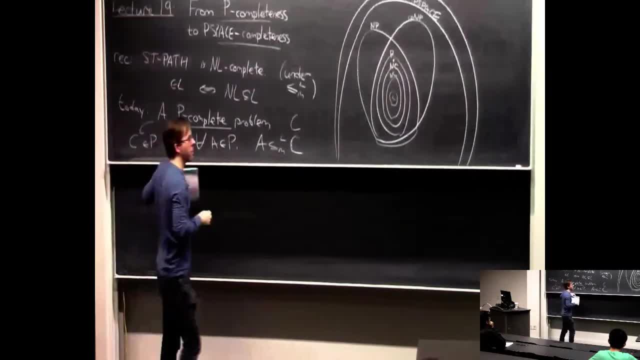 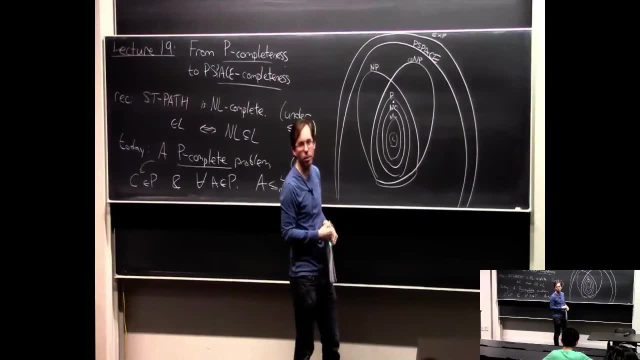 that we haven't talked about yet- NC- and in fact we won't talk about it in this class, but I wanted to mention it at this time. It's some complexity class that's bigger than nondeterministic log space and smaller than P, and at a vague level. 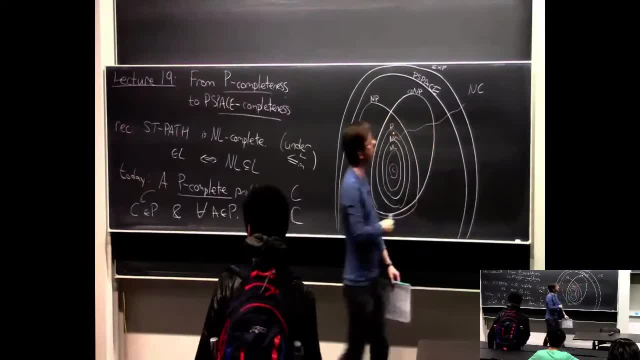 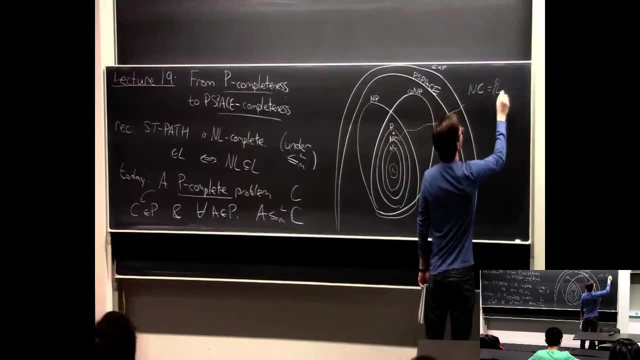 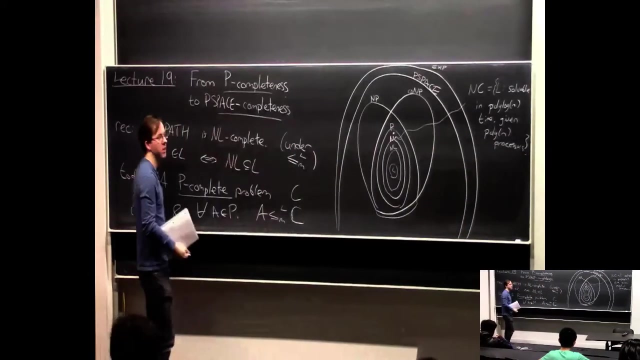 this NC is the class of problems that have very efficient parallelism. It may be able to solve problems in oder algorithms. so, without defining these terms precisely, it's all the languages solvable in Pauli, log and time given, polynomial and many processors. If you have a ton of processors to throw at a 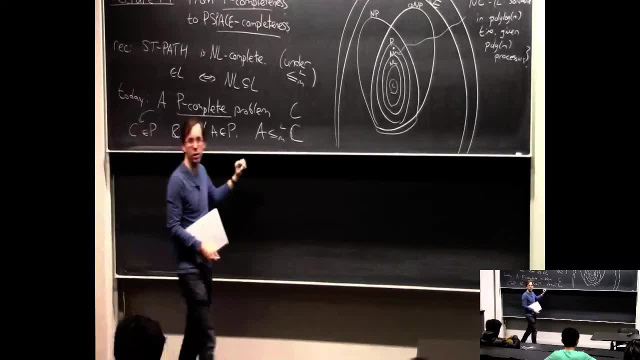 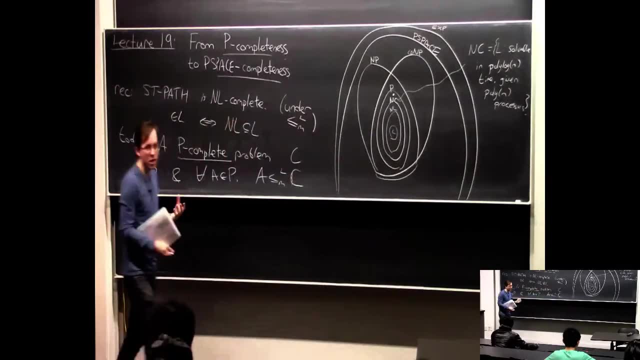 problem. some problems seem inherently serial. it doesn't seem. you can really a lot faster, like in polylog time, And this complexity class NC captures that It's inside P And so, for example, if you're interested in what's a problem, that 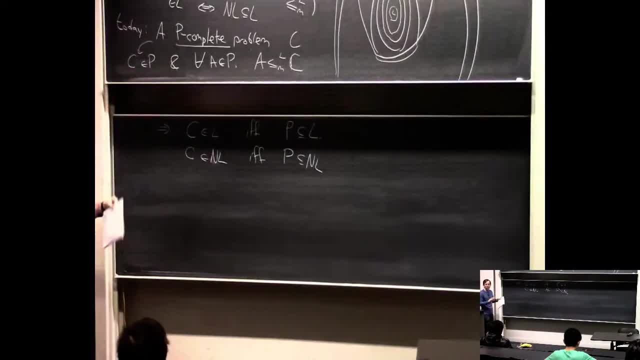 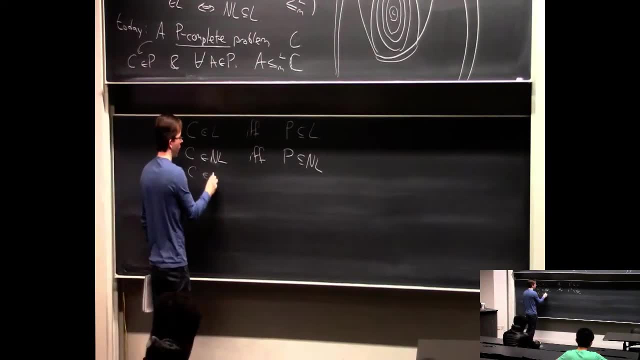 seems like it has the property that having tons of processors doesn't really help you solve it that much faster. well, a P-complete problem is what you're looking for. So this P-complete problem also has the property that's in NC if, and only if, everything in P. 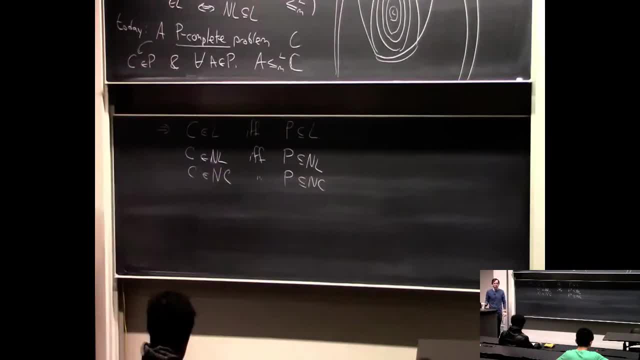 has a very efficient parallel algorithm. OK, so it might seem funny if you first come into 455 to talk about P-completeness, since you're used to NP-completeness and polynomial time reductions. This whole theory of completeness also makes a lot of sense for studying problems within P. 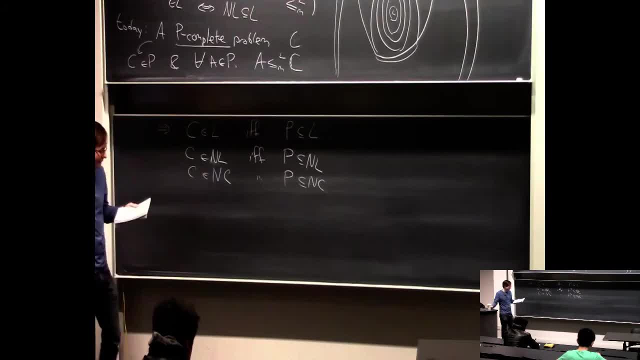 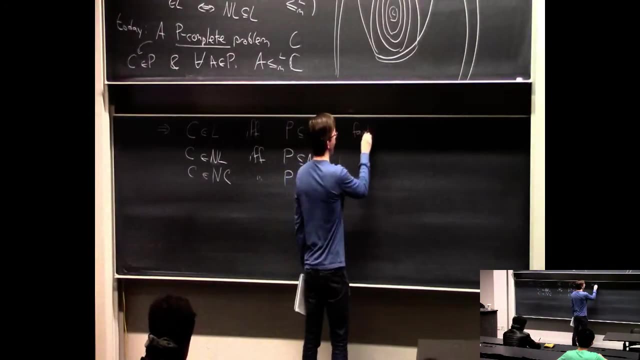 as well. OK, so I left it a bit of a mystery here. What is this language C? In fact, there are many languages that are P-complete, some that we've already studied, So let me just tell you as facts. here are some P-complete languages: 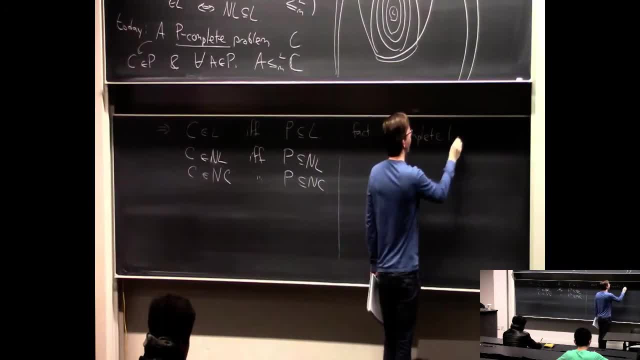 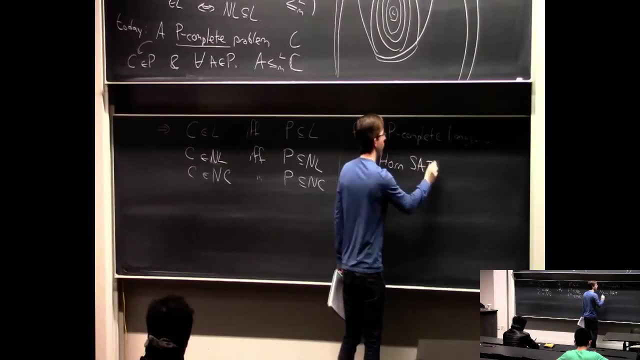 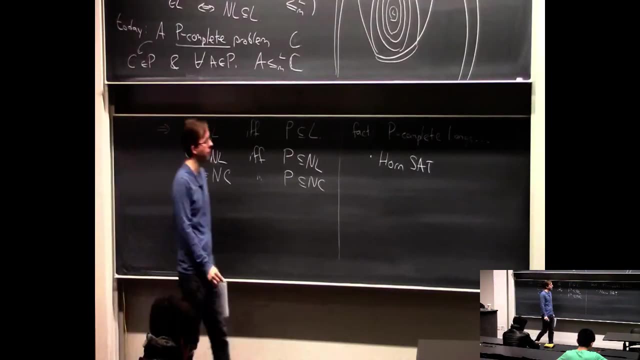 One is HORNSAT. This is a special form of the SAT problem that in some homework- some three or four or something you showed is actually solvable in polynomial time And in fact it's P-complete And I think I'll put that on the homework that's coming up as 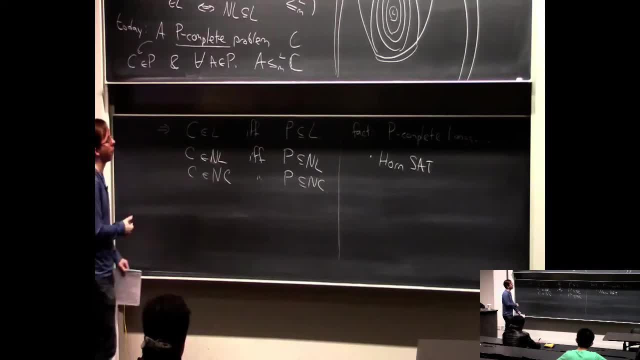 well. So that's an example of one of the hardest problems in P, one that's least likely to be in log space or non-deterministic log space or NC. Interestingly, on that same homework we showed another version of SAT that's in polynomial time. 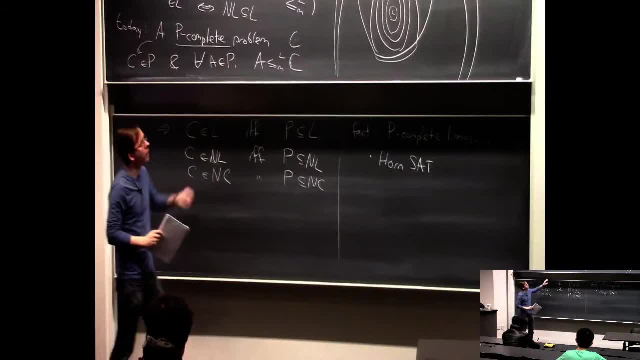 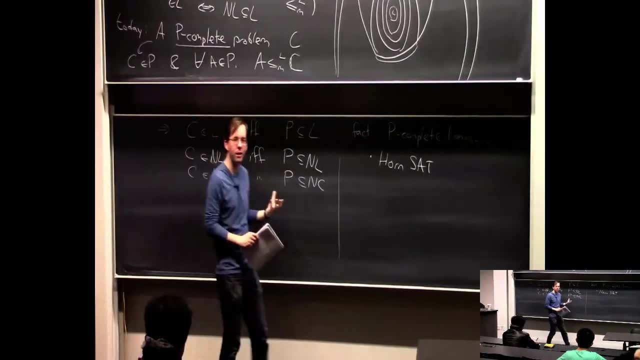 2SAT, And I think even later you'll find out that 2SAT is complete for NL. So somehow 2SAT is. although they're both in P 2SAT and HORNSAT, 2SAT is somehow fundamentally easier. 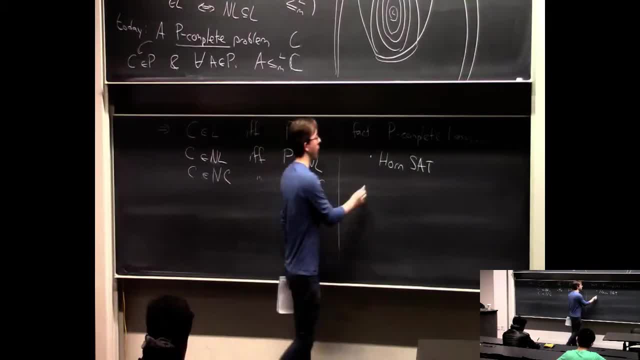 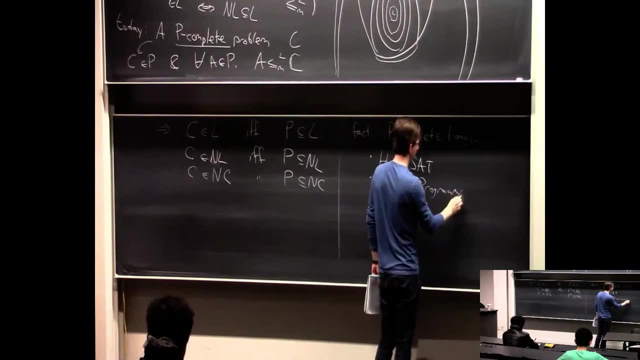 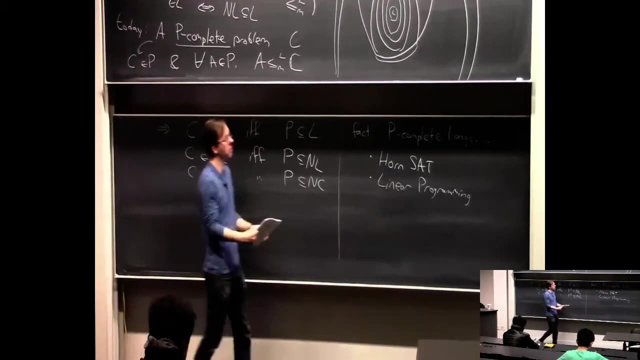 than HORNSAT. Another one is linear programming, which you may or may not have studied already in an algorithms class. This, to me, is like the greatest problem, It's like the most useful problem, that's in polynomial time, And perhaps it's not surprising that it's P-complete. 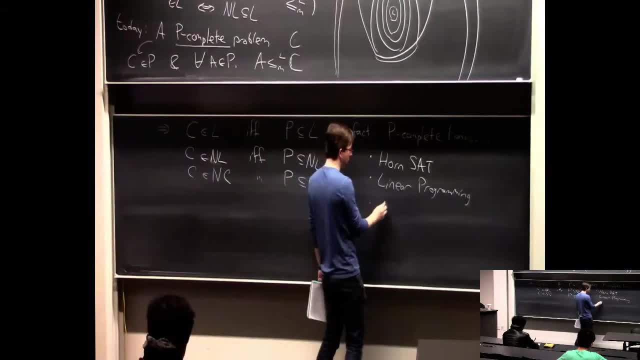 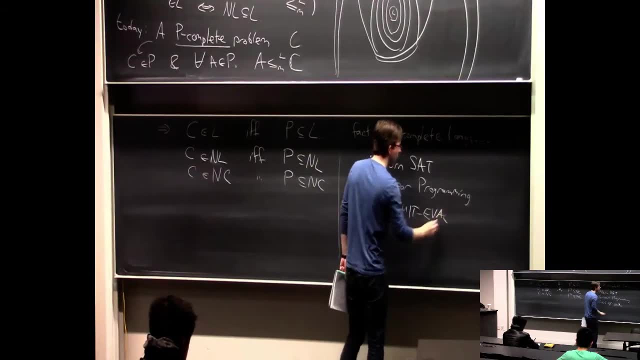 It's very powerful. And finally one I think I've mentioned it before And in fact this is what we'll see today. I don't know why I'm capitalizing this, but somehow the circuit evaluation problem Given a Boolean circuit and an input for that circuit. 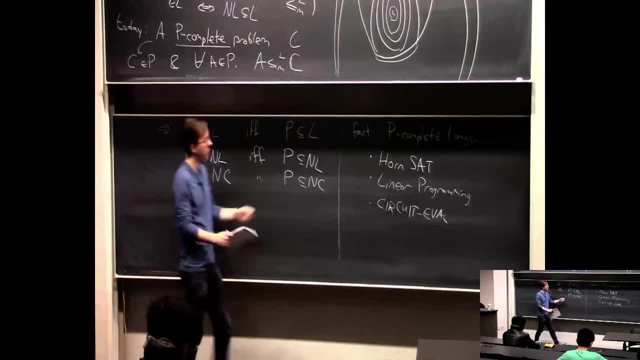 what is the output for the circuit? So these problems we already know are in polynomial time. Linear programming is also famously solvable in polynomial time And in fact all three of these problems are P-complete. They're sort of the hardest problems in polynomial time. 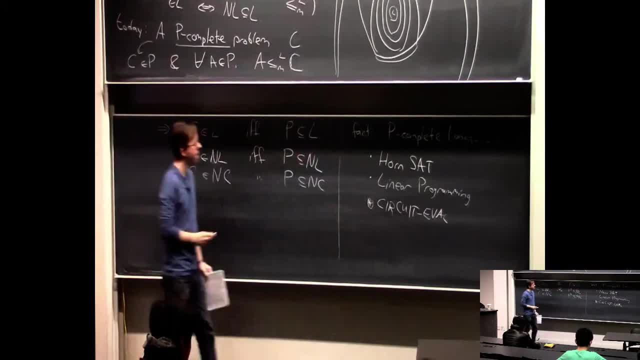 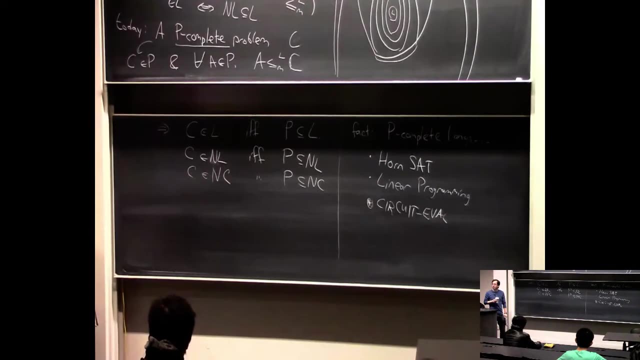 So we'll prove this one today. Questions so far: Well, do you mean depth-first search? So it's not a problem, That's an algorithm? Well, like, I guess the algorithm? Yeah, Is it in the algorithm? 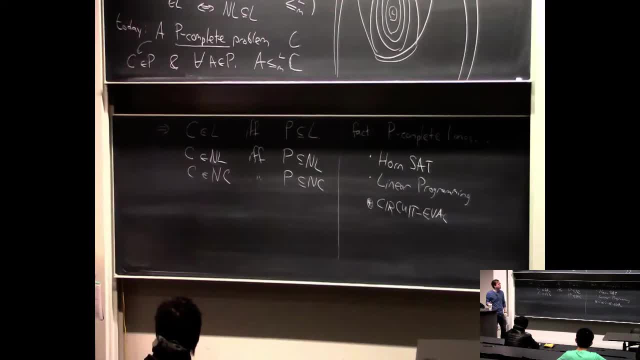 Or can you do it? Yeah, Is it in the DFS parallelizer? Does that fall under this category or no? Well, if by DFS you mean solving the ST path problem And the answer is yes, We didn't really prove it because we didn't actually 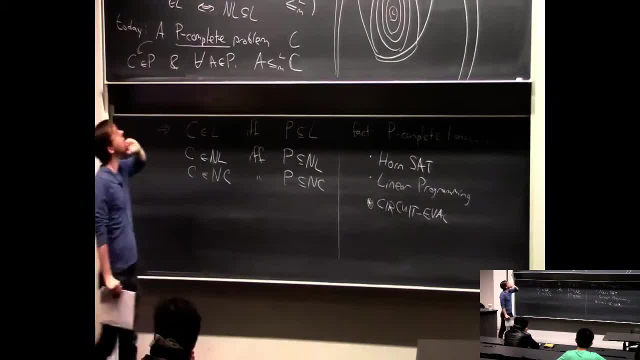 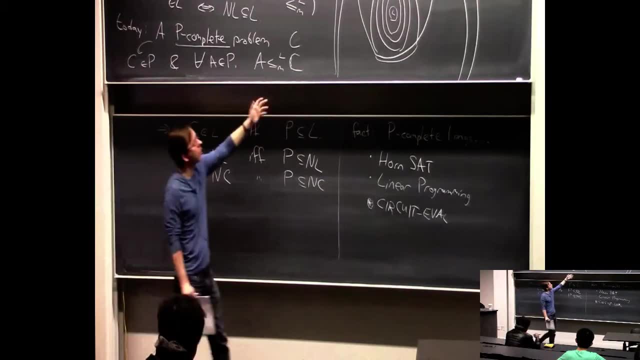 really talk about parallel algorithms, But so, in fact, this problem, ST path- you can have an efficient parallel algorithm for it. in this sense, And if you believe this complexity class inclusion, we know that ST path is in And now. so if you believe that this NC class contains NL, 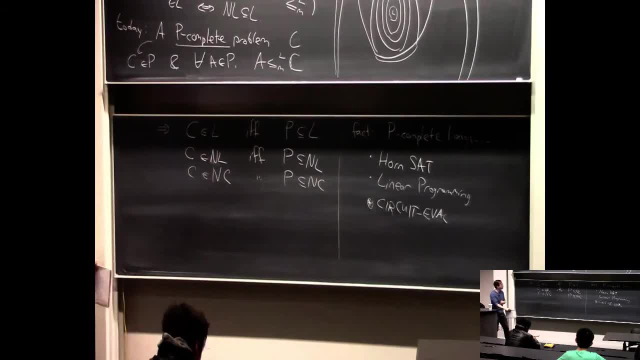 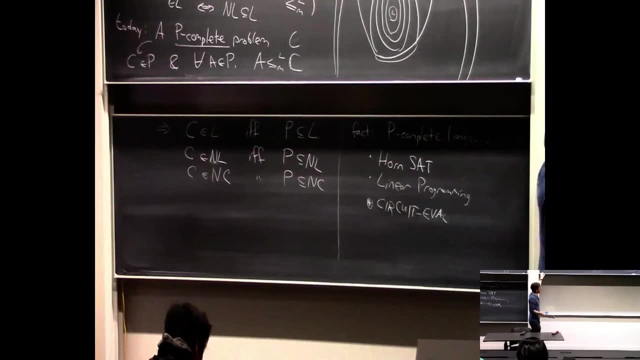 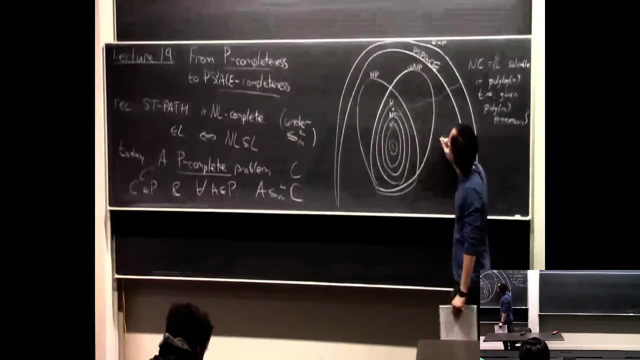 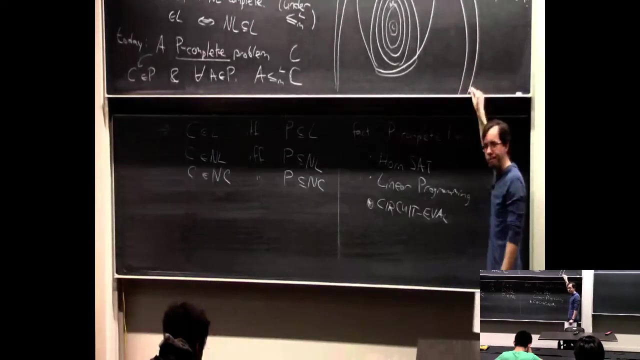 then it follows. So yeah, So today we're going to get to this, And then we're also going to similarly find a problem that's in here, a problem that's in PSPACE- It's unlikely to be in, let's say, P or smaller classes. 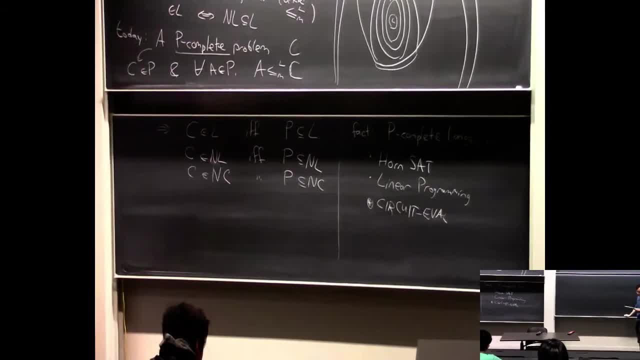 So complete problem for PSPACE. Now, before we get there, let me ask you a question That'll get us into some interesting directions. We always, in the theory of NP-completeness we say, oh, a classic NP-complete problem is 3SAT. 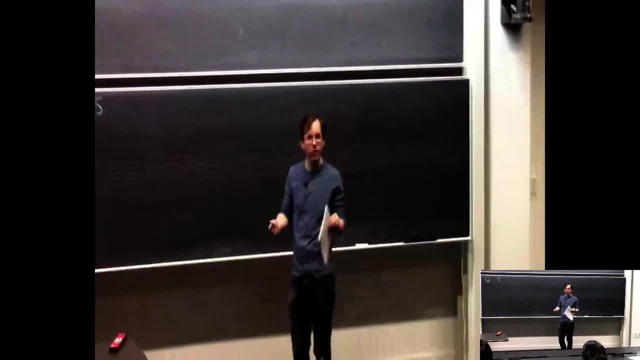 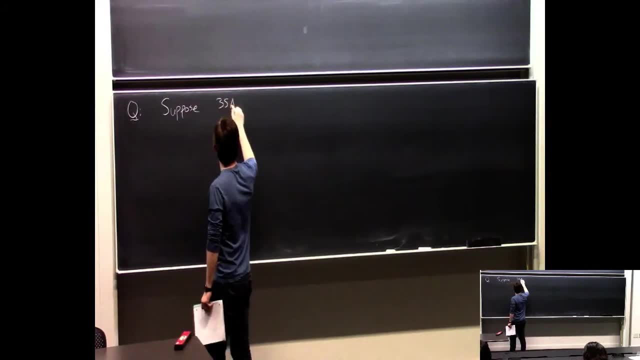 What happens if it's in polynomial time? Then the theory of NP-completeness tells us what other problems are also in polynomial time. Suppose we wake up tomorrow and somebody shows that 3SAT is actually in L. OK, It's even better. 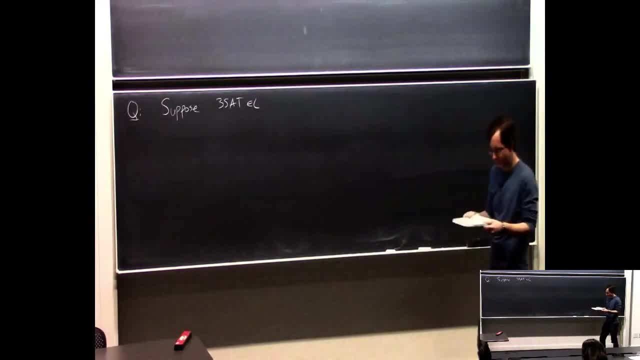 It's not just in polynomial time, It's in log space. Fantastic. So does it imply that all NP problems are contained in L? Yes, No, because what we showed was NP-completeness was in polynomial time direction. Let's see. 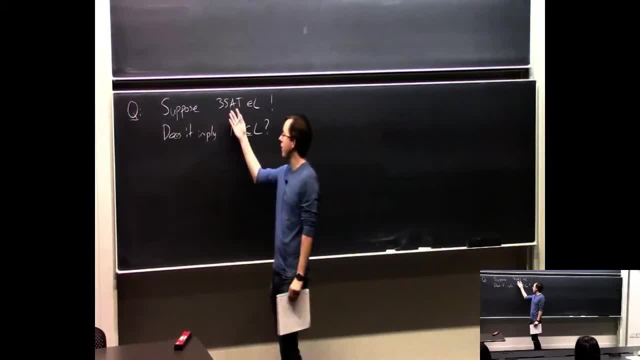 That's right. It's not clear. So you might think that well, 3SAT is NP-complete, It's supposed to be the hardest problem in NP. So if 3SAT is in L, then you might think well. 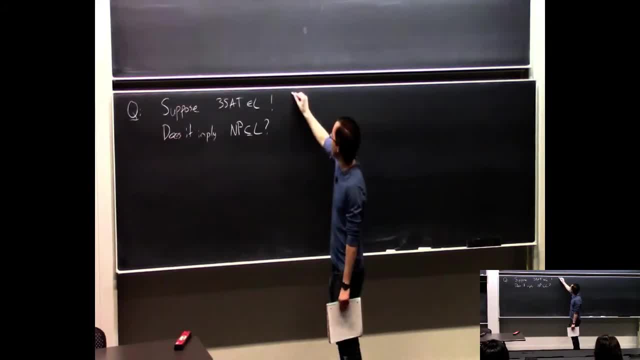 that should mean everything in NP is also in L. OK, If that's a little bit too hard to imagine, you can maybe ask the same question about NL. So you have non-determinism in both statements. But that's right. As mentioned, we don't, for example, know this yet. 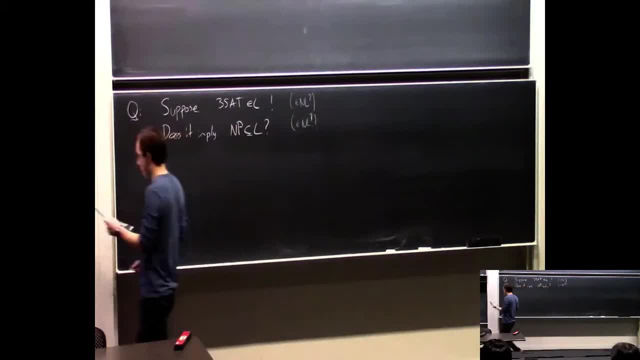 Because how do we prove this? We gave polynomial time reduction from anything in NP to 3SAT. That doesn't help us show that we faced this issue last time that a problem in NP is in L In order for that to work. 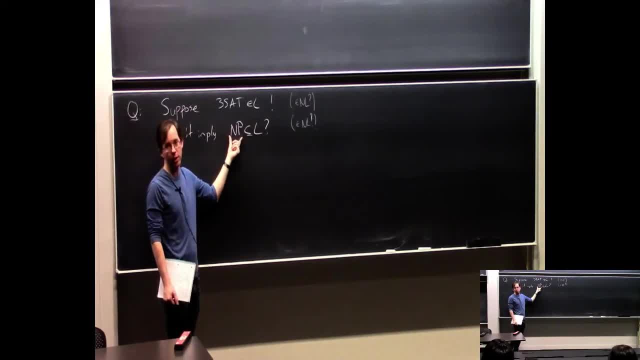 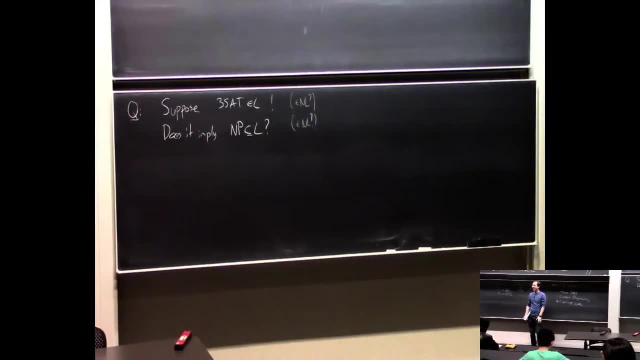 we would need to know whether there's a log space reduction from everything in NP to 3SAT. So is there? You're going to have to ask a different question. That's fine. So that means like if we're defining completeness. 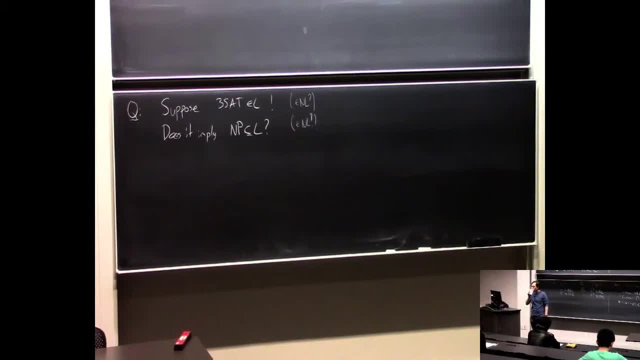 for a complexity class, we should find and expect some reduction. So P-complete is respect to P-completeness. OK, OK, OK, OK, That's right. Yeah, So technically, whenever you say something is complete for a complexity class, 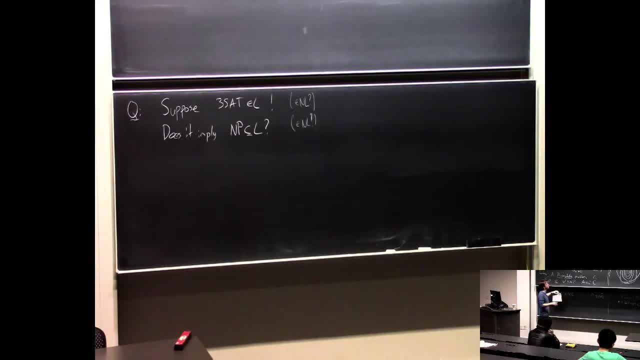 you should specify what kind of reductions you're talking about, Which I haven't always done, but technically I should. So here, for example, I specified this Right. Well, so this is a question And we actually have to ask ourselves. 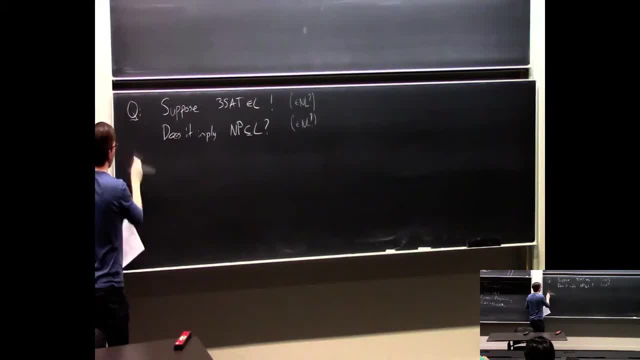 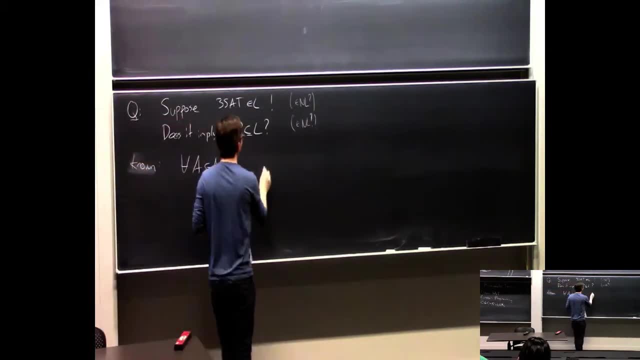 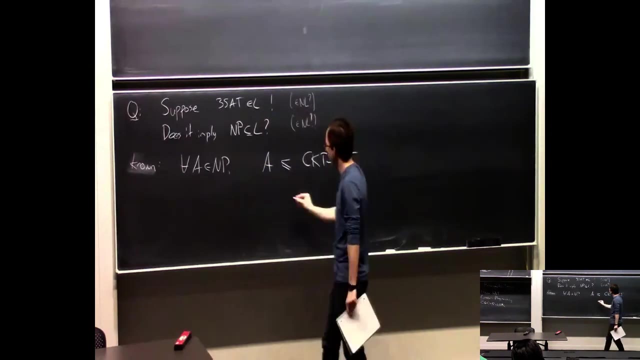 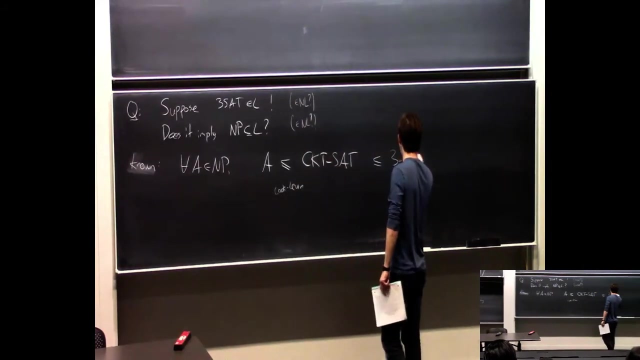 Wait, do I want to say a lemma? No, So it's known. But for all A and NP, A reduces to, in some sense, circuitSAT. That's Cook-Levin. And then we also know that circuitSAT reduces to 3SAT. 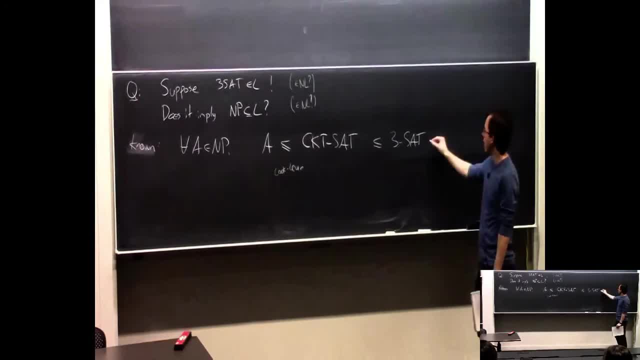 some kind of gadget reduction that we saw, And we also saw like a million other things. or you saw even in previous classes that 3SAT reduces to 3-coloring and so forth, But these were all things that we could reduce to 3SAT. 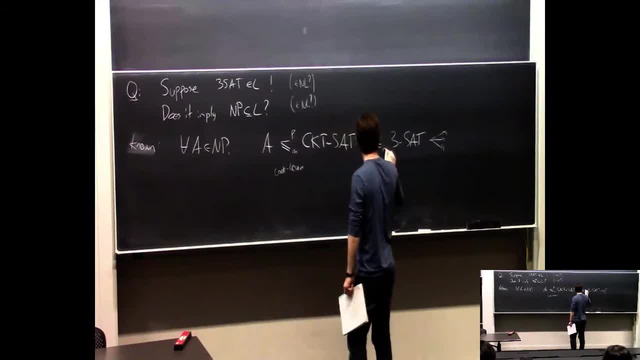 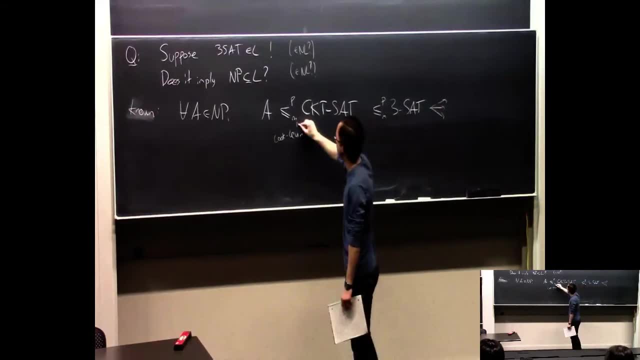 and these were all true with polynomial time reductions, And now that we are studying classes inside P, it seems worthwhile to ask ourselves, you know, is it also true with log-space reductions? And it would be good to know whether or not that's the case. 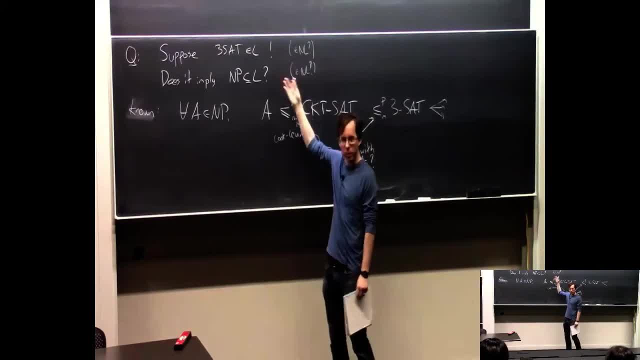 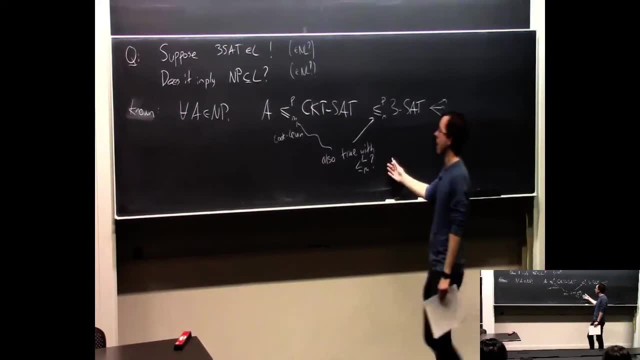 Because, if it were, then this implication would be positive. And in order to know the answer to that, you literally have to reinvestigate all the proofs of these reductions, which will do a little bit, Because, as it turns out, the following: 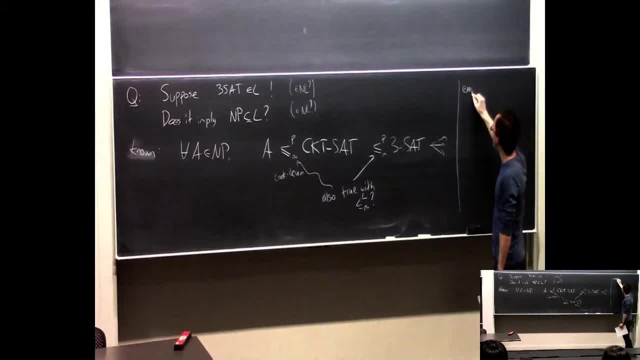 is not like a theorem, but it's like an empirical fact which I tell to you Whenever it's the case that a language A reduces in polynomial time to a language B- and you know A and B are like actual natural languages. 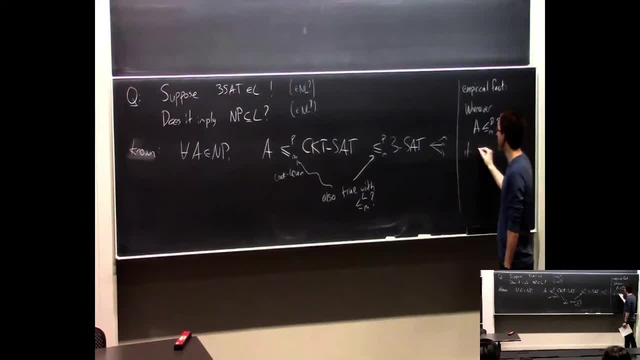 that you're interested in talking about. pretty much seems that indeed, A reduces to B in log-space as well. So it's not a theorem or anything, but it's like a fact of life that people have come to see over time. 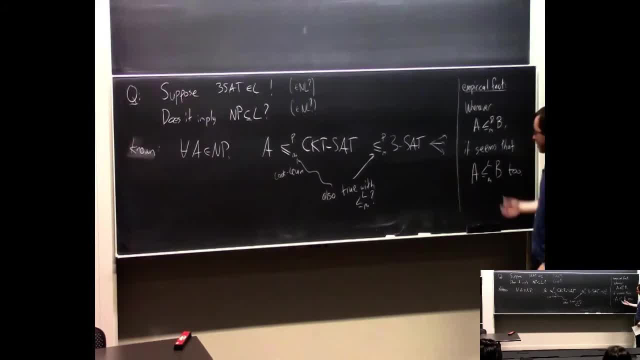 So you cannot appeal to this fact in homework or anything, but you have to, because you always have to think about whether this is true. but it can be a guiding principle for you. Yes, Is the converse true as well? Yeah, because every log-space reduction- 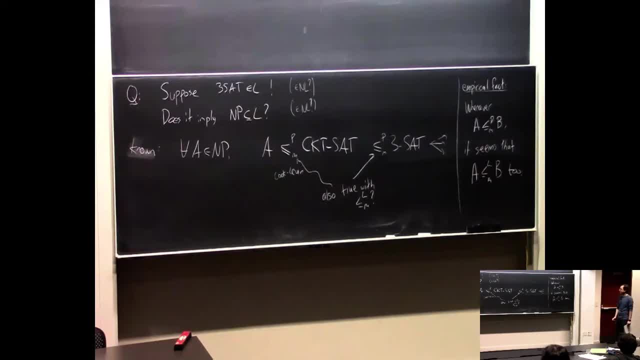 is also a polynomial time reduction. So in fact, the answer to all these questions is yes. So in fact, Cook-Levin's theorem is true with log-space reductions And circuit-set reduces to 3-set, with log-space reductions And therefore these consequences. 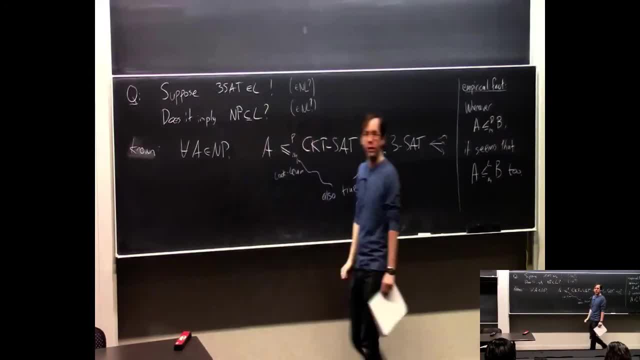 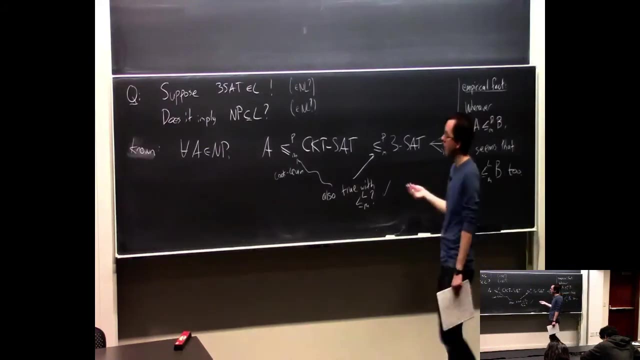 are true that if 3-set happens to be in L, then in fact everything in NP is even in L. So I'm not going to revisit every single reduction that we've proved in this course to try to convince you of this fact, but I'll revisit maybe one. 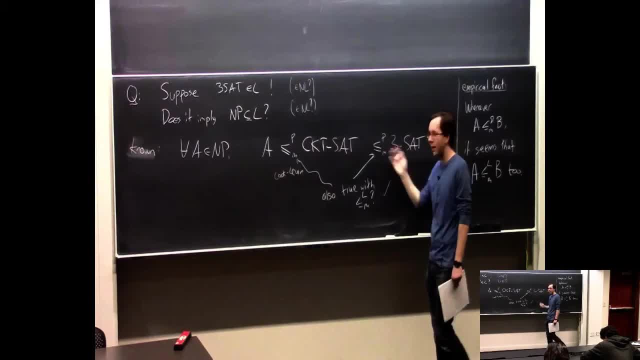 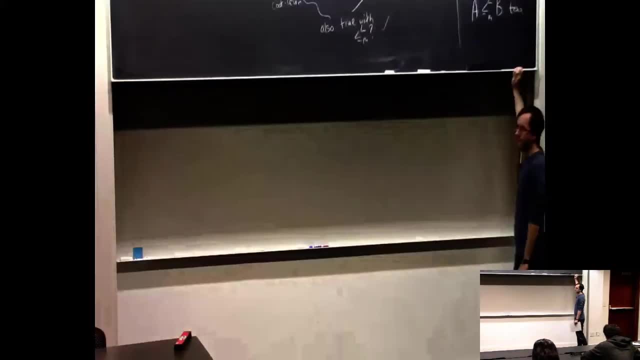 or two just to kind of get you in the mood for understanding why this is the case. OK, I hope it's a little bit motivated as well. Yeah, You're saying NP is a subset of L? like from an empirical sort of way. 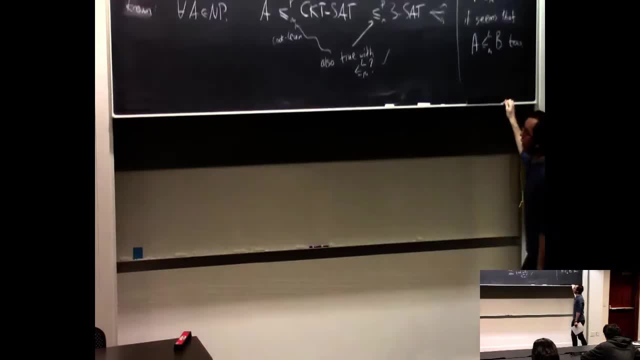 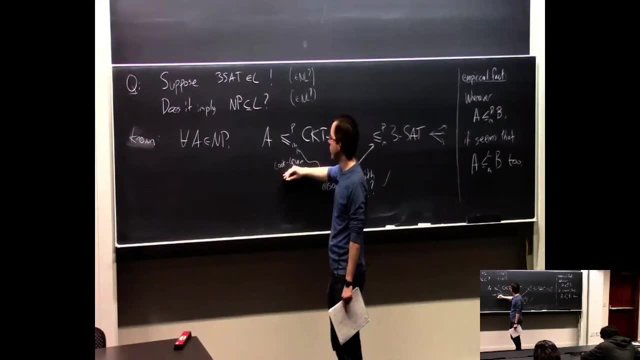 Or is he formally mentioned on that? No, OK, so this I'll state as a theorem: So Cook-Levin's theorem holds true. So this is Cook-Levin's theorem. from here this statement. And if I were to erase this and put L here: 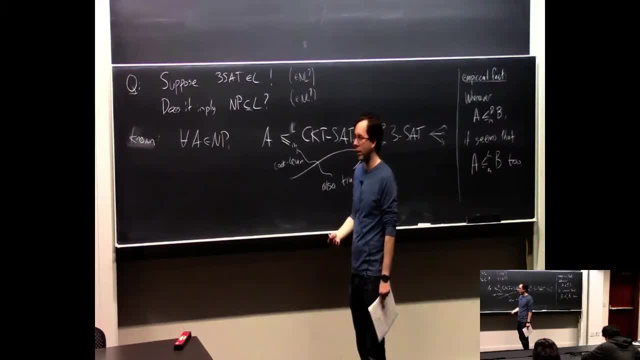 that's also a theorem, which I'll try to convince you of in 10 minutes or something. Given that that's a theorem, this is a. I didn't write it, but this is a. This is also a theorem. I mean, and this is also a theorem with L here. 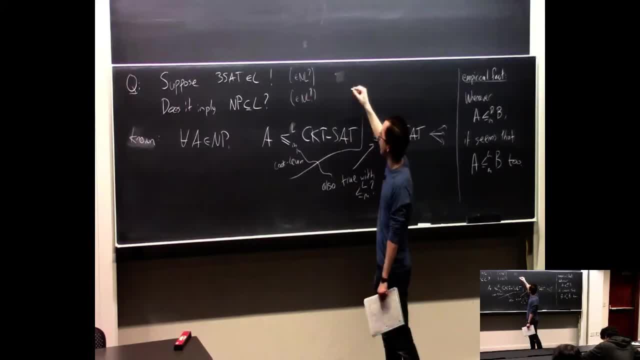 I'll convince you of that in a second. And putting them together, these theorems imply also that 3SAT in L implies NP is a subset of L. Why is that? Doesn't that depend on your empirical fact in general, Like if you have a language that you know is an NP because you 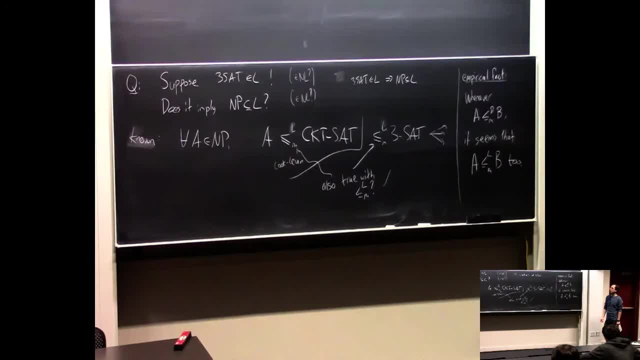 have a reduction from 3SAT, but you can't find a reduction from 3SAT. how do you know? Because this is going to be a theorem For all languages in NP: that language reduces in log space to circuit SAT. And another theorem is that we'll also show in a second. 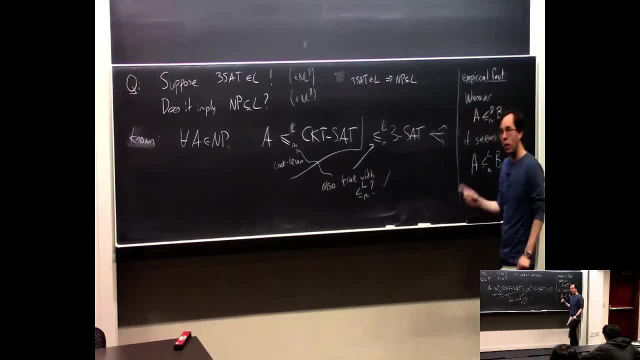 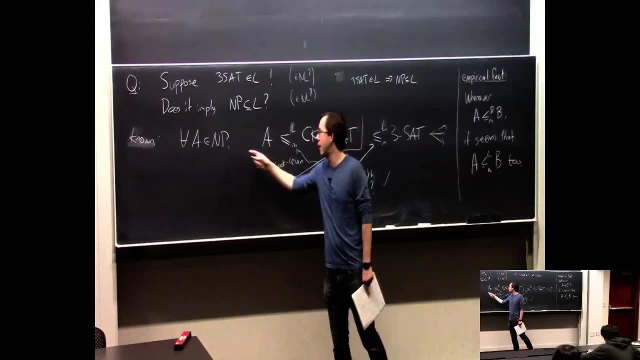 is that circuit SAT reduces in log space to 3SAT. So last time we ended on proving that these log space reductions are transitive. So we therefore get as a consequence that all languages in NP have the fact that they reduce in log space to 3SAT. 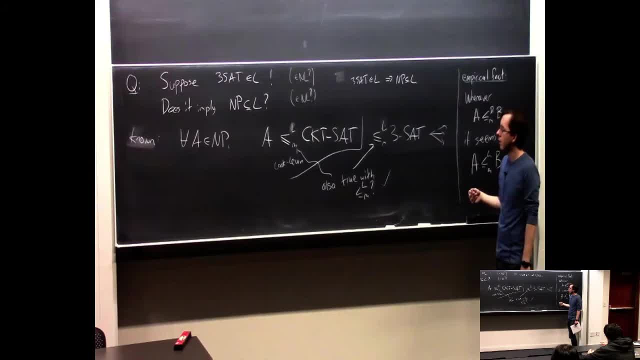 And then, Yeah, NP is closed under log space reduction. So if 3SAT is in L, then anything that reduces to 3SAT in log space is also in L. Actually, we don't need anything about NP for that L, we need that L is closed under log space reductions. 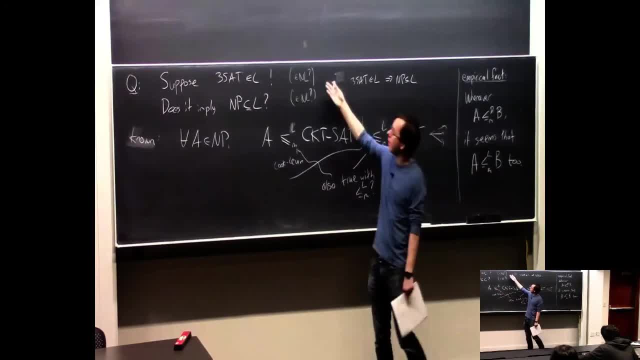 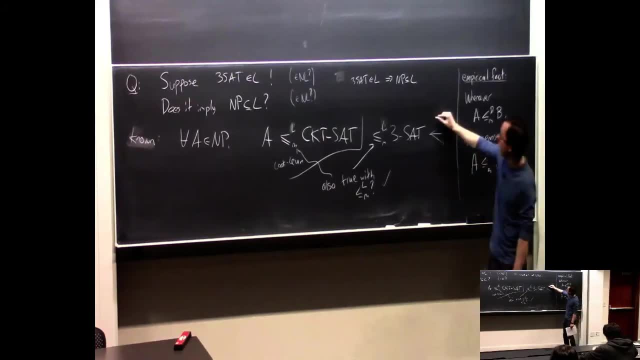 So if 3SAT is in L, then everything in NP is in L, And if 3SAT is in NL, then everything in NP is in L. I mention this because, for example, I'm not going to discuss the 1,000 reductions from 3SAT. 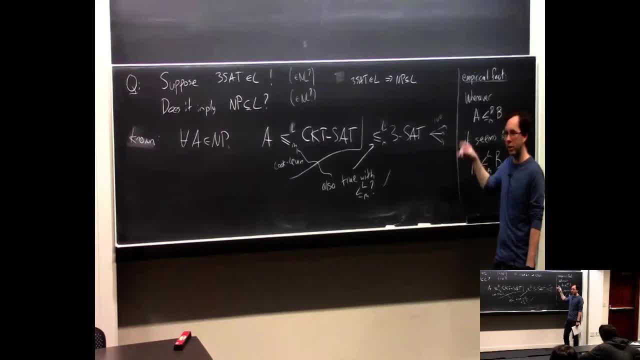 to other things Like 3 coloring and independent set and chromatic number and solving Tetris and Sudoku and everything. I mention this empirical fact to assure you that all of those problems are also NP-hard under log space reductions. 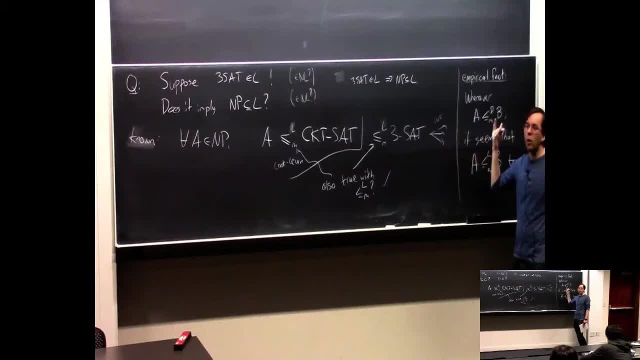 So if any of those problems, like the thousands of problems that you know or have heard, are NP-complete, if any of those problems is in L, then all of NP is in L. So that relies on checking that. all these reductions that you start seeing in 251 and so forth. 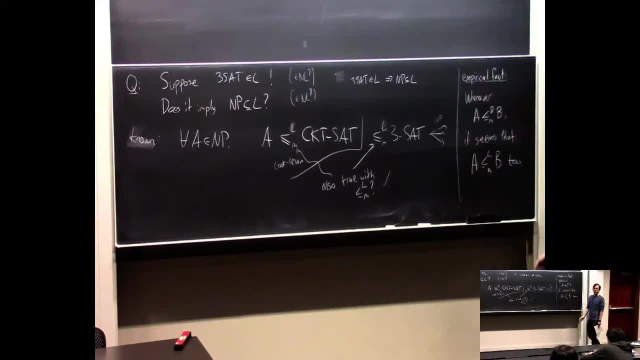 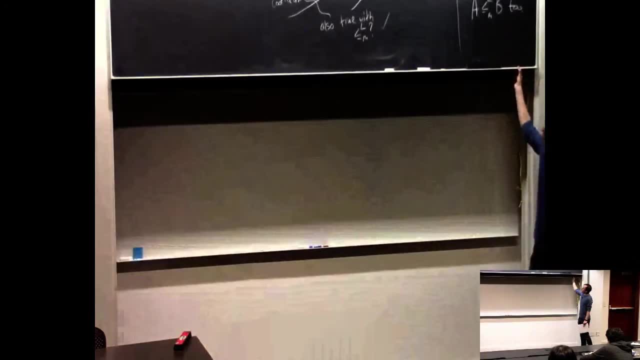 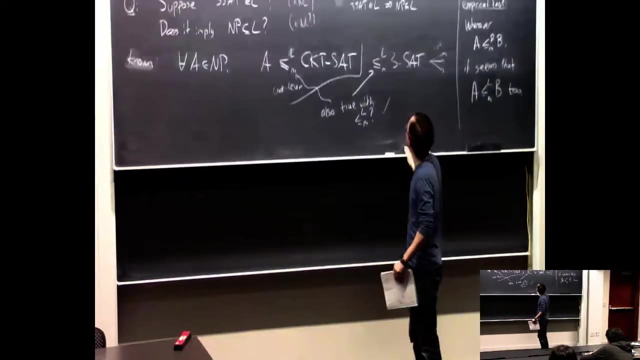 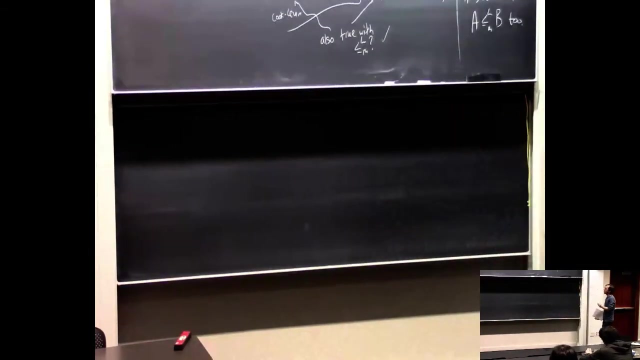 251 and so forth are not only polynomial time but also log space. OK, So let me do some example. Let me start by doing this example right here, Or not even doing it, but I'll show it to you. So recall that when we first defined reductions, 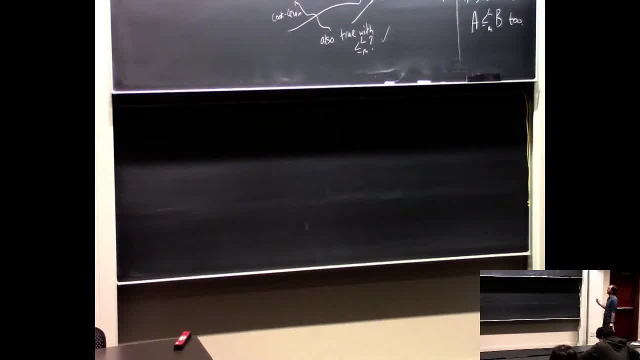 in fact, the first one that we looked at, or maybe the second one we looked at, was that circuit SAT reduces to three SAT in polynomial time, And now I'll show you that it also reduces to it in log space, which is a stronger statement. 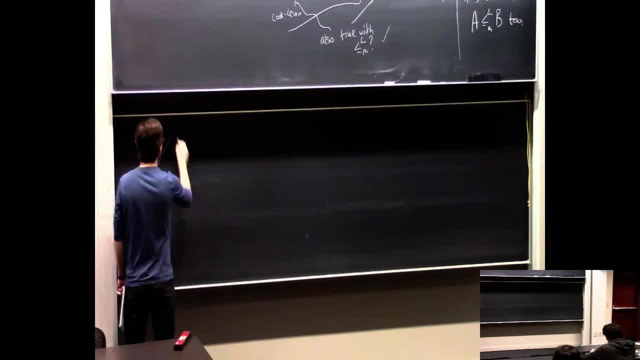 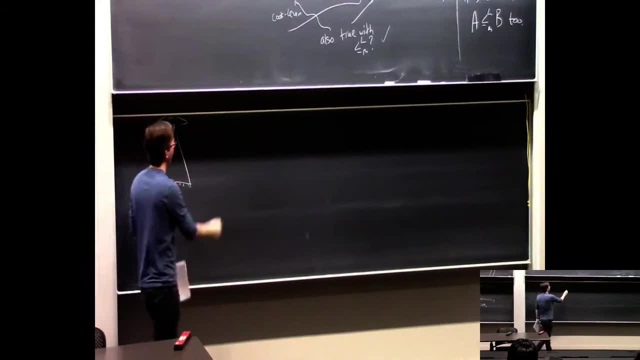 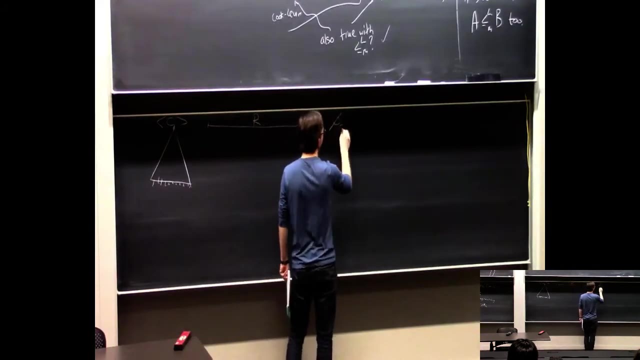 OK, So let's remember how that reduction works. You know, you're given a circuit, C, one output and n inputs, And you had a polynomial time reduction that took the description of the circuit and output, the description of a 3-CNF formula. 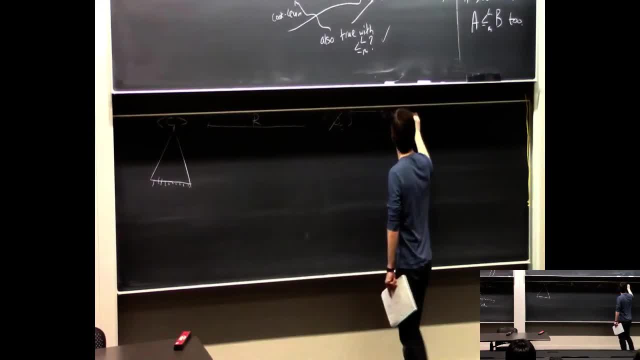 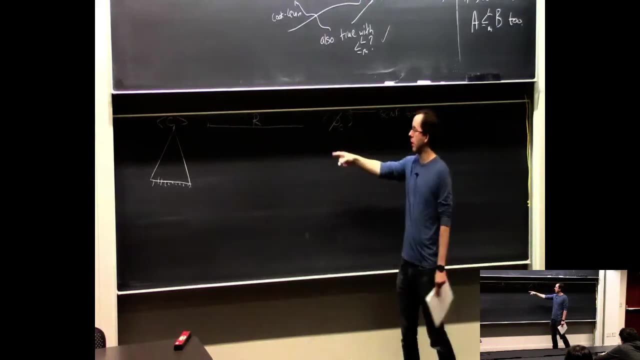 This is a 3-CNF formula And one thing we proved about the reduction. well, we proved two things about the reduction. First of all, it's polynomial time And second of all, we proved that C is satisfiable if, and only if, this 3-CNF formula is satisfiable. 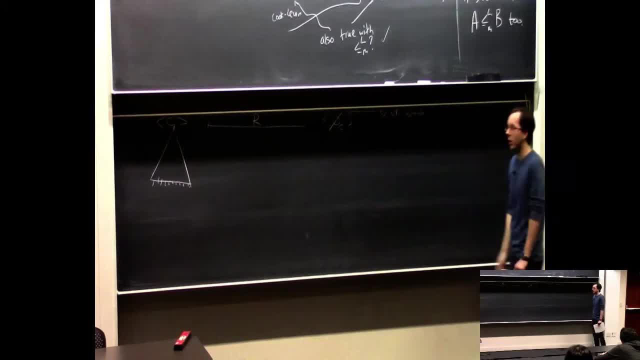 And that gives us a polynomial time reduction from circuit SAT to 3-SAT. And we're going to use the exact same reduction. We're just going to observe that not only can be computed in polynomial time, but it can be computed in log space. 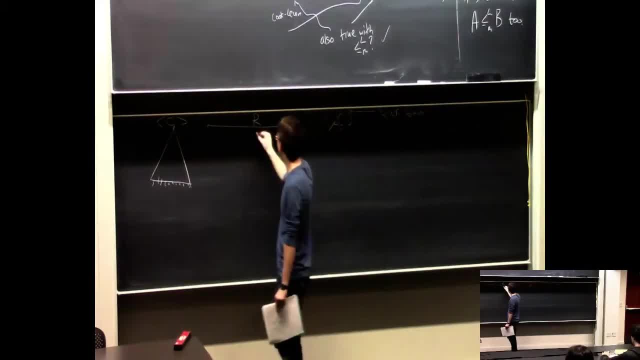 OK, So we'll show that this is also computable in log space. Well, show might be a strong word, but I'll sketch it for you because after a little while you'll see it's not overly interesting, Right? So what was the idea of this reduction, if you recall? 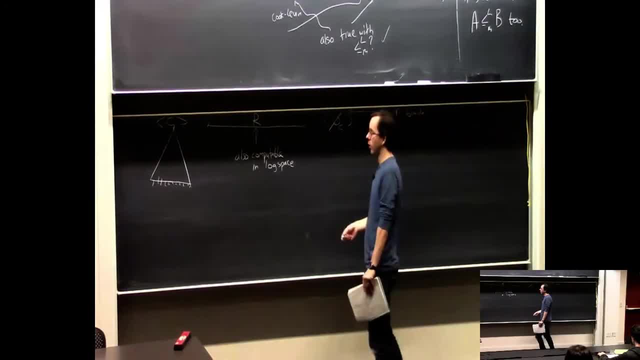 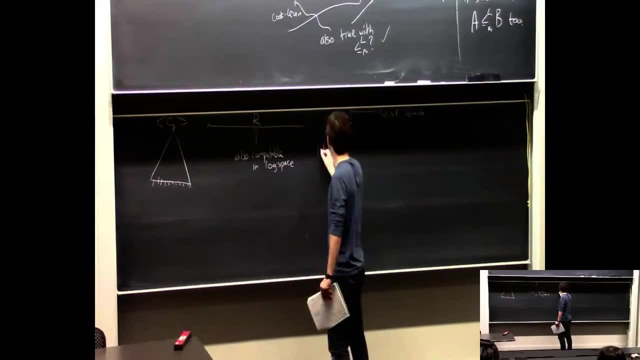 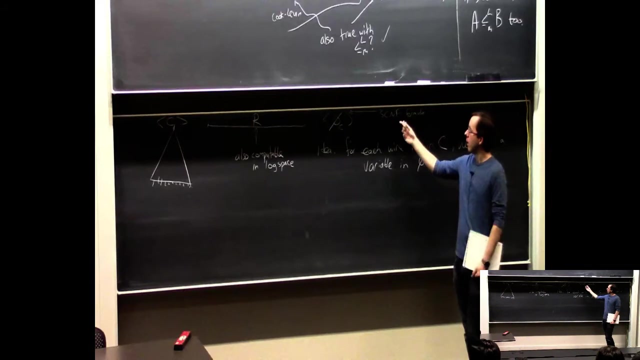 The idea is, for each wire here we're going to have a 3-CNF- OK. In C we're going to have a variable in phi C- OK, And basically what we need to do when constructing this formula is put in some clauses of length and length. 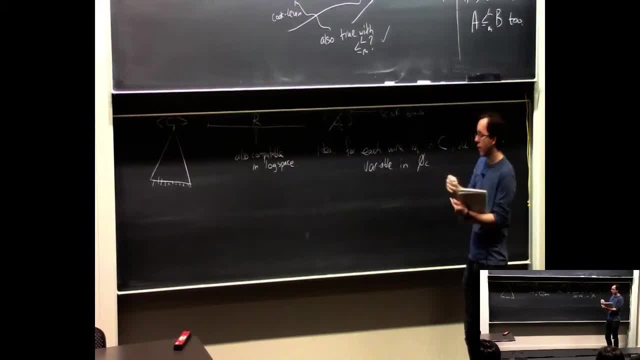 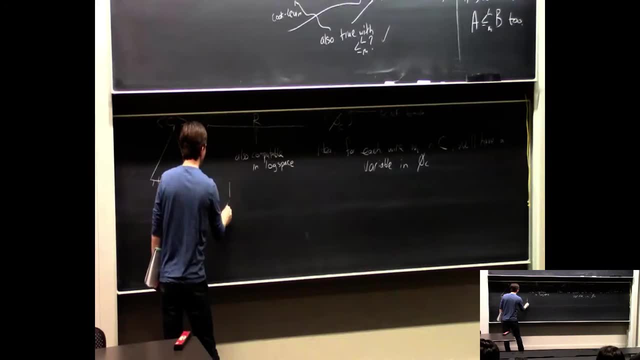 OK. So we're going to have some clauses of length 3 that say all of the wire variables are what they're supposed to be. So for example, if over here you have an AND gate inside C and this wire is wi and this wire is wj and this wire is wk, 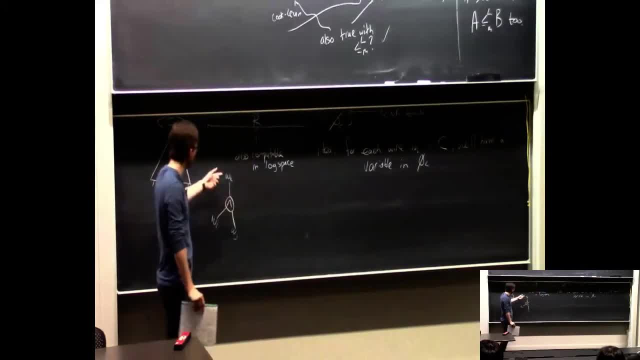 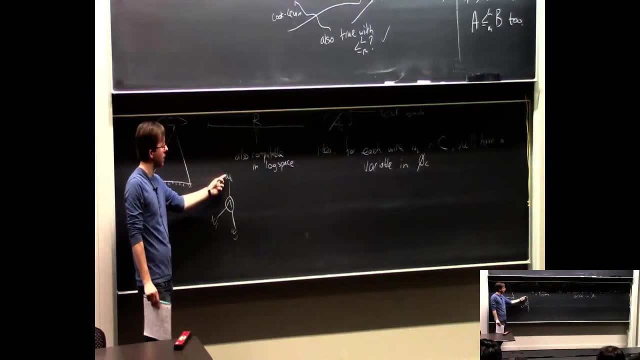 you need to put some 3-CNF clauses into phi C that sort of specify that. indeed, however, wi and wj are set, if you're going to satisfy phi C, you have to set wk to be the AND of wi and wj. 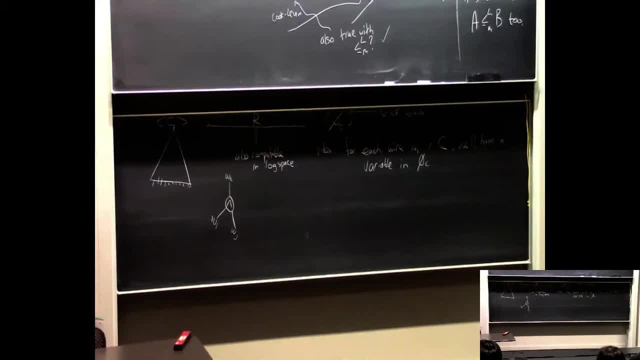 And you have to do this also for the NOT gates and the OR gates. And then the input wires just stay free in the circuit And you also put in one extra clause at the end that just contains the output wire, OK, And then phi C is. phi C is satisfiable. 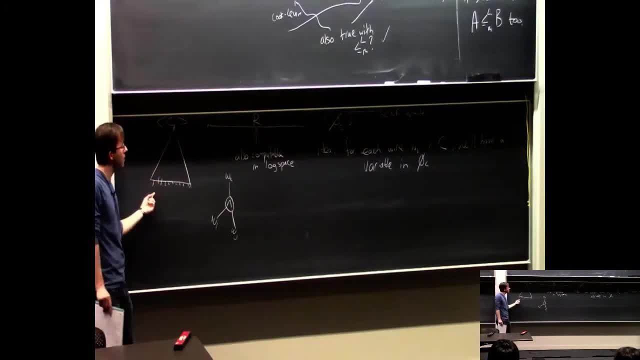 In order to satisfy phi C, you have to find some setting for the input wires And that forces all the settings for the internal wires if you're going to satisfy it, because we put in clauses that enforce these relationships And you have to satisfy the output wire. 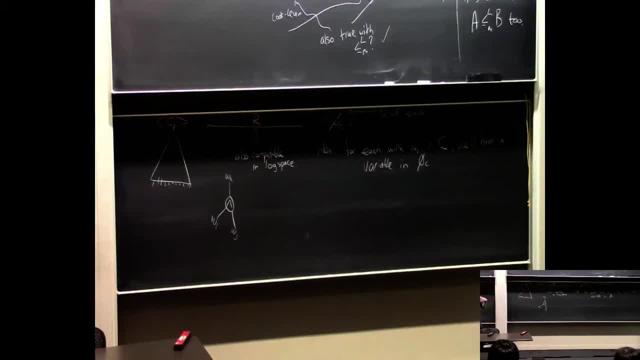 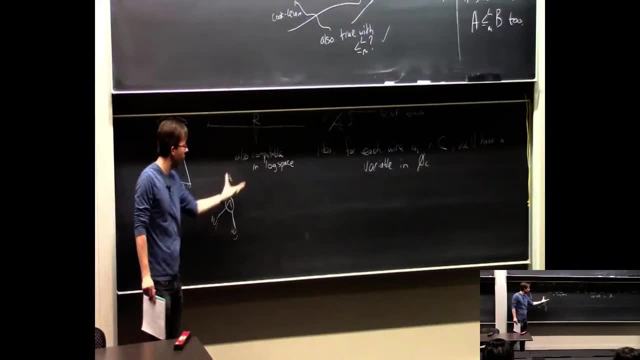 which is also in the 3-CNF. OK, So hopefully you kind of remember all that from when we talked about reductions. But the main part was of what the reduction had to do was it had to go through each basically gate in this circuit. 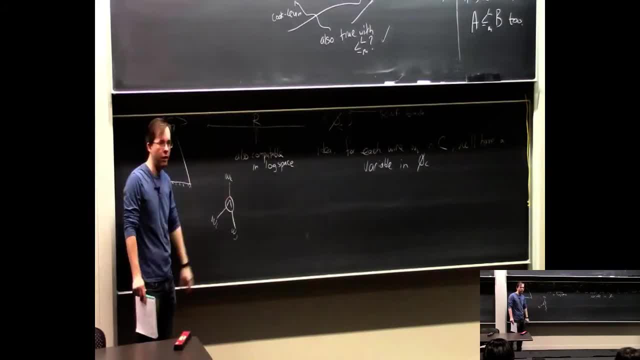 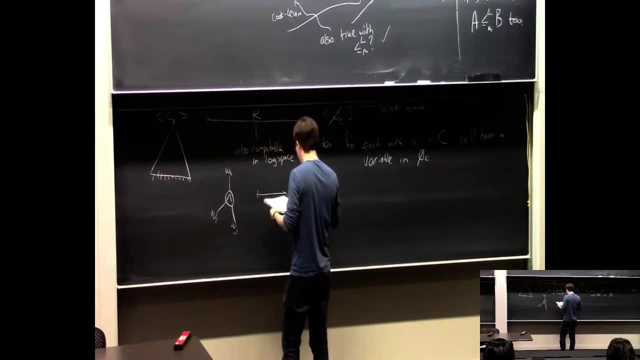 and put in some clauses in the formula based on the gates, So like I'll write it down, For this specific gate we explicitly put in like WK, NOT or WI. That was one clause: WK, NOT or WJ. 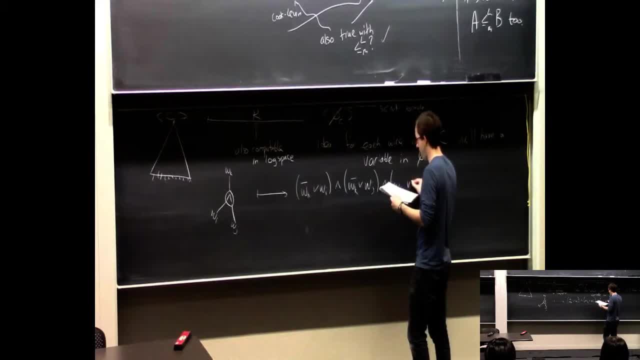 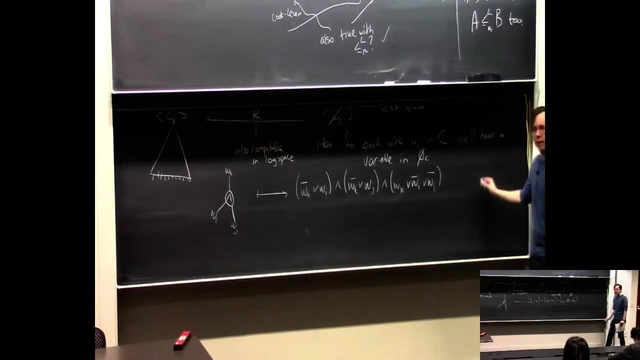 That was another clause. WK or WI or WJ, NOT, That was another clause. OK, And there's like a similar one for OR and a simpler one for NOT gates- OK, And then you also stuck in the output wire at the end. 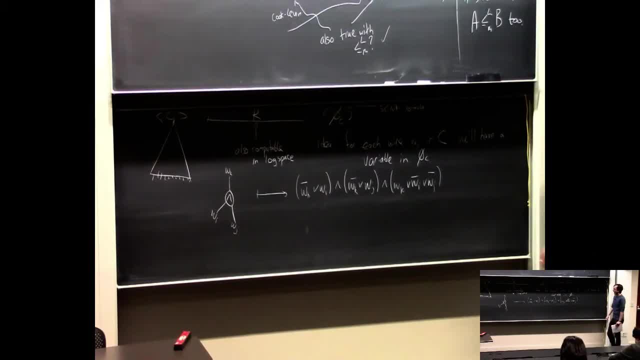 So that's the reduction R And we probably at the time just said: well, it's pretty simple, Like you can do that in polynomial time. Now we have to look at it a little bit to make sure that you can do it in log space. 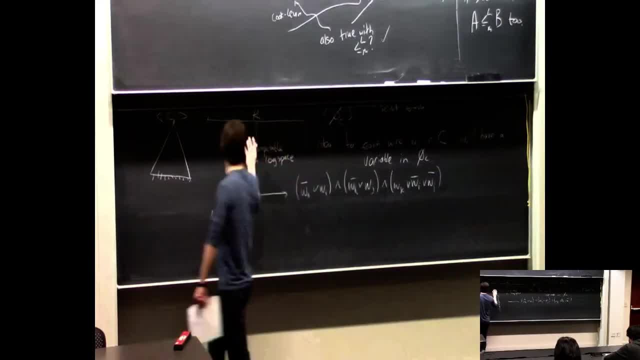 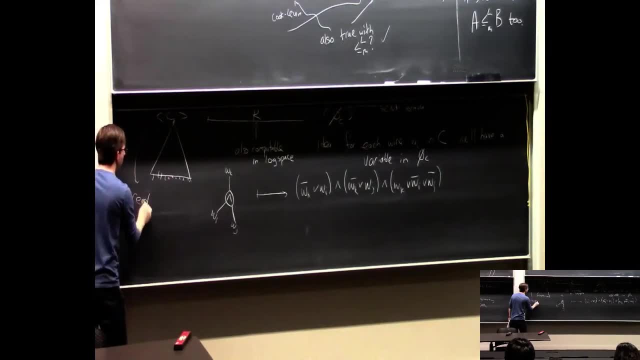 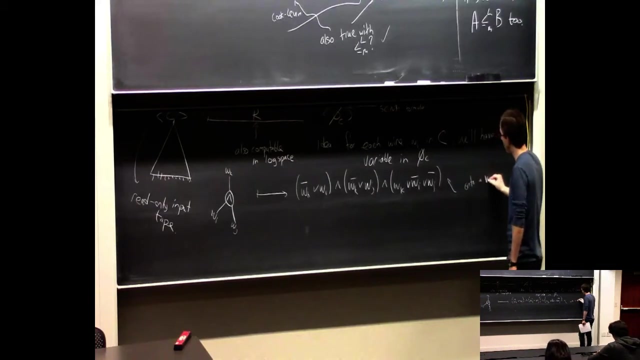 And we even have to remember the model. So what is the model for algorithms with input and output in log space? We have that this circuit diagram is sitting on a read-only input tape And the algorithm has to write this final phi, c. This has to get onto a write-once output tape. 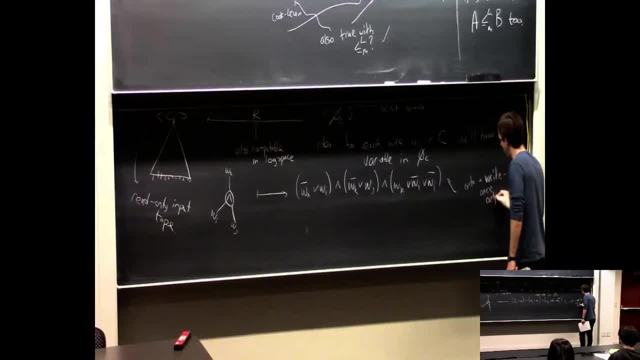 OK, And the algorithm is allowed to have order log n. Well, order log the size of the description of c bits of working circuit. OK, And then we have to write down the name of the variable. OK, And then we have to write down the name of the variable. 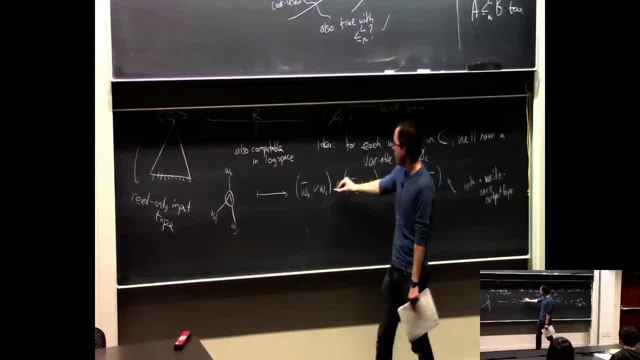 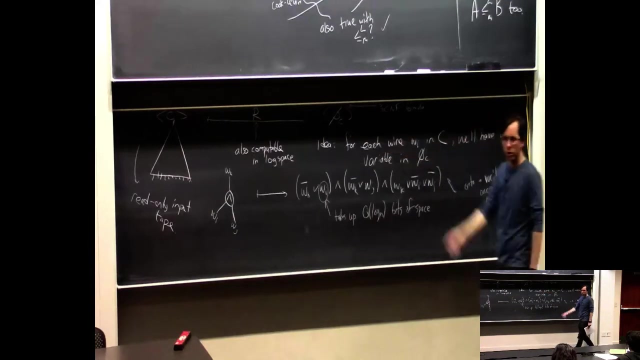 OK. And then we just also observe here that, like writing down the name of one variable, it basically involves writing down the index. So like this takes up: well, basically order, log the number of variables, bits of space, OK, And then we have to log the size of the input. 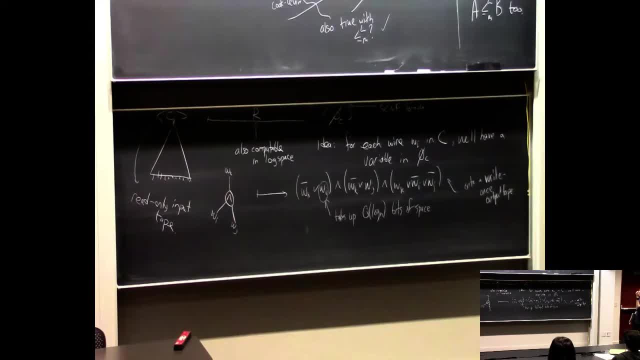 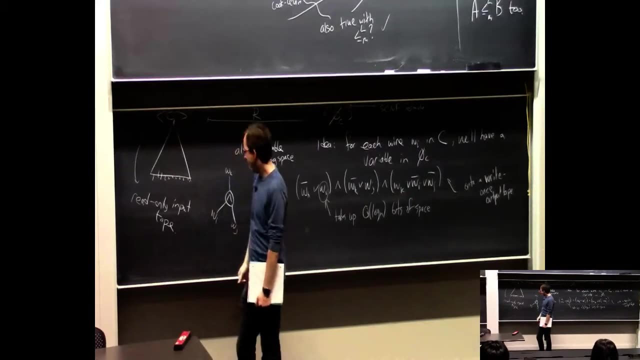 There are no more variables than bits in the input. OK, So you see this task that R has to do. it has to basically go through every. it's very methodical and pretty simple. It goes through every circuit in the sorry, every gate in the input circuit. 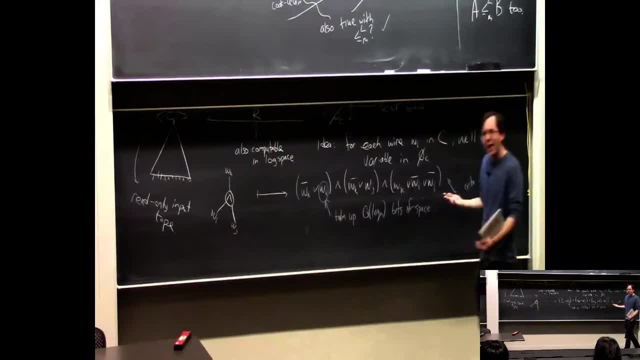 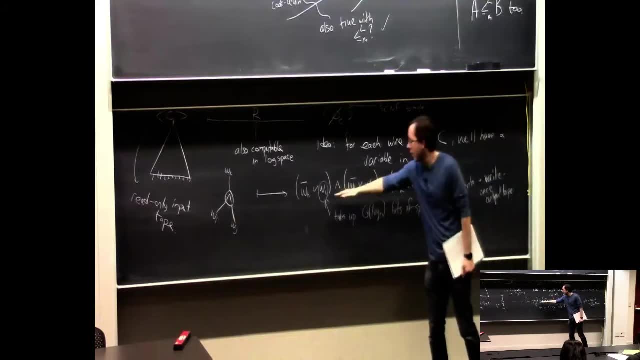 And it has to for each gate, like spit out, basically a gadget, you know, like a small constant size, you know. piece of the final answer. Now, constant in the sense that it has a constant number of variables, but actually each of these to write down. 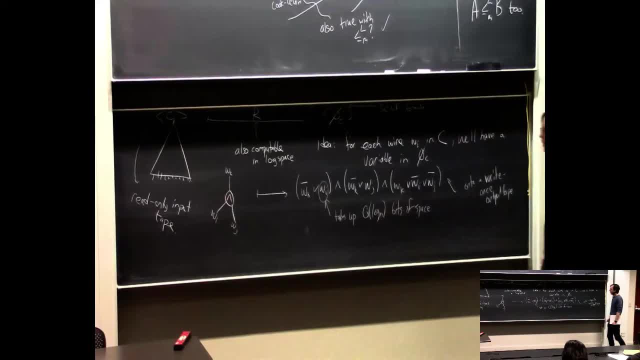 takes up log n bits. But at this point I just want to say basically that you can do it in log space, right? I mean, if you think about, we don't want to get like into too much detail, but OK, the machine is going to have to. 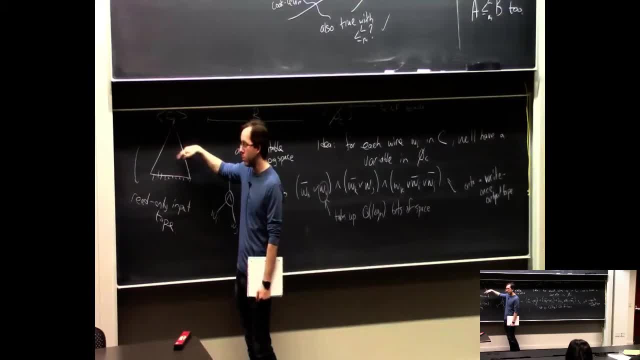 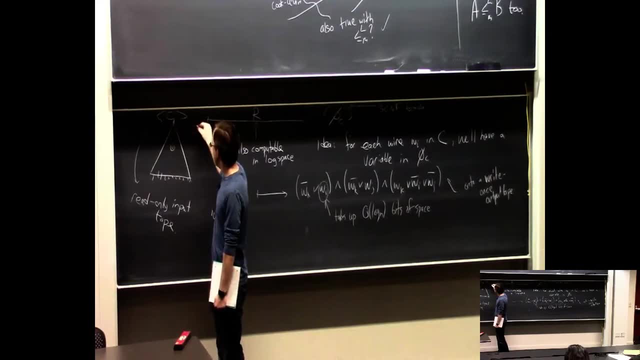 yeah, like maybe walk around the input tape a lot. You know if it's on some gate up here, you know it probably has some work tape that has the index of what's. you know what the input is. It has the index of what you know. 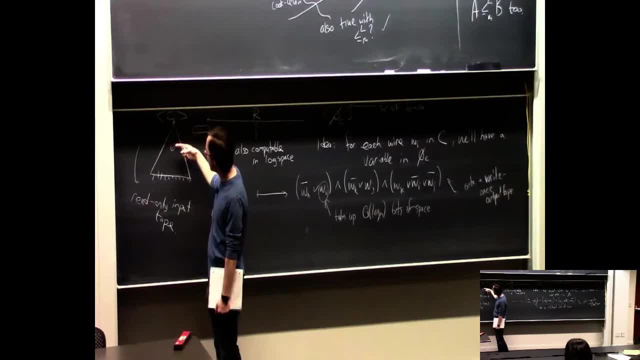 number gate this is, And now it's working on this gate. It has to look into the input to see the number of where this gate's inputs are coming from- some previous gates and so forth. So it has to understand, like you know. 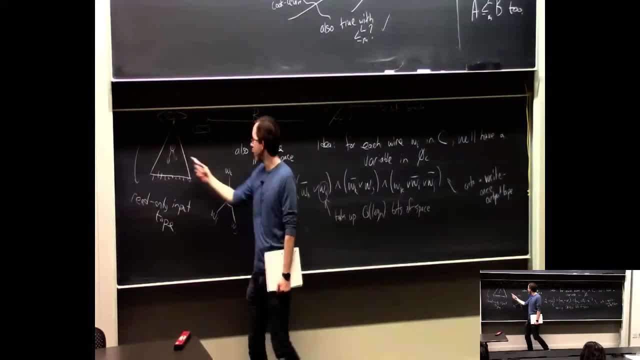 the situation for each gate, where its inputs are, And then it has to output this sort of 3CNF gadgetry for that gate. But you know, this is like some log n bits of sort of look up into the inputs and figure out what to write. 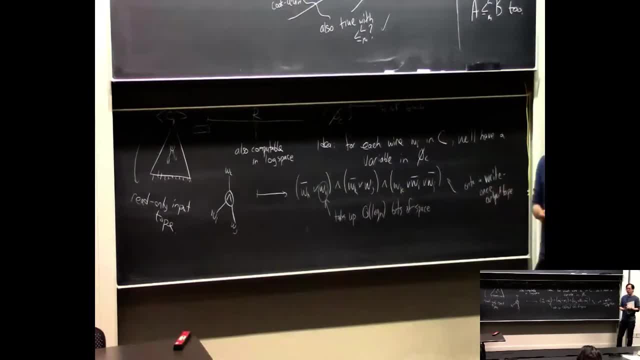 And then it has to write this, which it has to do in a write once fashion. But that's OK. You know it prepares this on a work tape, let's say, which is only order, log n bits. And then it says: all right, I'm going to irrevocably. 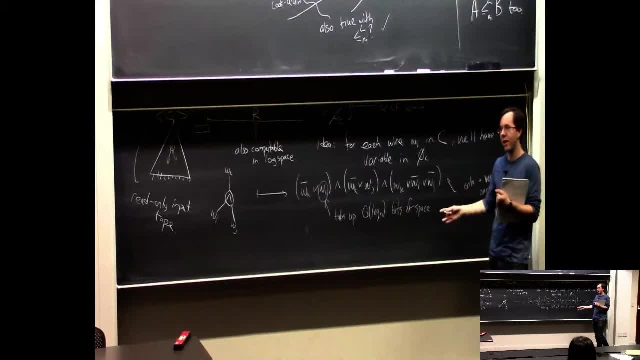 write this onto the you know output tape And you know it does that And you know it just goes until it's done. It doesn't ever have to, let's say, read back at what it looked at. 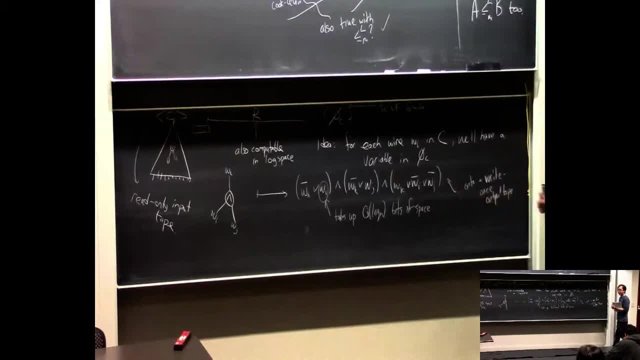 go back and look at what it wrote on the output tape, for example. So this is the. I mean any questions about this. You know this is the kind of stuff that you have to do when you're verifying, like the 1,000,. you know reductions. 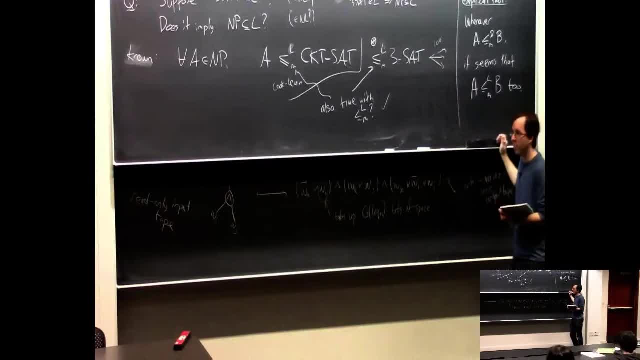 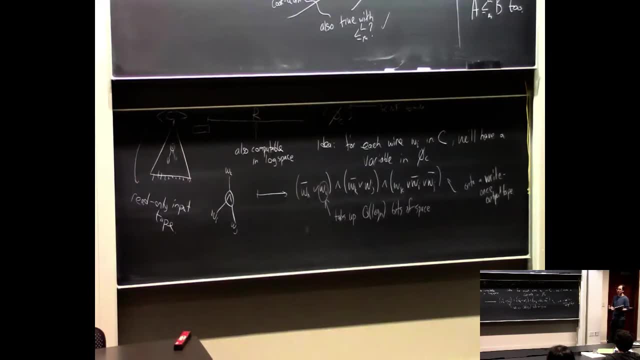 from 3SAT to 3-coloring or to independent set or what have you. You just have to look back at how they work and sort of verify for yourself that indeed you can do them in log space And it pretty much always works. 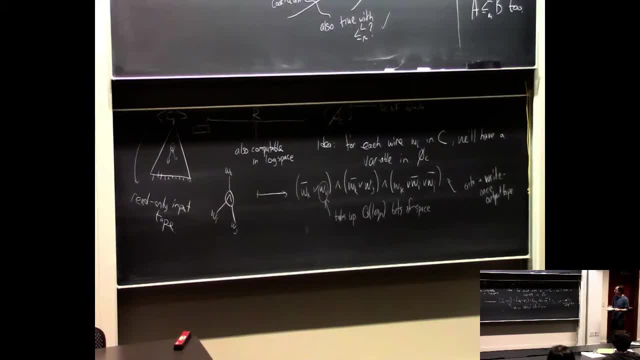 And let me say just even a little bit more why you might expect it sort of is always going to work. It's always doable in log space Like think about a reduction, a classic textbook, 251 reduction from 3SAT to 3-coloring. 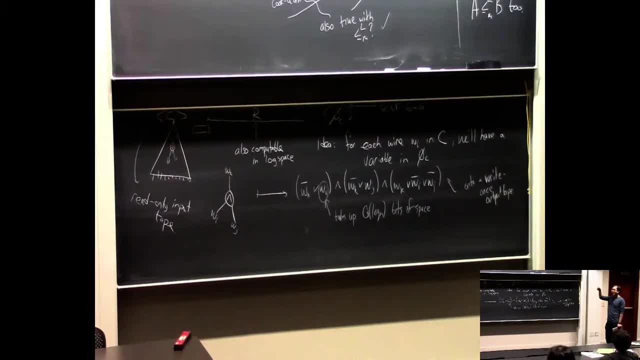 How does it work? You know, maybe you draw like a. you have to take a 3SAT formula and output like a graph which is 3-colorable if, and only if, the 3SAT formula is satisfiable. So maybe you like start by like. 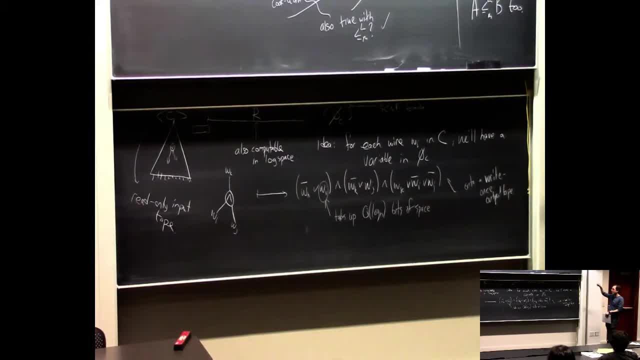 writing down a graph with a triangle in it and maybe you know that's going to. one of the vertices is going to represent true and one's going to represent false and one of them is: you know, doesn't represent anything. So okay, you can do that first part in log space. 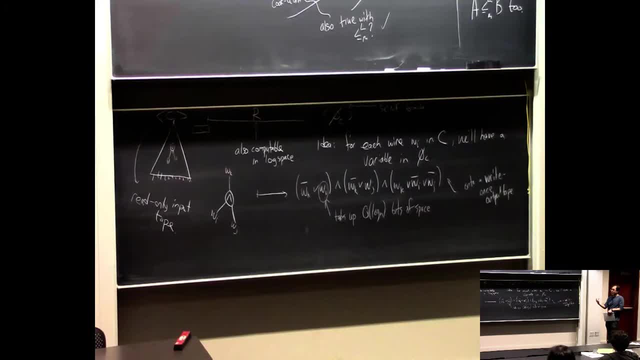 But the main part of the reduction is always like you go through each of the clauses in the 3SAT formula, which is like the or of three literals, you know, x, i or x, j, bar or x, k, And then, like, you put in some like. 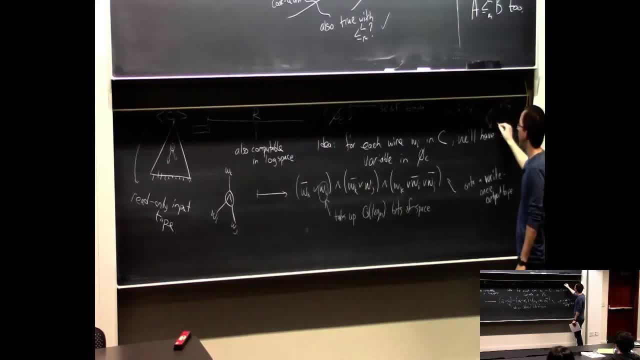 weird gadget graph with, like you know, 12 vertices and they're connected in some way and there's like a vertex for each x i or maybe there's a triangle for each x i And you know, you put in some. 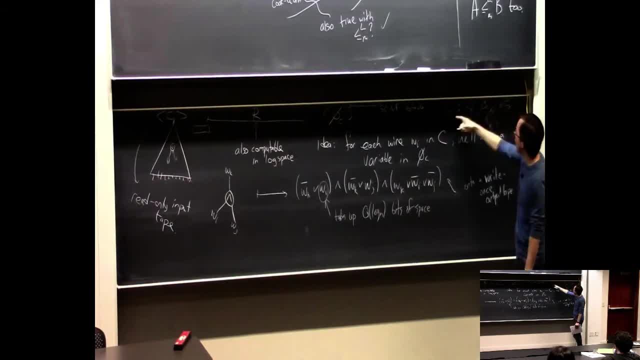 constant size graph that like connects up the vertices for i and the vertices for j and the vertices for k and maybe some of the base vertices or something. Okay, so this is my picture of a 3SAT: the three coloring reduction. 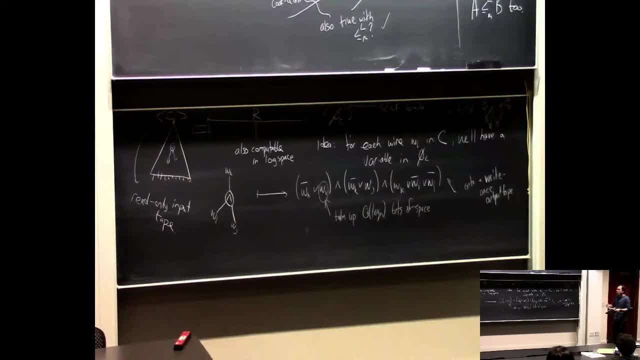 But the main point is: I mean, if you remember these things, you basically go through the inputs you know, look at what you know variables or pieces are connected to what- and you output like a constant size gadget for each piece of the input. 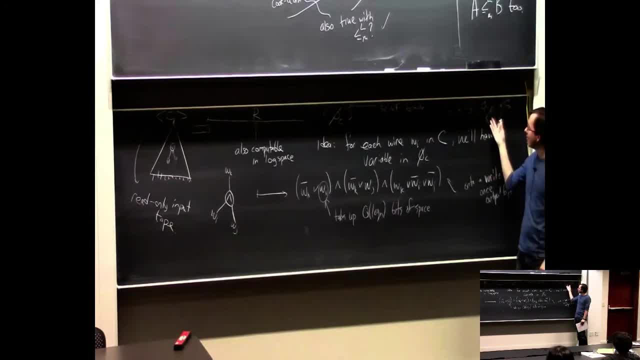 And that gadget will involve constantly many- I don't know- variable names or vertex names, each of which is like the order log n bits. Okay, so basically, since most gadgets kind of work this way, they go through the input and like 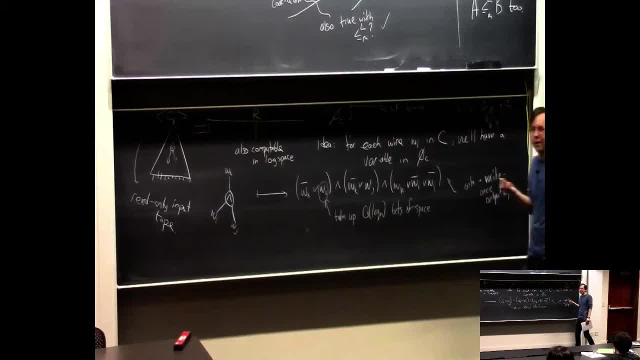 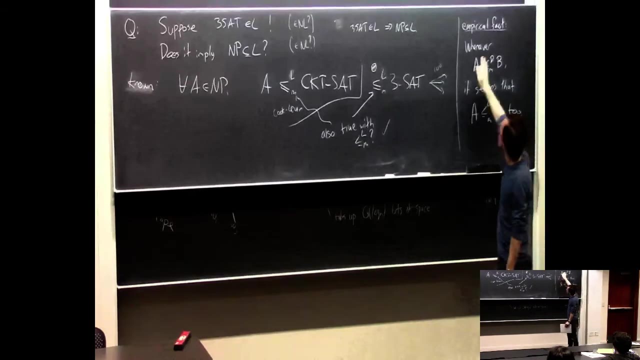 create a little gadget for each piece of the input. That's sort of why all these reductions, or these textbook reductions, are even doable in log space. Okay, so this is like a little bit boring, but that's life. So you know this empirical fact. 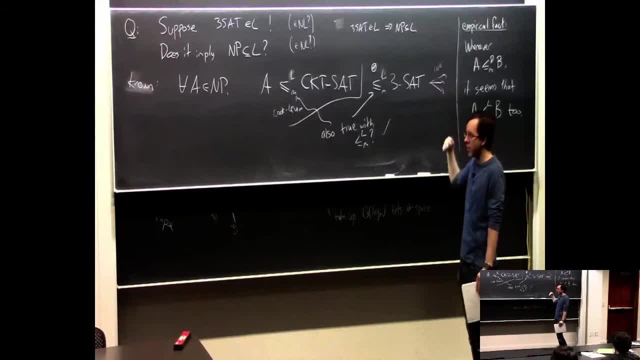 is maybe about convincing you to not worry that all the textbook reductions you know in polynomial time. they're also log space, This one we talked about in a bit more explicit detail just for fun, And now I'm going to show you details about this one too. 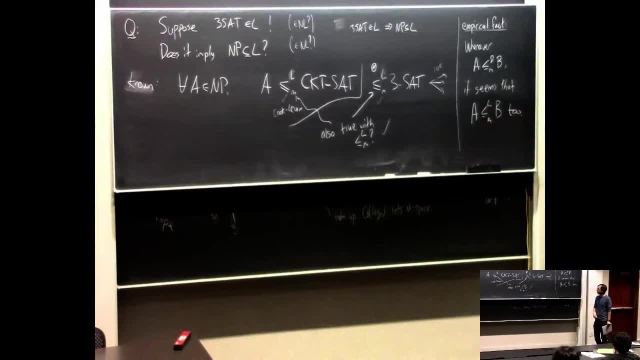 Because this one maybe is a little bit different from all the other kind of textbook reductions. You know, this is the Cook-Levin theorem. You take, like any language at all, in NP and show that it can be reduced in log space to circuit set. 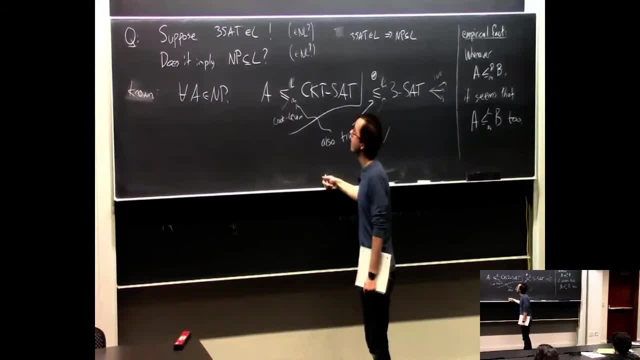 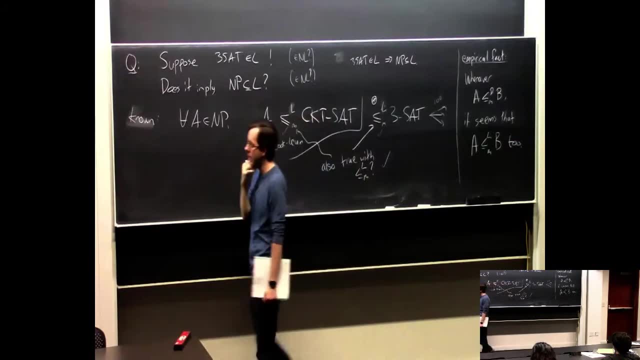 And, you know, one reason I'm actually going to focus on it is well, as a consequence, we'll get these kinds of conclusions that if 3SAT is in L, then NP is also contained in L, But the proof is basically going to prove this theorem. 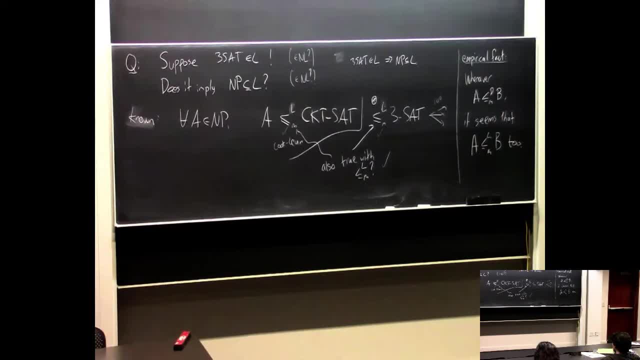 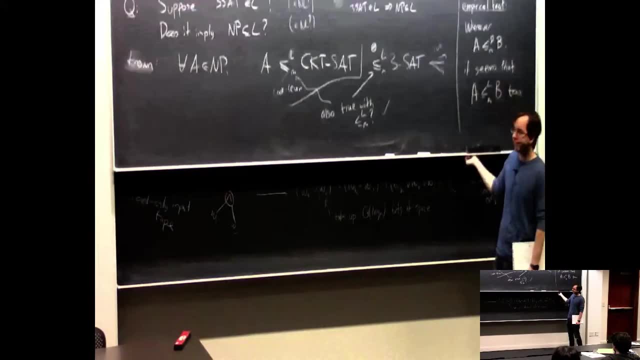 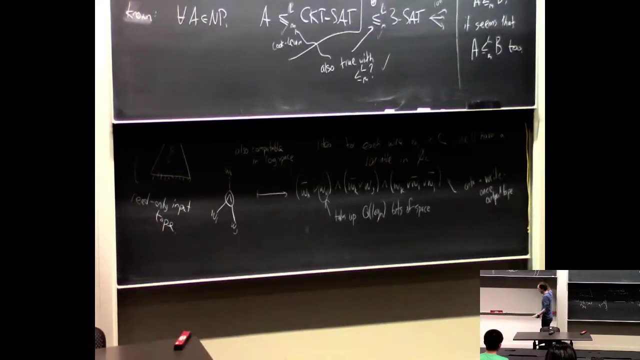 which I do quite care about that. the circuit evaluation problem is complete for P, Okay. so that's why I actually want to get into some detail about this Cook-Levin theorem, Okay, So uh, well, here's a theorem. 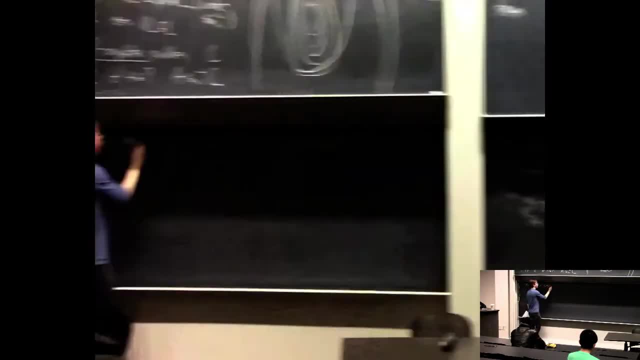 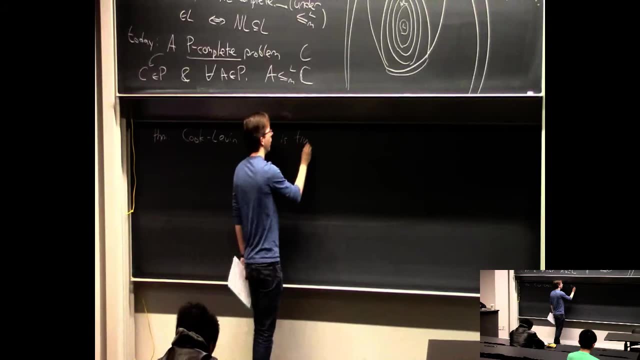 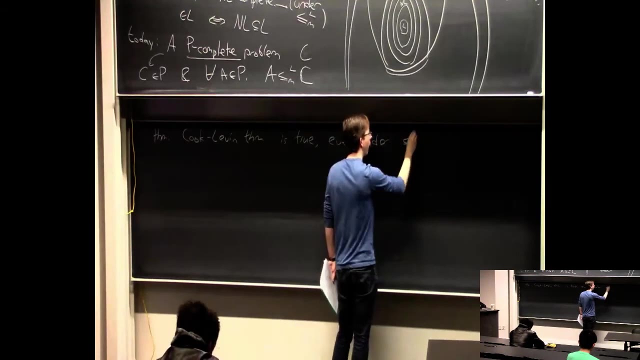 Cook-Levin theorem is true. That we proved. well, you proved a few lectures ago. But I'll add, even under log space reductions. and you know I'm not going to prove all the details, but I'll sketch it to you. 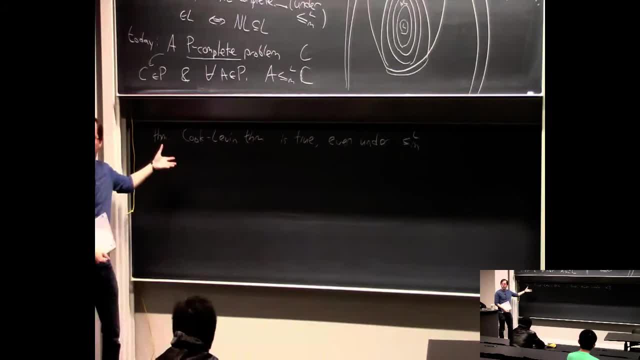 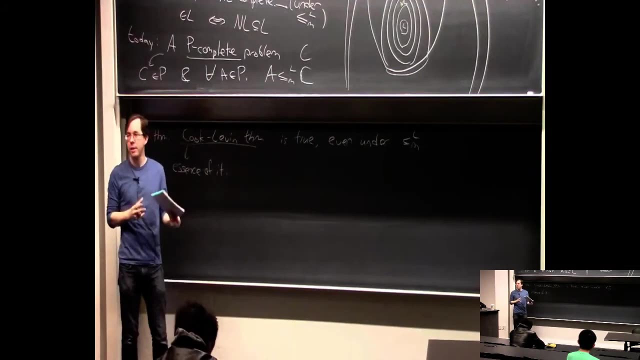 And let's you know, remember why. how does the Cook-Levin theorem work? Like? why is it true, If you remember, like 99% of the essence of the Cook-Levin theorem was the fact that polynomial time Turing machines. 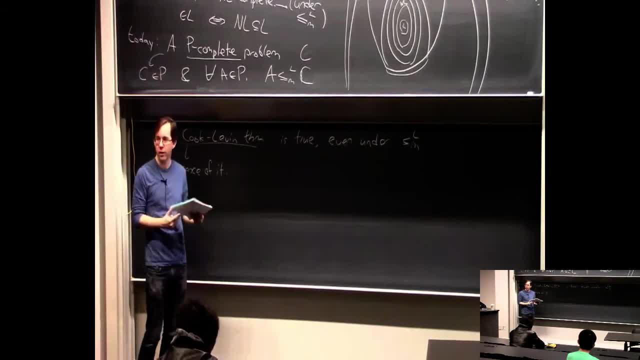 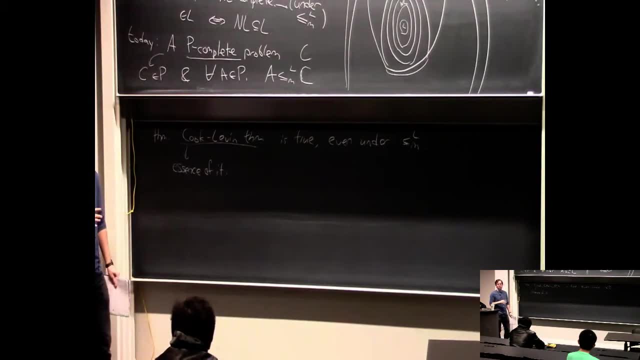 can be simulated by polynomial size circuits. That was the essence of it, In fact, if we we said that if you have a Turing machine, just a regular deterministic Turing machine that runs in time T, then you can build a circuit that simulates it. 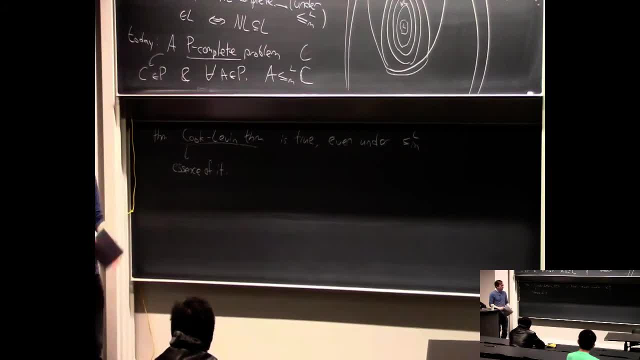 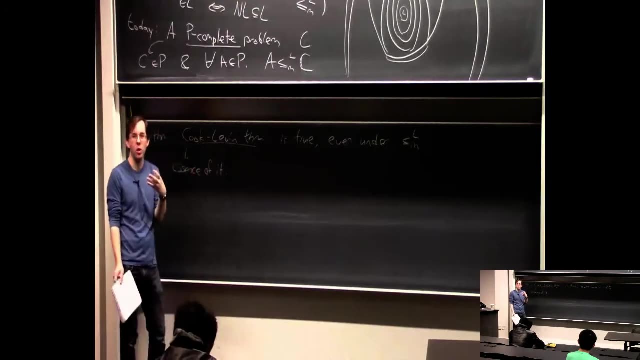 in size T squared, And that was like 95% of the proof of the Cook-Levin theorem. And in order to you know, verify this theorem, you actually had to show that the process for a fixed time, T Turing machine, the process of 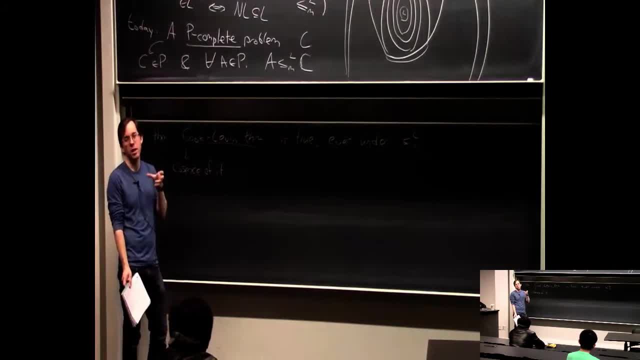 taking an input string, x, and building the circuit that simulated m on x. that process itself had to be doable in polynomial time And similarly, like we just sketched that process mathematically and we said, ah, it's pretty easy. 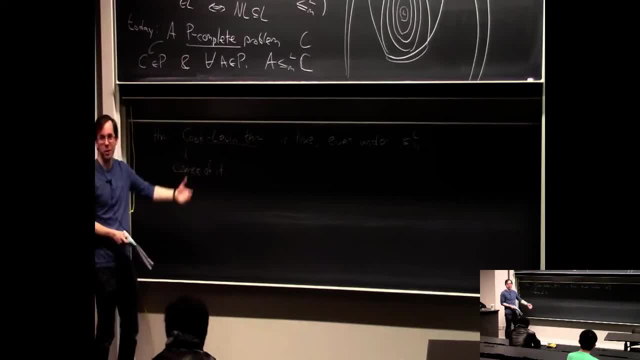 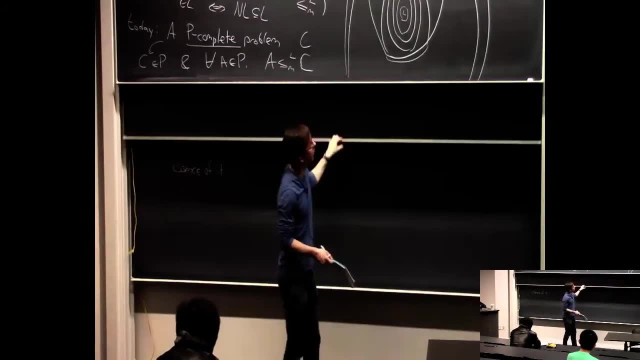 it's pretty clear that you can do it in polynomial time. You're also going to be able to do it in log space, And that's going to be the reason why the Cook-Levin theorem is true with log space reductions And also why the circuit evaluation problem is p-complete. 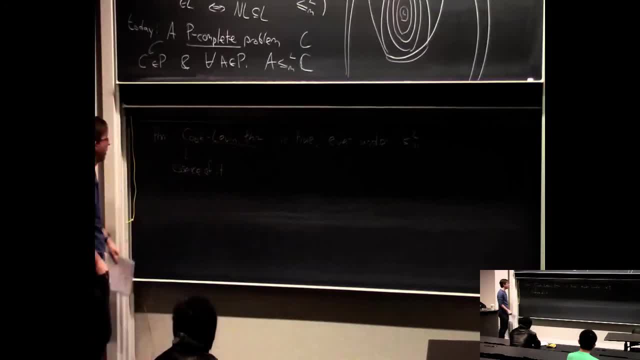 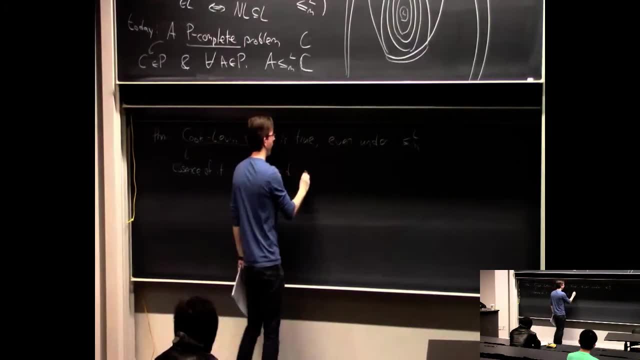 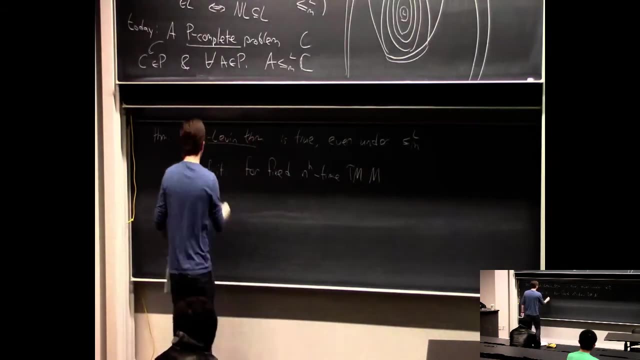 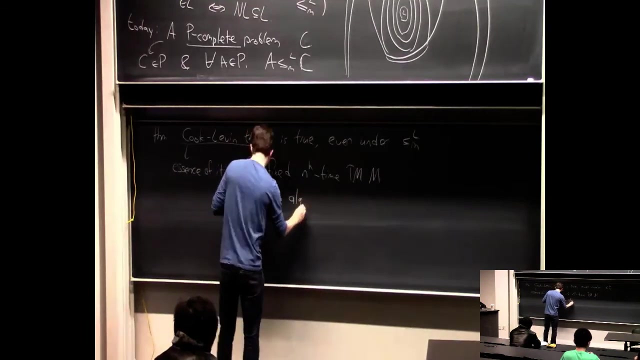 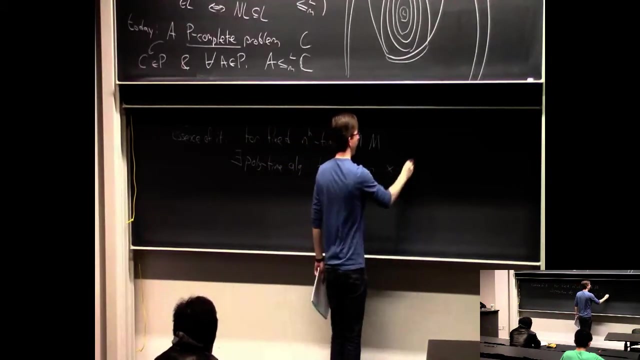 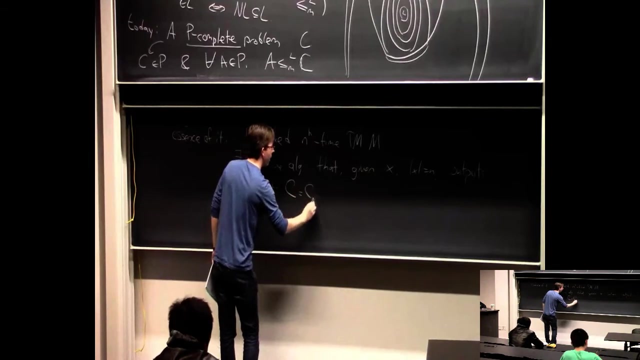 So let me give you some details about that. So for a fixed n to the k time Turing machine m, there exists a polynomial time algorithm that, given a string x of length n, outputs a circuit c which depends on m and x. actually, 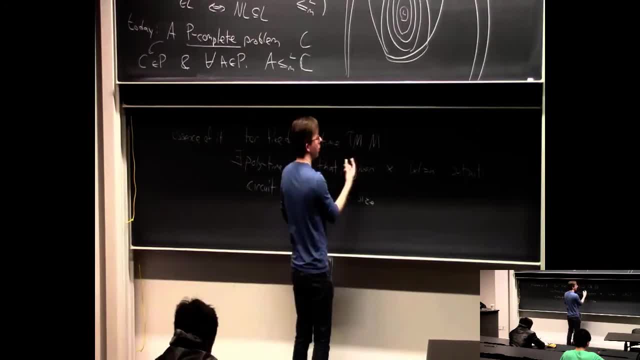 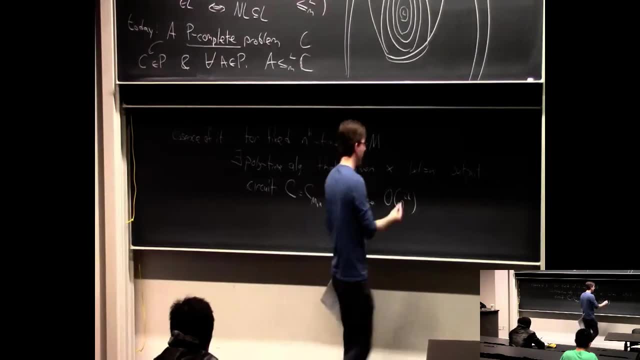 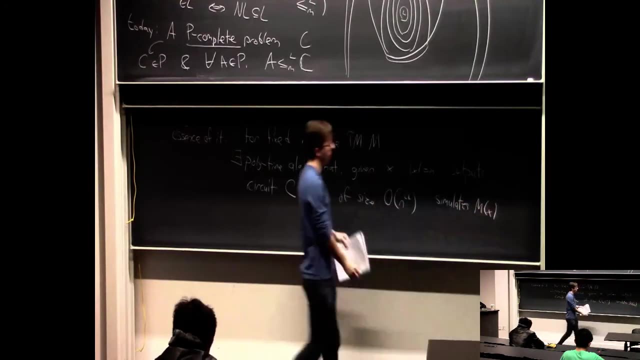 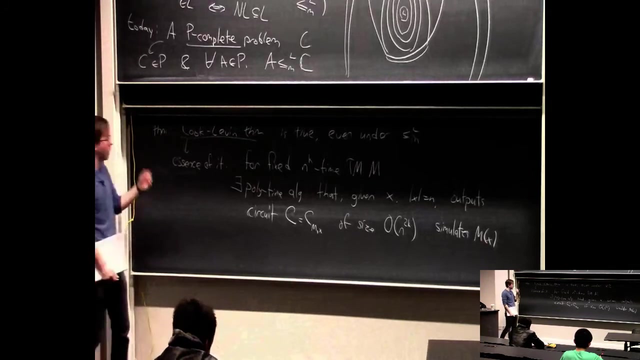 of size not too much bigger than the running time of m. so in fact, the square of it, the order n to the 2k that simulates m on x, And this was basically the proof of the Cook-Levin theorem. Actually, it's a little bit more subtle than that. 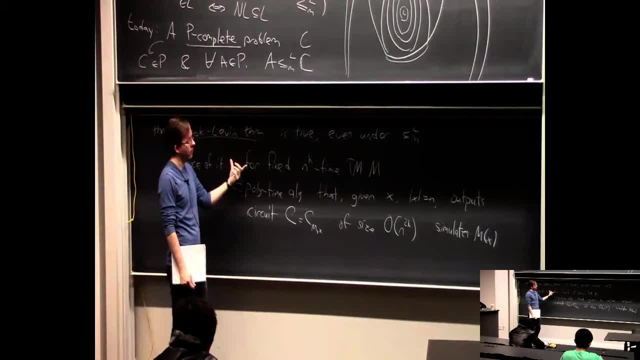 So in the Cook-Levin theorem this is actually a verification algorithm, So it actually has two inputs, x and y, and you build the circuit that has the computation of the verification algorithm with x like sort of hard-coded in. 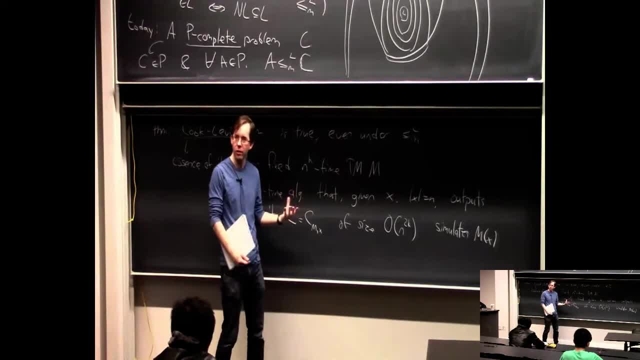 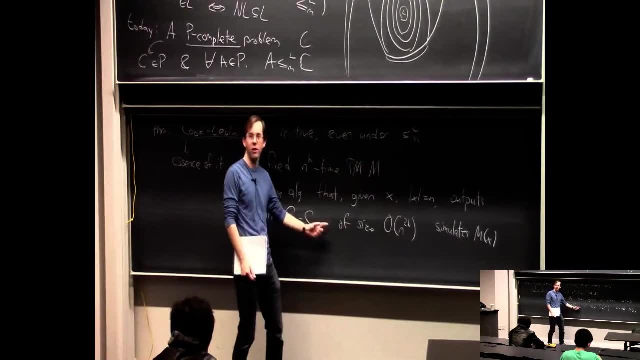 but, like the y part, still has variables. And then you say that, well, there exists a y that makes the verifier accept if, and only if, the circuit you produce has the property that there exists a y that makes that circuit output one. 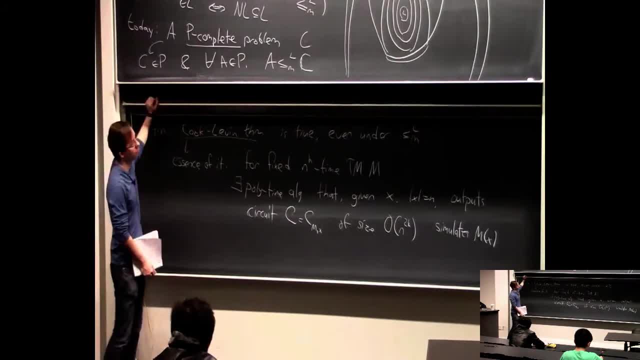 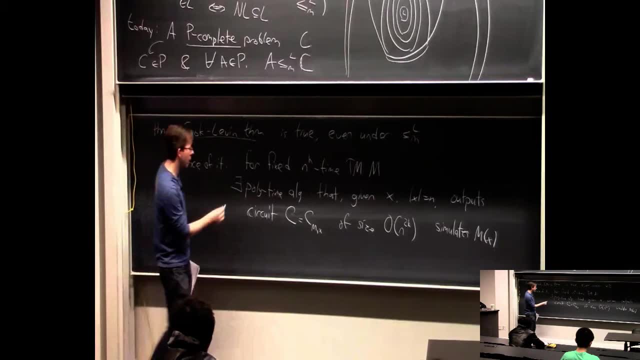 And the situation with the p-completeness of circuit value problem is actually even simpler. And what I'd like to show you now is just- or sketch for you now very briefly, is that this polynomial time algorithm is even doable in log space. 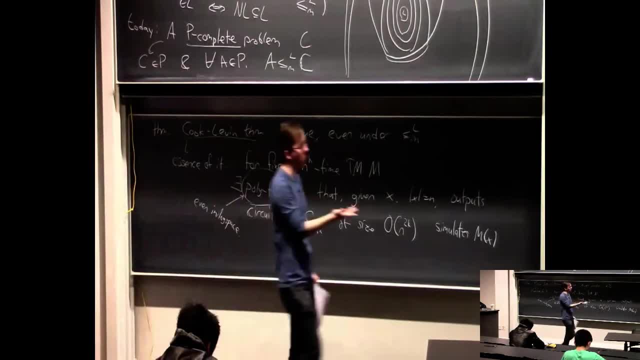 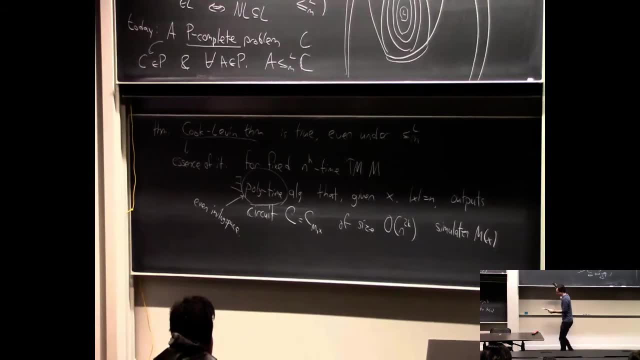 And really the proof of this is like, not much more- I'm not going to sketch it- really- much more than this proof because in the end they're kind of similar. Let me just draw a picture. Sketch of claim. 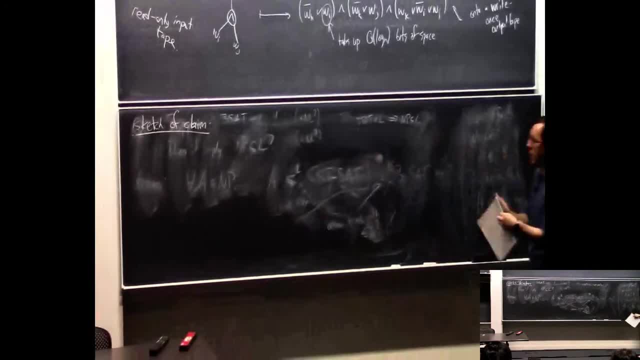 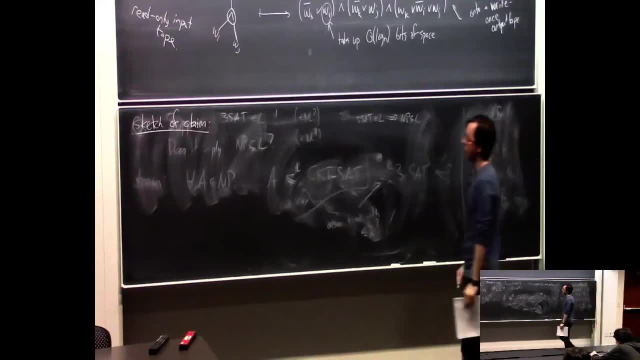 So how did this work? You had a fixed Turing machine, m, an input string X, and you want to build the circuit the kind of did M on X. so the circuit was kind of divided into layers and sort of each layer. well, each layer has some wires and these wires encode the configuration of M on 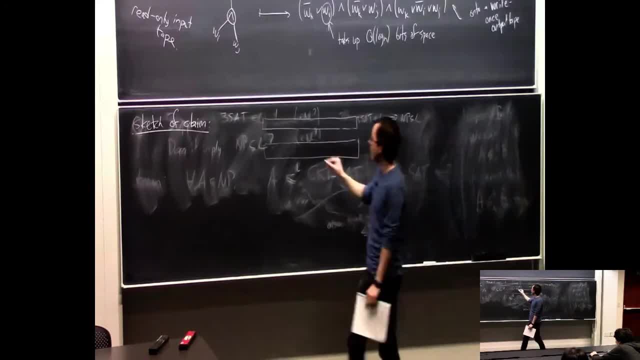 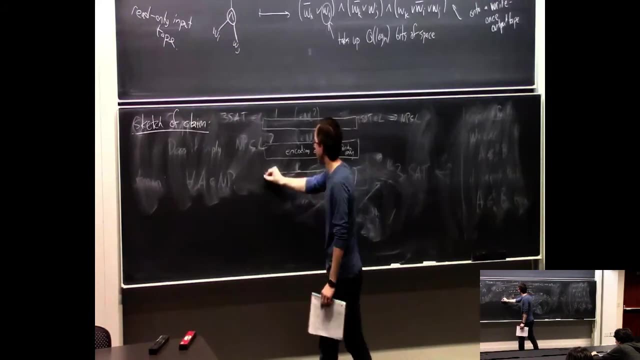 computing on X at each time step. so this was like somehow in the circuit you had an encoding of you know M's second configuration here in this picture. then you had wires that encoded M's third configuration and so forth and so on. so this first configuration kind of looks like encoding of Q, 0 and X and maybe, if 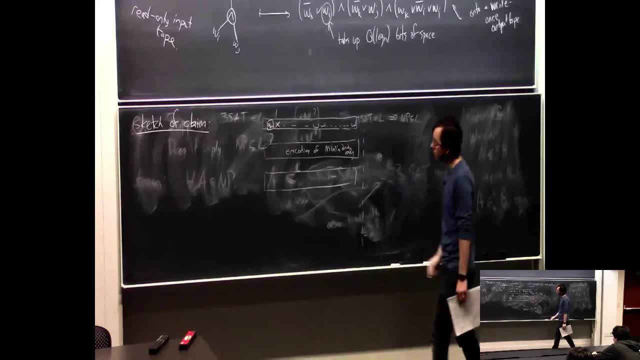 you want to make them all the same width, you can put blanks out here. okay, so since that's the way it's going to be, it's going to be a little bit more complicated. M runs in time n to the K. it never uses more than n to the K space. so all the 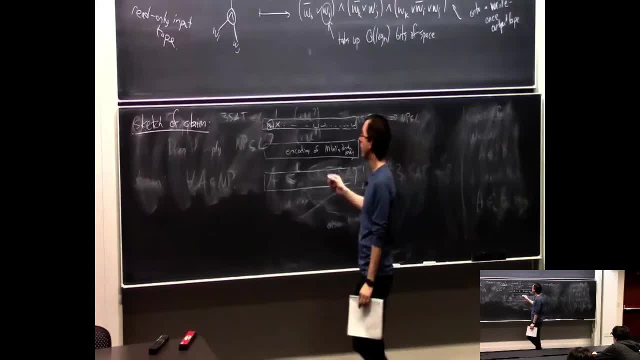 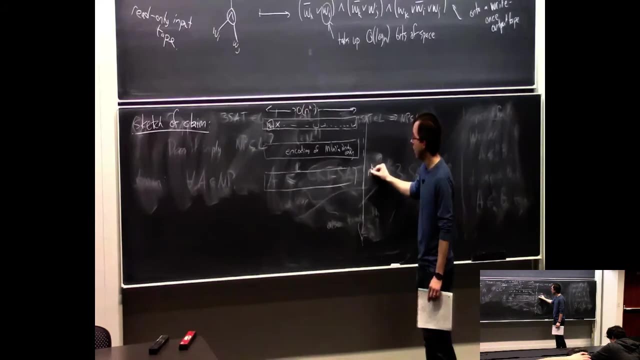 configurations have no more than n to the K characters. so basically, though you know, the width here is order n to the K and since it runs in order n to the K time, like there are no more than n to the K different configurations, so this whole list of configurations is sometimes called the. 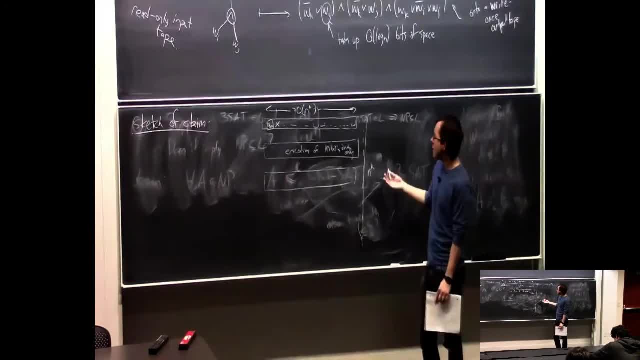 tableau of the computation of M on X and the total number of bits in it is something like n to the k times n to the k. so that's where the order and to the 2k comes from. so maybe there's this many fires, okay, and basically a bit like this: 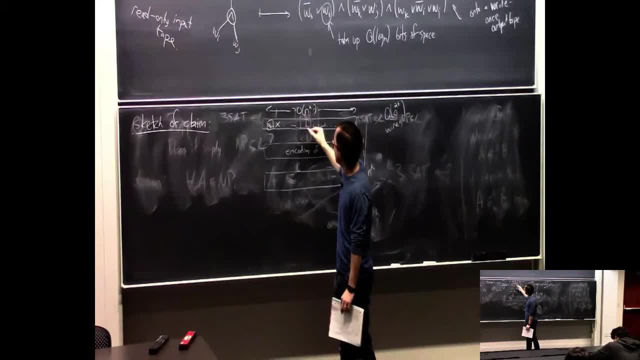 actually for every. you know. you know three cells up here which are actually encoded by constant number of bits in every cell down here. you put some kind of gadget here that can locally check that this position of the configuration is what it should be, if this was the right encoding. 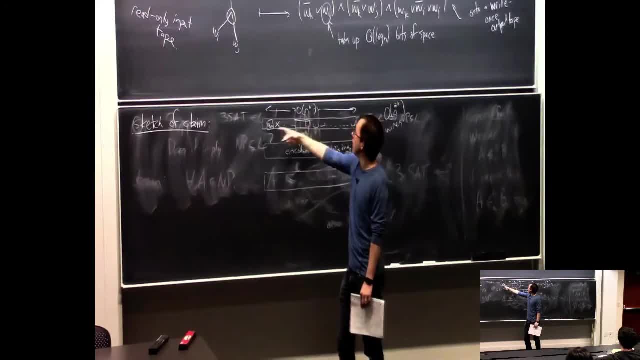 of the configuration that followed from this one. If there's no state symbol here- it means the head is nowhere near here- then this symbol will just be the same as this symbol, And the gadget also checks to see if you have the encoding of a state symbol here. 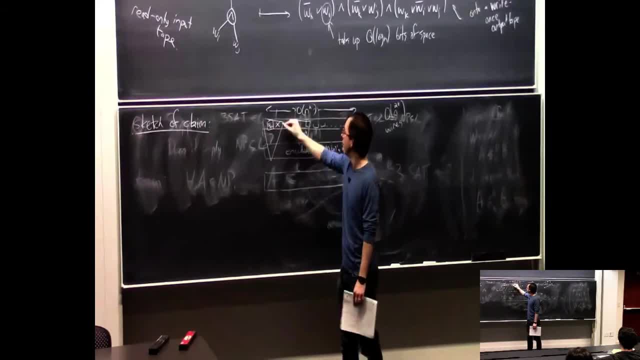 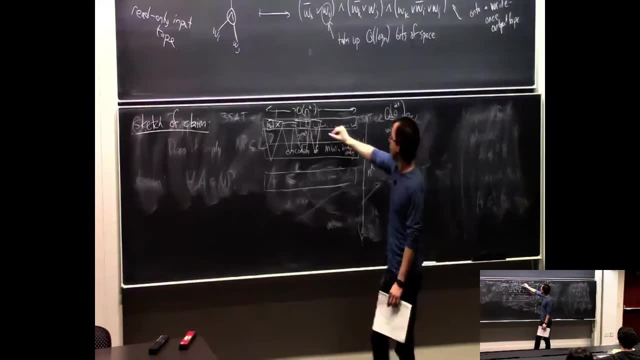 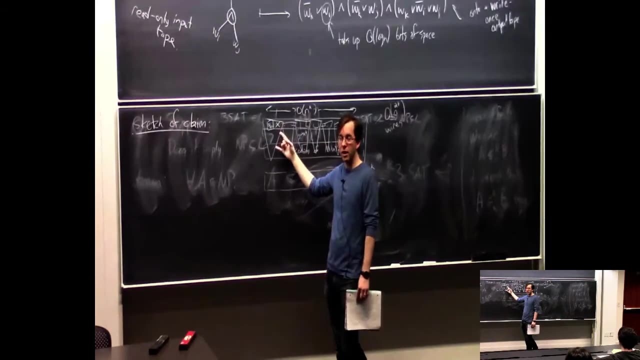 then the right small change happens down here and so forth. So this is quite a sketchy sketch of what you did in one hour, but the point is you basically set up a circuit that has many, many, many copies of this gadget circuit. 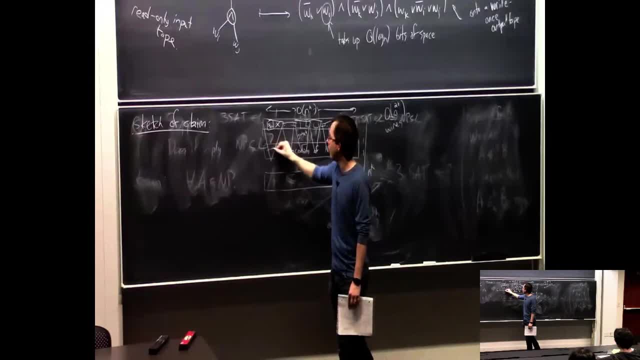 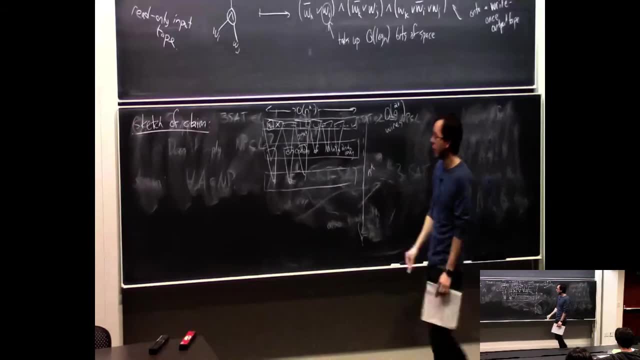 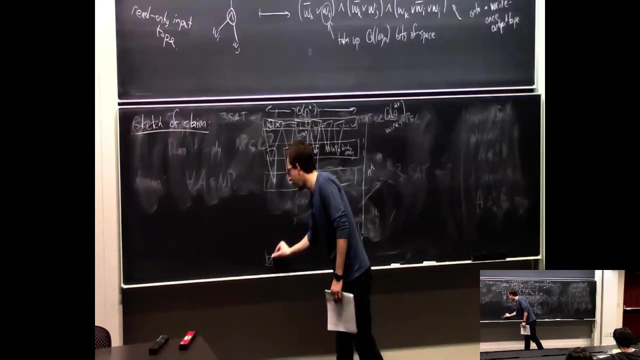 of constant size which locally checks that every piece of each configuration follows from the preceding pieces of the configuration. OK, and then finally, the output of the circuit is: you have a little other circuit here that checks if the final state is an accept state or a reject state. 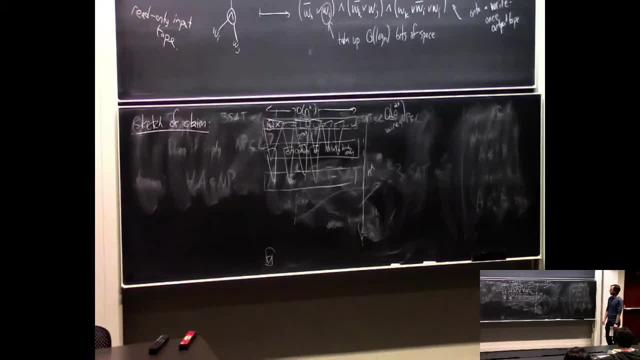 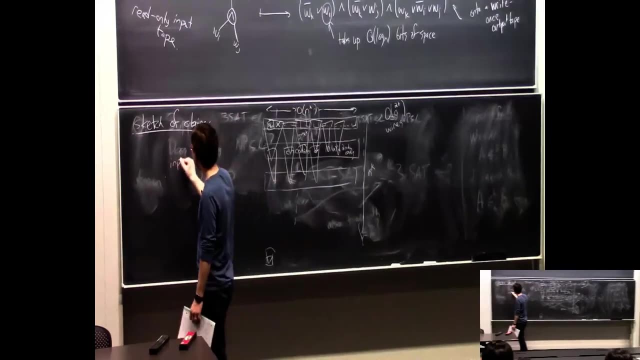 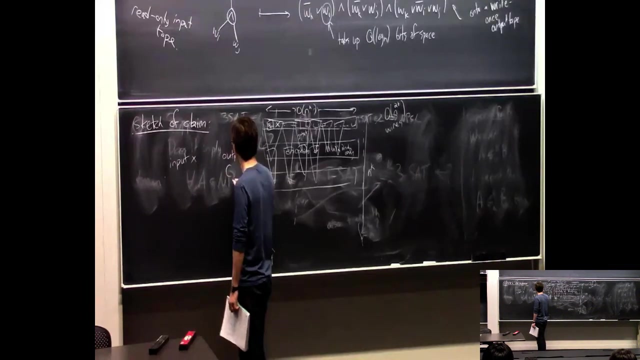 and outputs 0 or 1, dependingly. So at the time we argued that this could all be done in a polynomial space, And really this is: the input, remember, is x, Capital M is considered And the output is this circuit C. 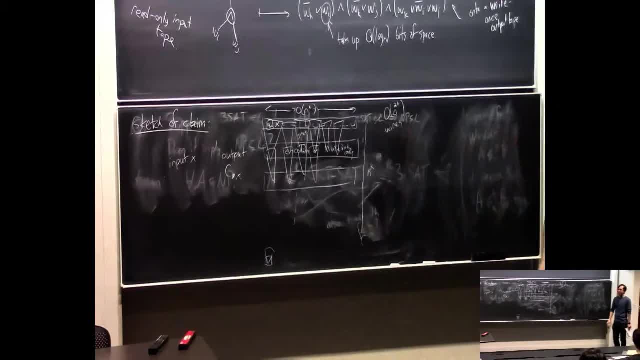 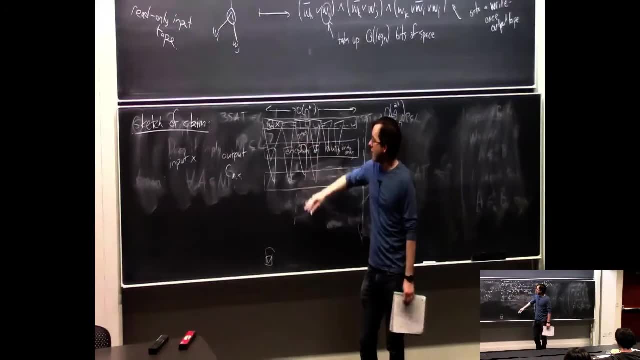 And I just want to claim to you that it can also be done in log space, And the high level reason is actually: all this stuff is quite simple, It's very just repeating. In fact, the only part that involves the input is up here. 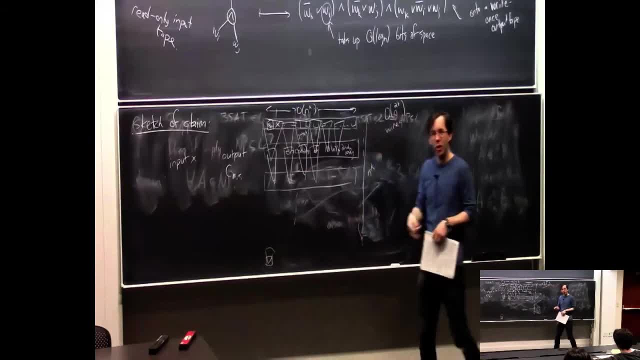 But basically you're putting the same copy of the circuit gadget down over and over and over again and just connecting up it carefully. So there's no problem. OK, There's not much difficulty, if you really get into it, in just showing that you can do it. 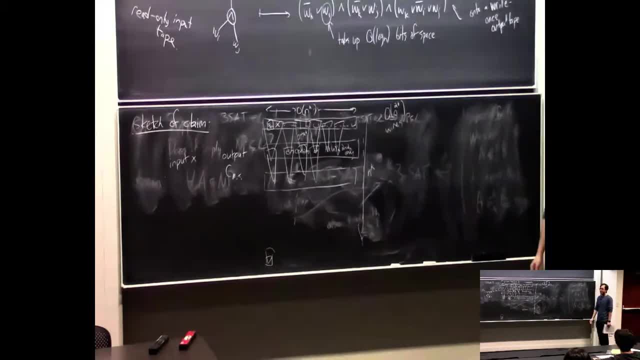 with a write-once output tape. Yeah, So when we have issues writing every line of the tableau, or we don't do that, we only do it for one gadget at a time and we sort of forget that previous gadget. So the algorithm doesn't actually write the tableau. 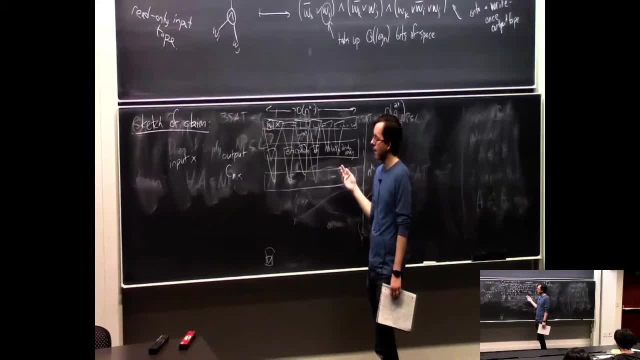 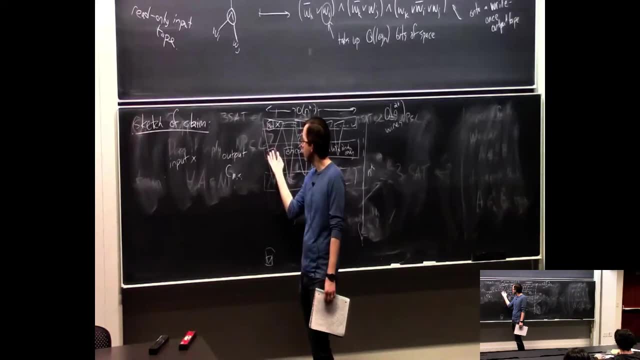 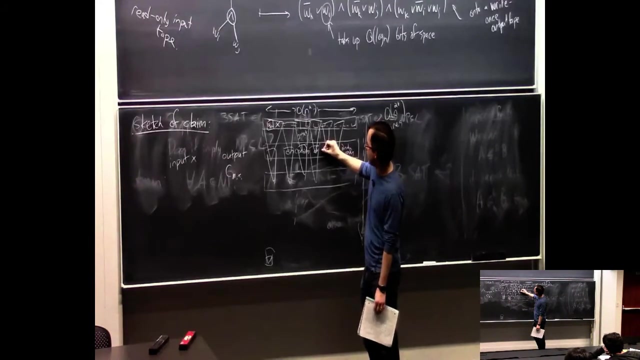 It writes like it writes gadgetry that well, yeah. so yeah, I'm not sure how to answer this question without getting into an extreme amount of detail, But you're basically writing the description of a circuit in which each gate here: 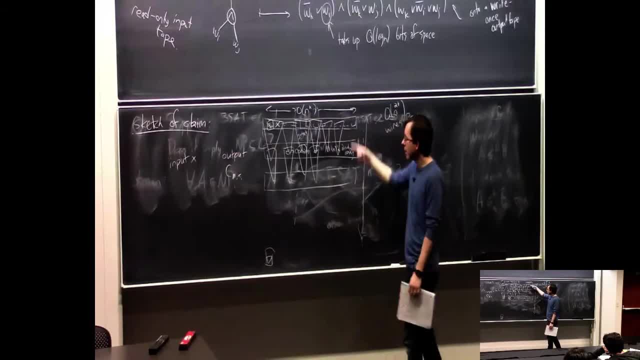 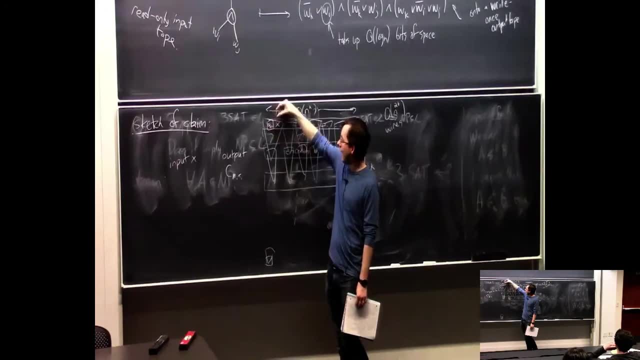 depends on a constant number of gates back here And it's sort of- except for the beginning part where you have to get x involved, because you have to sort of check that x is hard-coded in this, And then you have to get x into the top here. 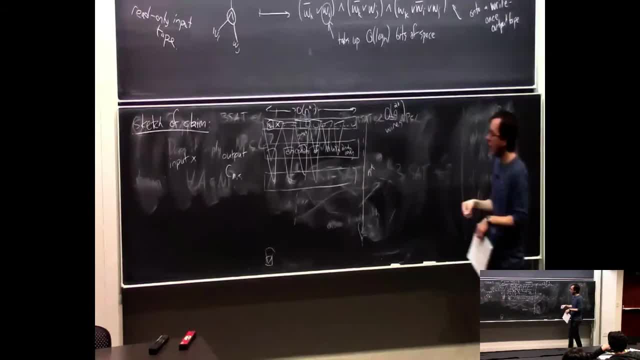 It's the same kind of constant gadget at each time, So it has to keep track of the indexes of positions back here. But it's kind of a very repetitive and methodical process. So yeah, I guess I'm not going to get into much more detail. 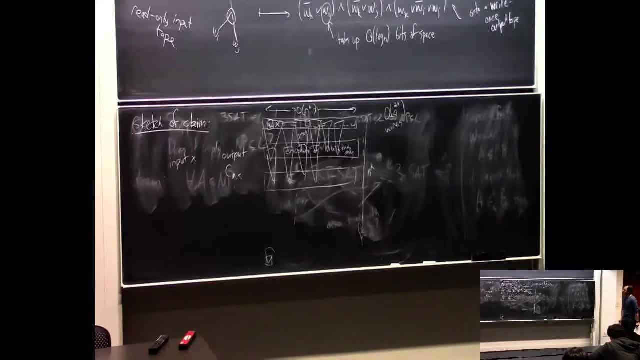 than that. OK, So let's assume you believe that this can be done in log space. Then we actually have some constant gadgets And I'm going to show you some of the consequences, And actually the easier consequence, the first consequence. 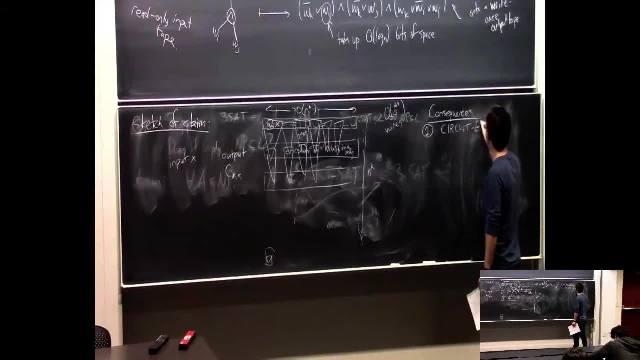 is this fact that I want to claim that the circuit evaluation problem is p-complete. So, in fact, we know that circuit evaluations in polynomial time. I give you a circuit and a string. What is the circuit output? That's easy. So what I'm really claiming is that it's p-hard. 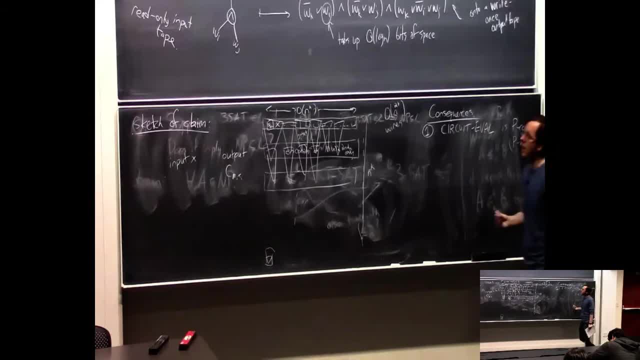 And what does that mean If it's still up here? it means that for every language a and p, it reduces in log space to circuit evaluation. So why is that true in words? Well, suppose you have some language a in polynomial time. 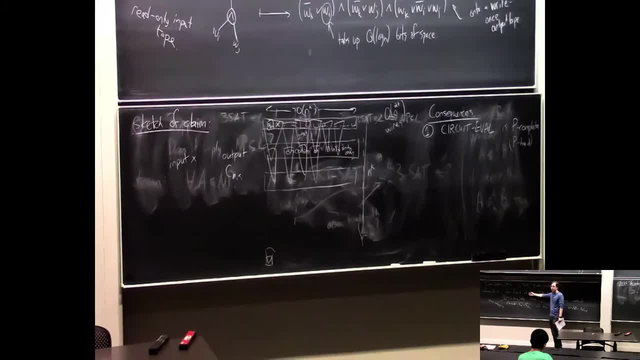 It's decided by some Turing machine, m, running in some polynomial time, like n to the k. So we need a log space reduction that takes an input string, x, And it's trying to reduce in some polynomial time. It's trying to decide if x is in a. 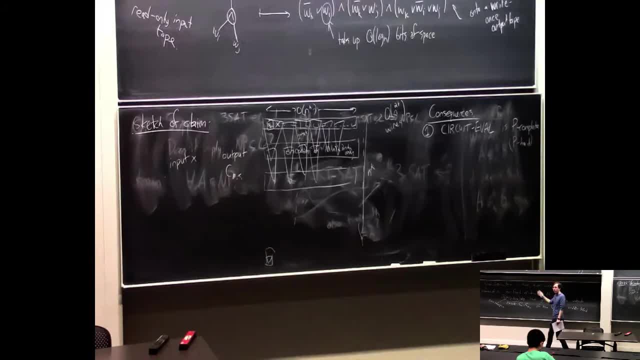 And what it does is it converts it to an equivalent circuit value problem. whose answer gives the answer to whether or not x is in a And what is the reduction? It's exactly this. The reduction has m fixed and it takes the input x. 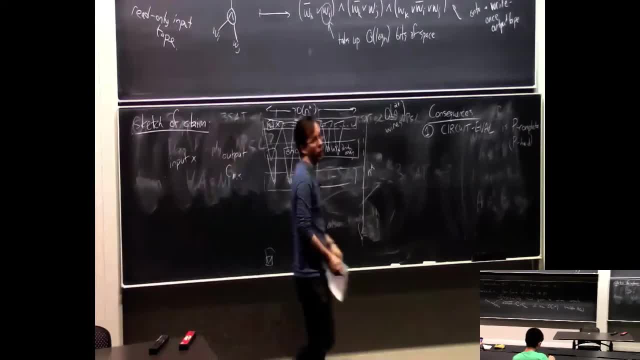 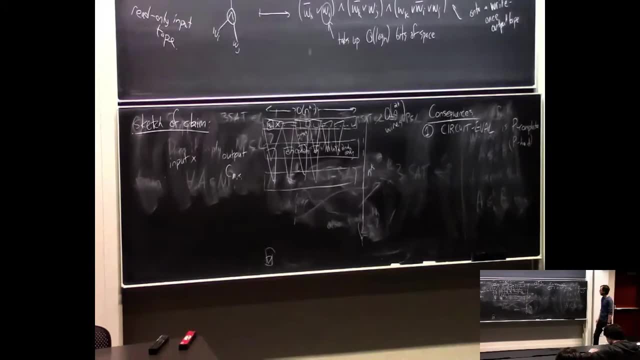 and it reduces it to this circuit and the question of whether or not this circuit outputs 0 or 1.. That gives the correct answer for whether or not x is in the language a. OK. So that's one consequence, And the other one is the Cook-Levin theorem. 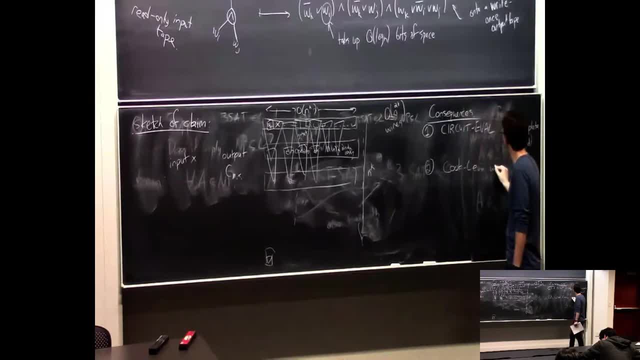 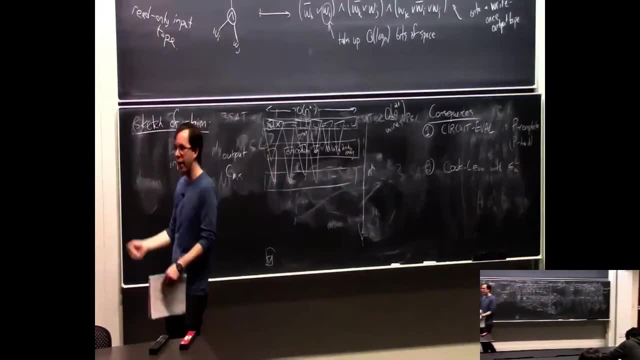 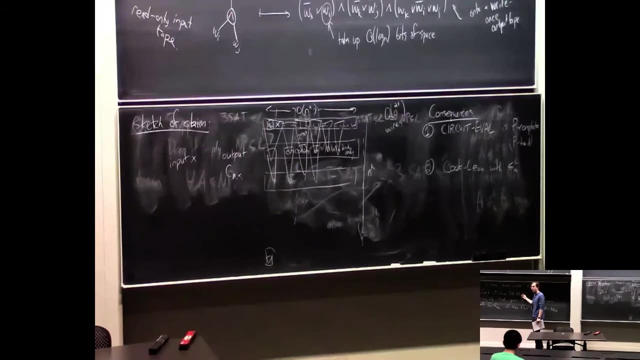 with log space reductions. And that's the same story again, except now it's a little bit more complicated because the Turing machine is a verifier, so it has this extra input y. It's the same sort of situation: Given an x, there will be a y that makes the verifier accept. 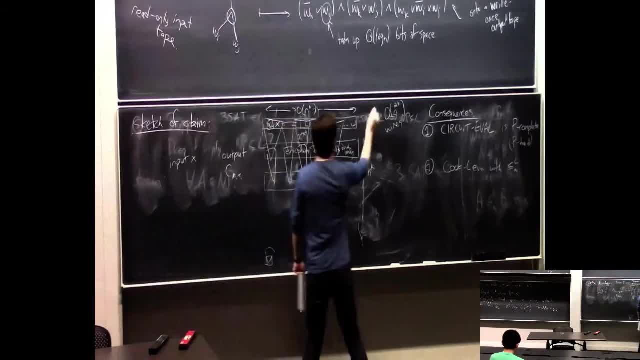 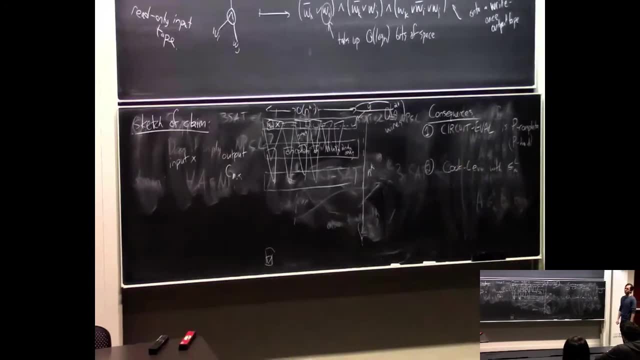 the verifier Turing machine. if, and only if, there's a y that goes into the circuit Here. Here, That makes the circuit output 1.. OK, So this is a bit technical stuff, but this is good to know and this is also very good to know. 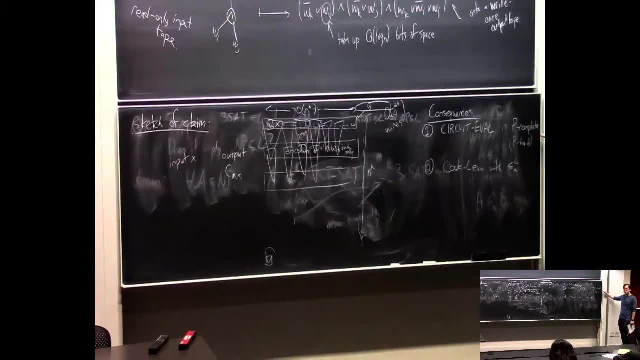 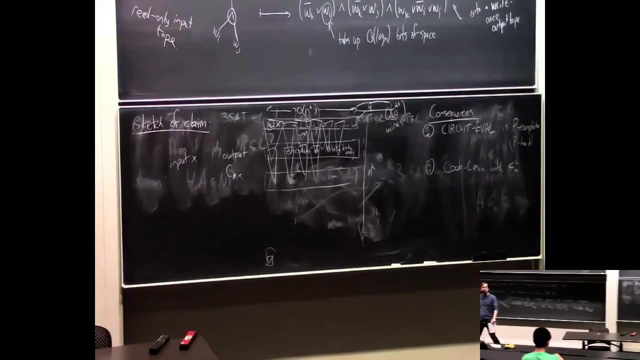 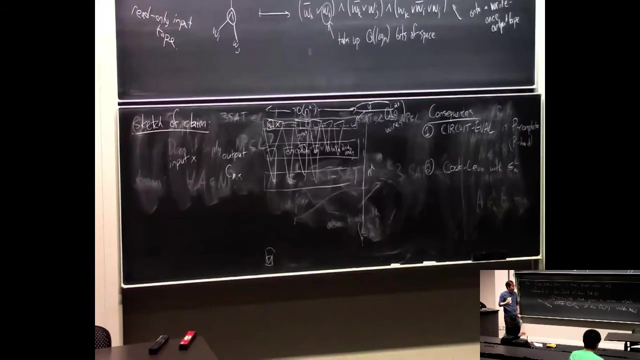 The canonical example of a problem that's the hardest problem in P. OK, Any questions? Great OK. So we got this diagram. We know the ST path is a complete problem here. Circuit valuation is a complete problem here, You know. 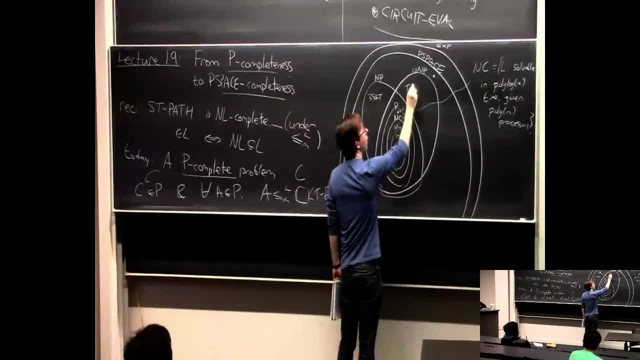 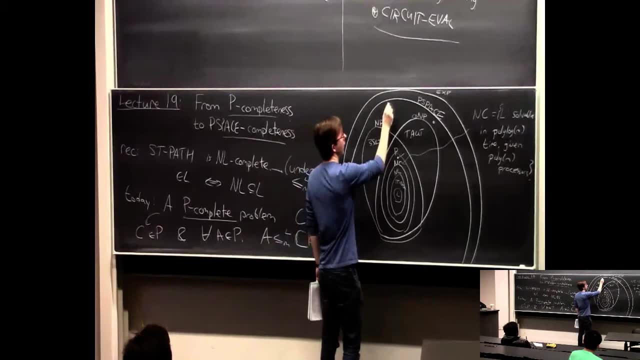 3SAT, or circuit SAT, was a complete problem here, Tautology was a complete problem for coNP, And the last thing I want to talk about today, which hopefully I'll be able to finish, is a problem that's complete for PSPACE, which will be called for some reason. 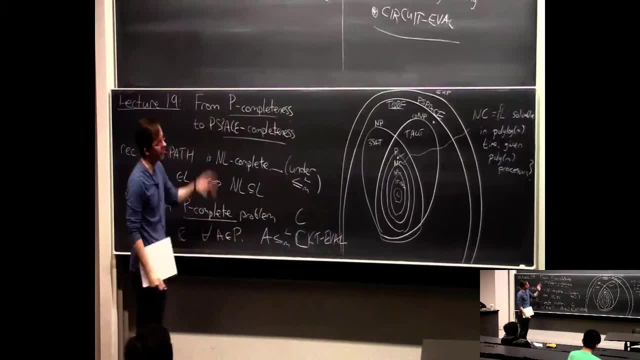 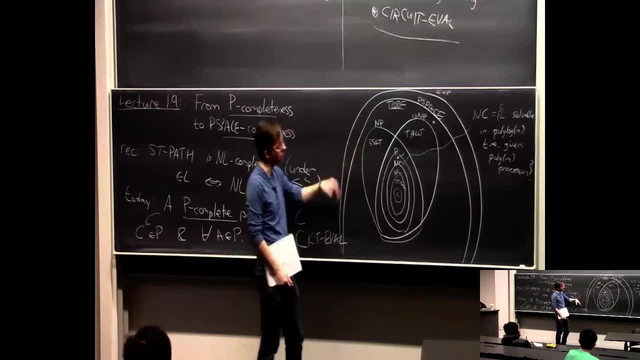 TQBF And then x. I don't care about x time, It's pretty big, So we'll kind of have a complete problem for all these nice complexity classes: PSPACE, NP, P, NL, et cetera. 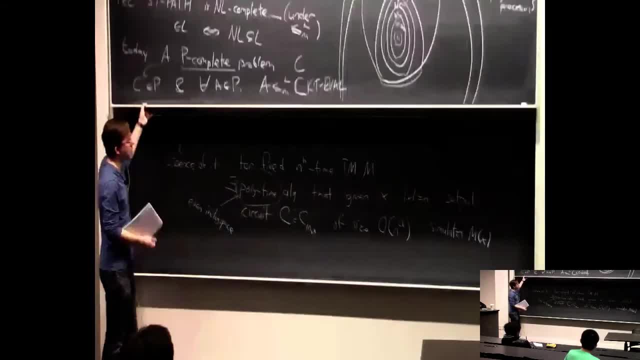 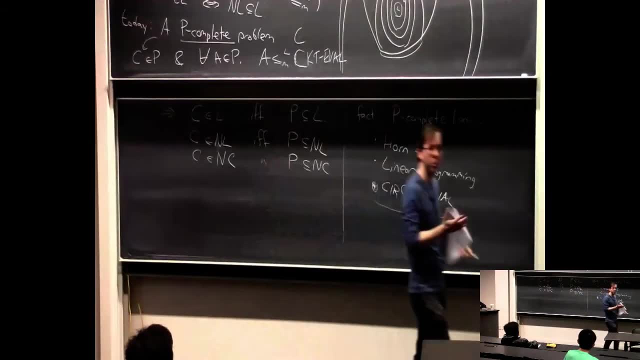 OK. So, as I mentioned a couple times, to really understand a complexity class, or appreciate a complexity class, is to have a nice problem which is complete for it. So that's what we're going to do for PSPACE, And then we'll have a very complete picture. 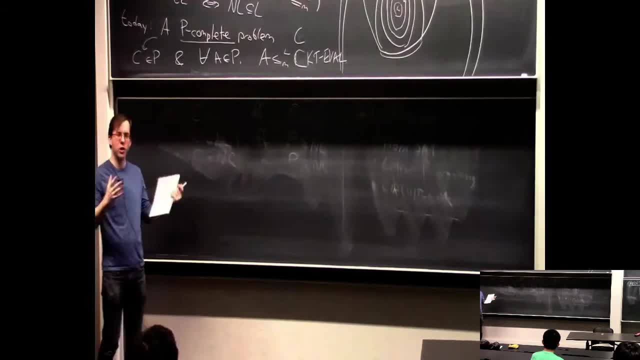 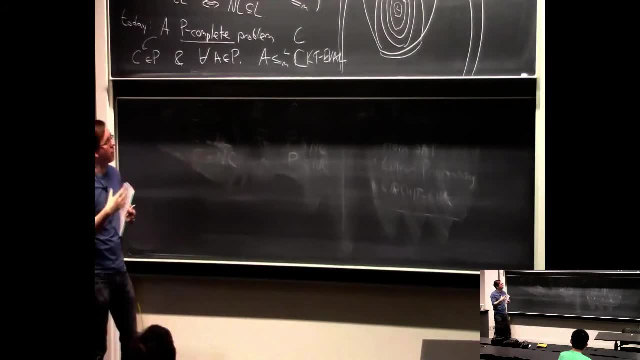 OK, So let me introduce you to. actually we have to change our mindset a little bit. We've been talking for a long time about things inside P, like these really feasible things, And trying to understand. can you get it down to log space? 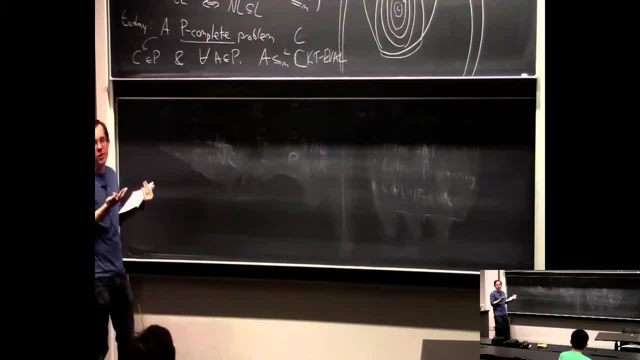 or whatnot. Now we're actually jumping up to a very crazy class. I mean, it's all the things you can solve in polynomial space, which is very liberal. It's much bigger than polynomial time. presumably These are not actually feasible problems, seemingly. 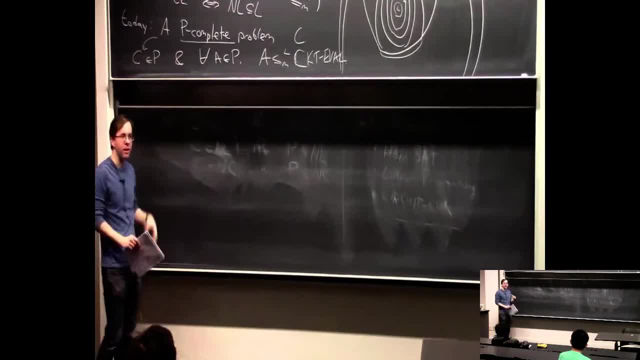 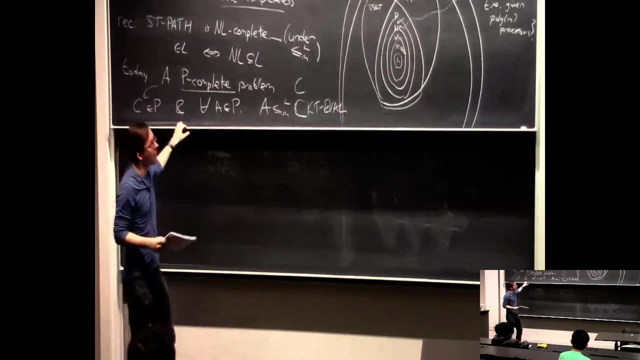 that we're going to talk about. But I think actually PSPACE is kind of the class. that's sort of the limit of what is not definitely crazy. Like you know, people tried to code up SAT solvers, Anyway, even though SAT is NP-complete. 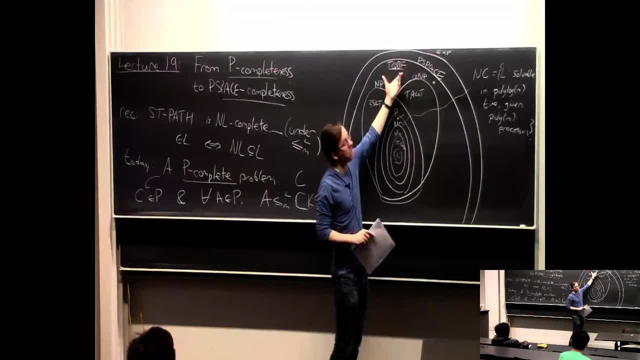 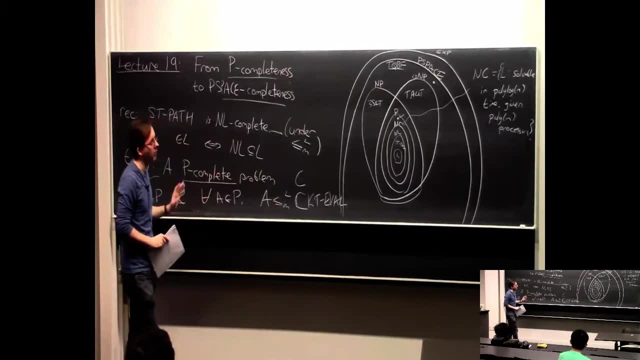 And I think you know they even attempt to. I know people that attempt to code up solvers for this problem, even though it's PSPACE-complete Somehow. once you get beyond PSPACE, you're really in the realm of like there's. 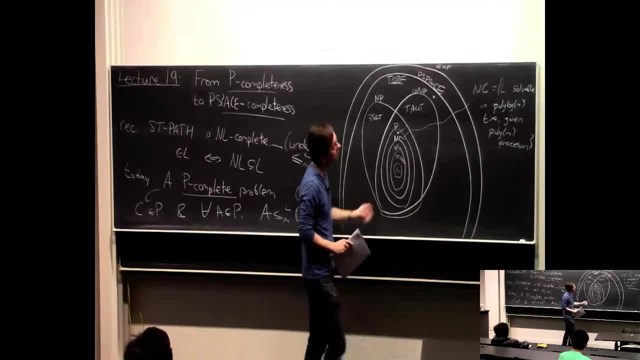 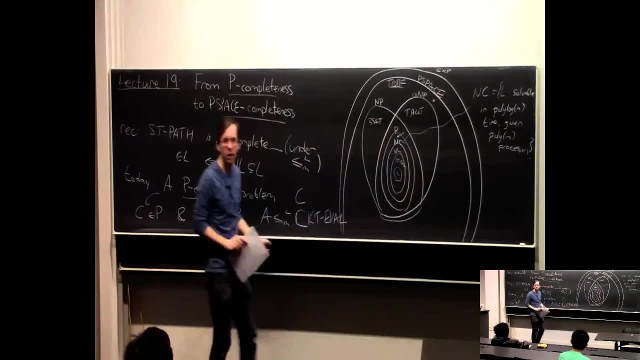 no way that you can consider this genuinely possibly practical. In fact, we know that once you get into exponential time, we explicitly know there are problems there that are not solvable in polynomial time. by the time hierarchy theorem, But actually as far as we know, PSPACE could equal P, Although 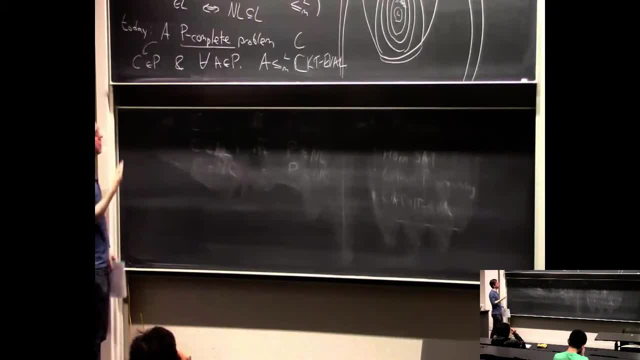 it's very unlikely. So just to change your mindset a little bit, now we're talking about very liberal bounds on computation power, PSPACE. So let me define for you the problem. that's going to be PSPACE-complete. It's a variation of SAT. 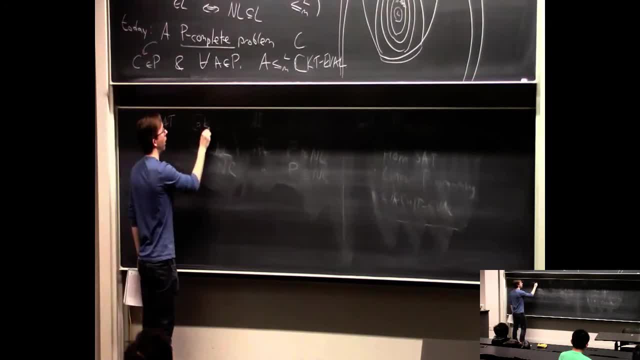 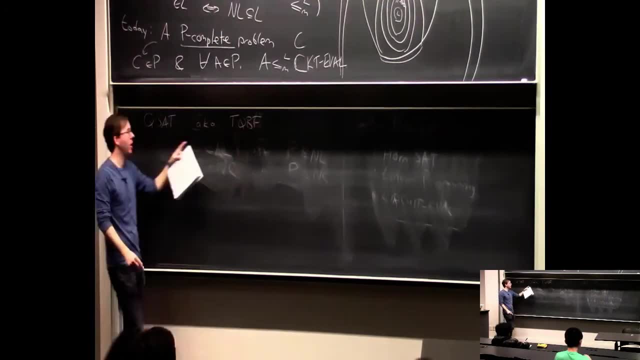 Some people call it QSAT, Other people call it TQBF. I prefer this name, QSAT, But most people call it by this, So I guess I have to go with this one. sadly, So, the Q in both cases stands for quantified. 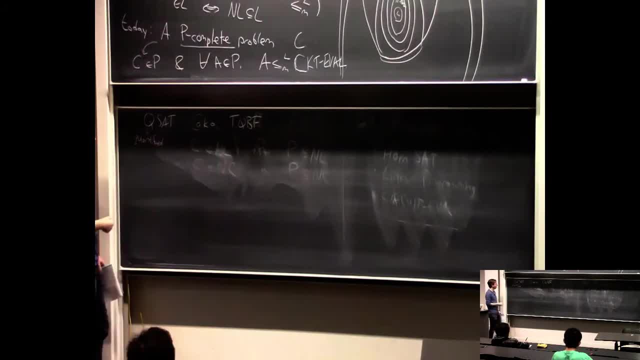 It's a variation of SAT. It's more complicated than SAT. It's quantified SAT. Quantified is going to mean like for all exists those things. This stands for quantified Boolean formula And this stands for either true or totally. 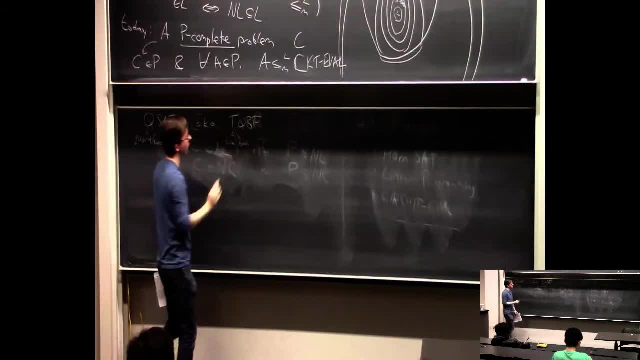 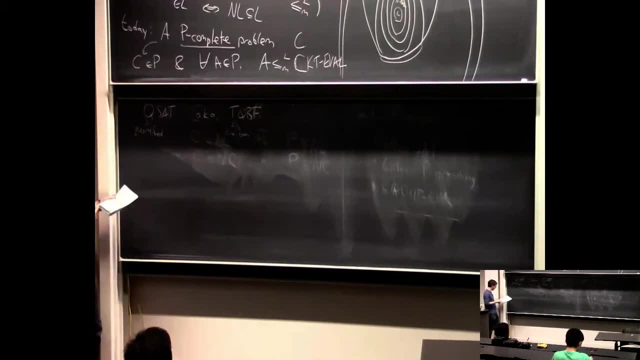 depending on who you ask. So either totally quantified Boolean or totally quantified. So this is the quantified Boolean formula or true quantified Boolean formula. But enough about the name. What is the problem? So here's the problem. 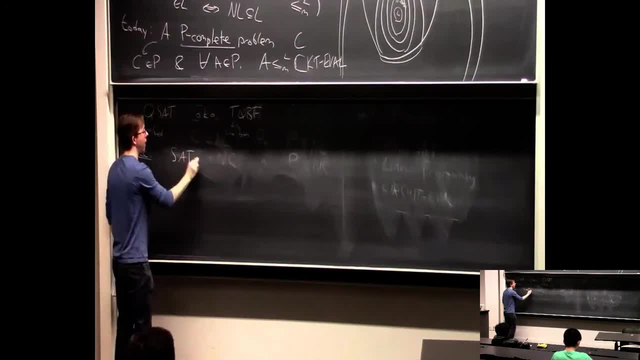 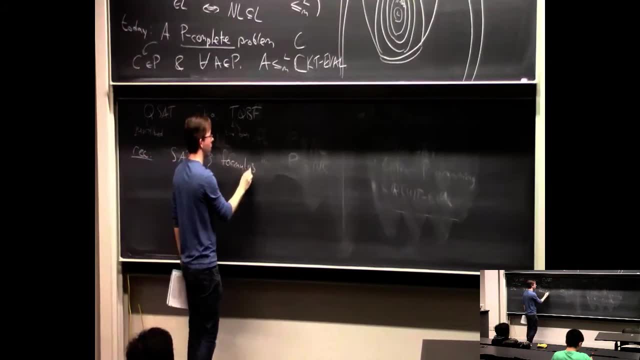 Let's first recall what is SAT problem? I hope you know, but it'll be good to compare it with QSAT. So SAT is all the language of all formulas, propositional formulas with Boolean variables, phi, such that well, phi is satisfiable. 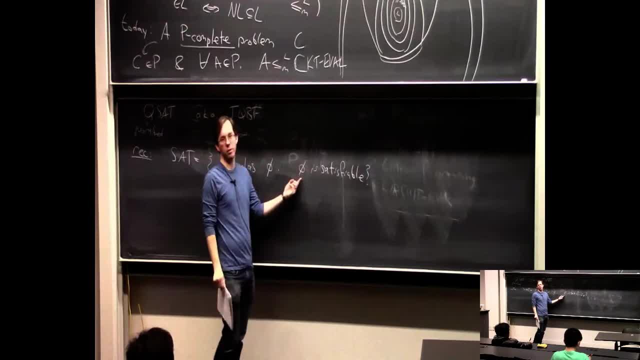 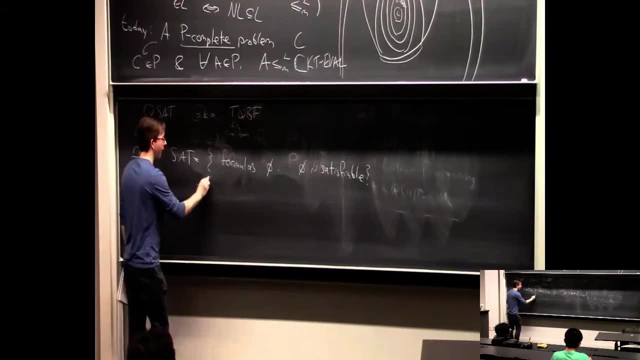 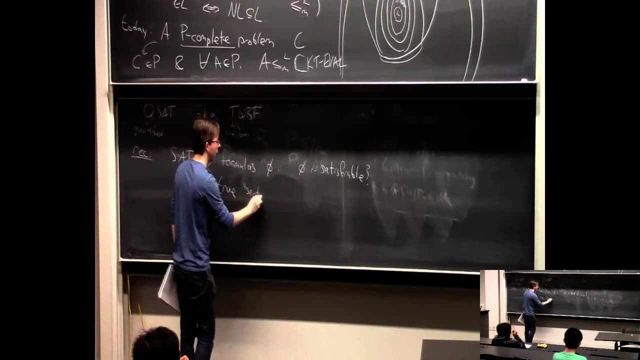 It's just that exists truth. assignment 0 or 1 to the variables in phi, then make it evaluate to true. So let me just write it a different, equivalent way. It's the language of all true sentences. Sentence is like a logic term. 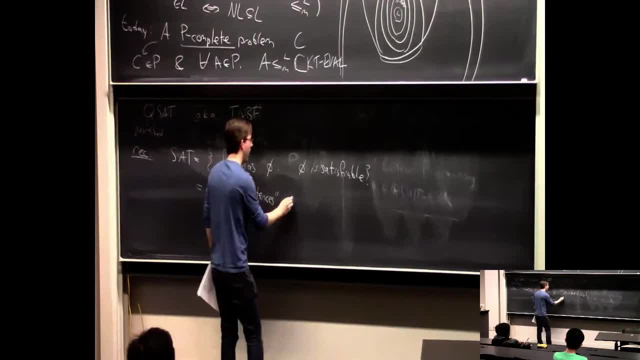 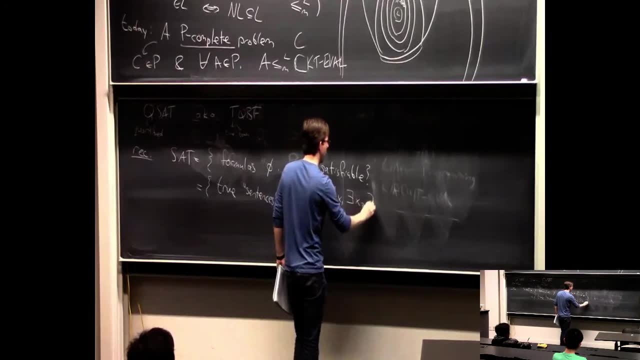 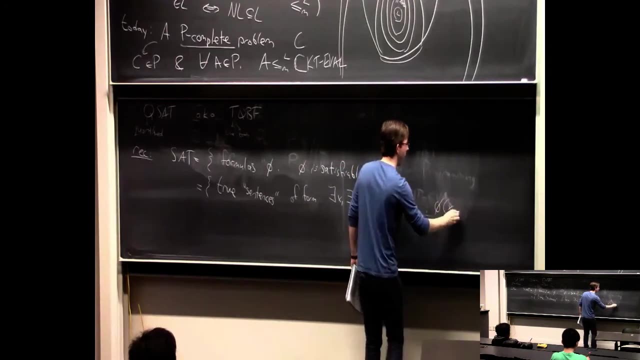 True sentences of this form, of the form. there exists x1, such that there exists x2, such that there exists x3.. These are all Boolean variables. There exists sn, such that phi of x1 through xn is true. Let me write 1 for true. 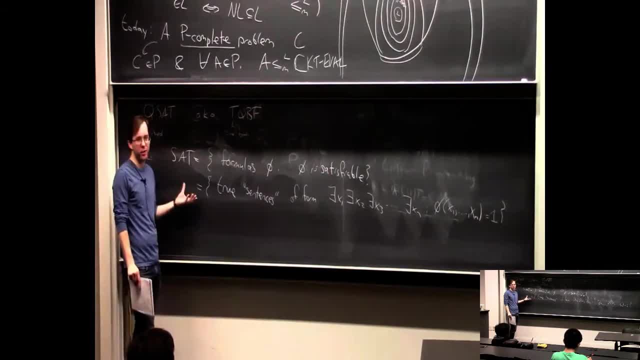 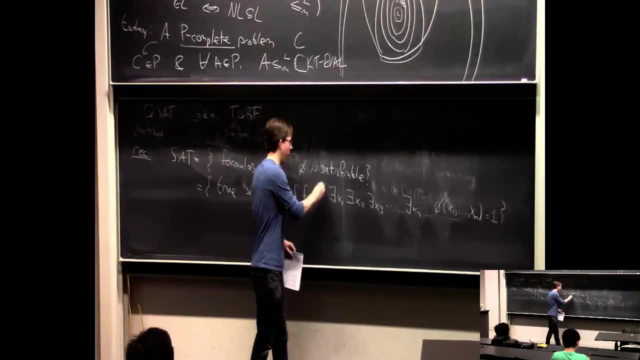 And actually I think this would have been a more natural way to write the SAT problem in the first place, because it's really about existence. This is the whole sentence. I guess this just inherently asserts that something is true, So let me drop that. 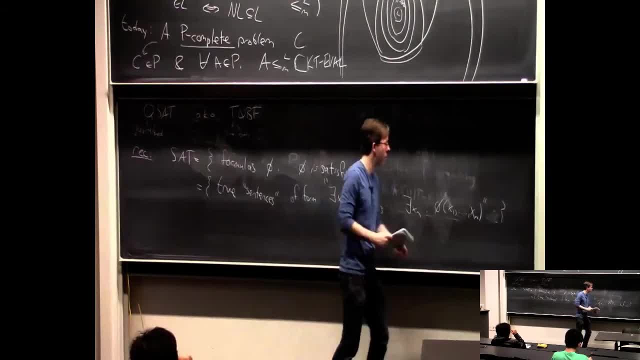 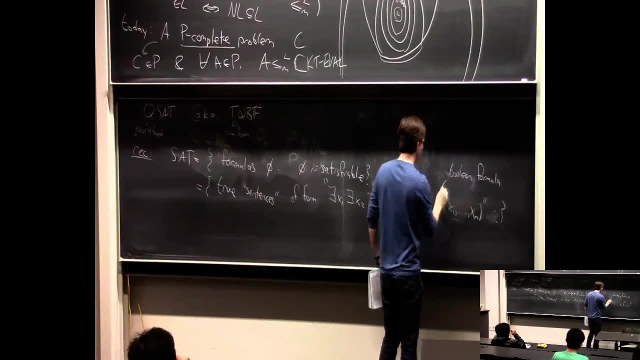 This is the whole sentence. There exists truth assignments for n variables. that makes a certain Boolean formula true And the SAT problem is to check if a sentence like that is true. It's a bit weird actually when you just specify a bare formula. 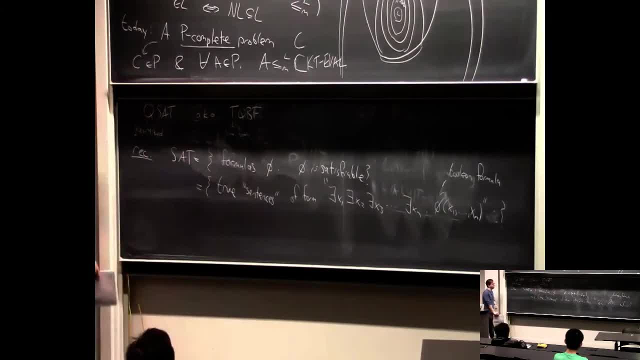 and it's implicit that you're trying to decide if it has a satisfying truth assignment or not. And let me just, for technical reasons, remind you that in SAT we're talking about Boolean formulas that are a bit more general, So they don't have to be conjunctive normal form. 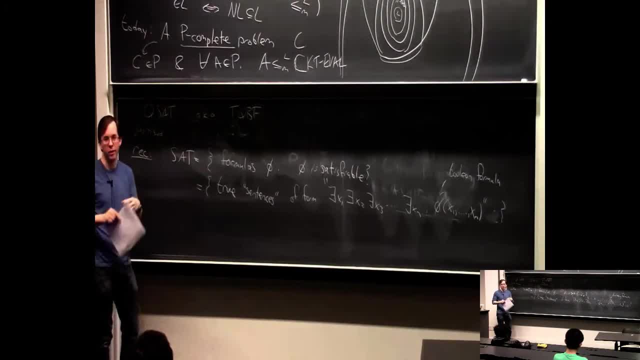 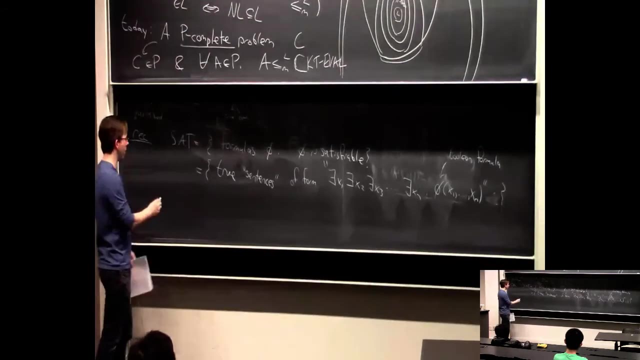 formulas. They can have ors and ands and implies and parentheses and so forth, Any kind of classic Boolean formula. OK, So that's the SAT problem. That's the problem that we know is complete for NP. And while we're here, let me remind you: 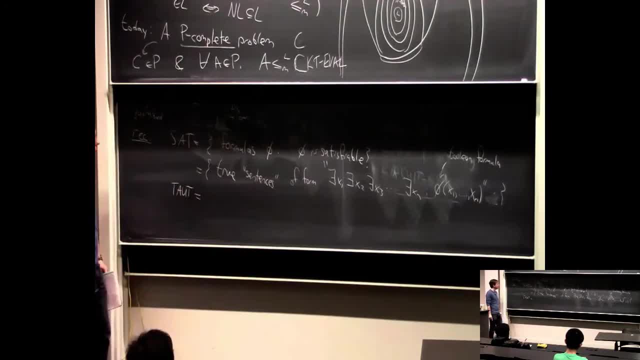 about a lecture that came right before the midterm where we talked about co-NP And we had this class, tautology. This was. we described it as the class of all Boolean formulas that are true under every truth assignment, And it would be quite nice to write that like this. 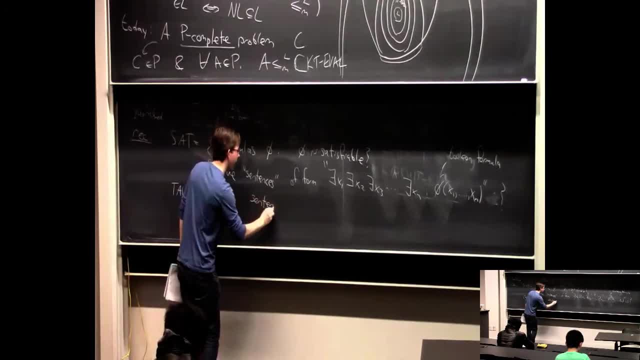 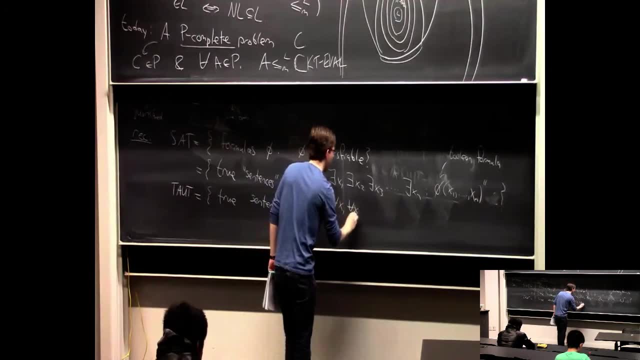 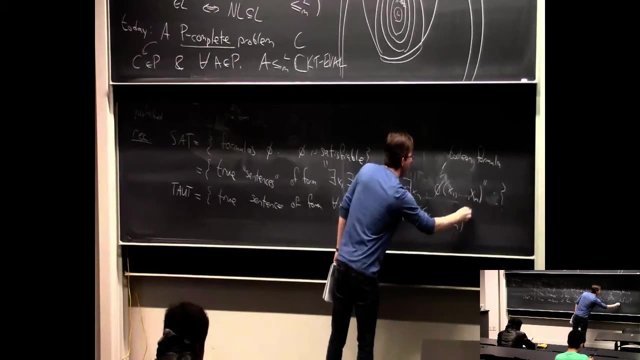 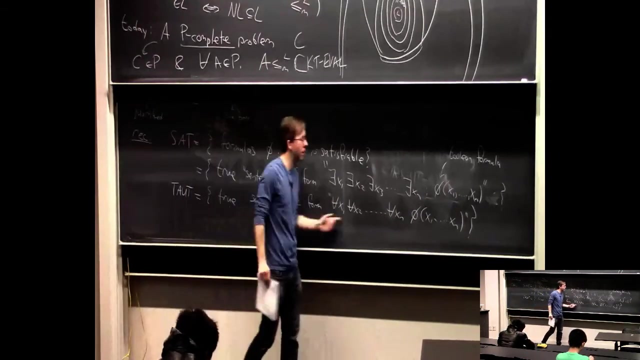 It's the true sentences of the form. well, same thing, but with for all, For all x1, for all x2, for all xn, phi of x1 through xn. OK, So the tautology problem is: I give you a Boolean sentence that: 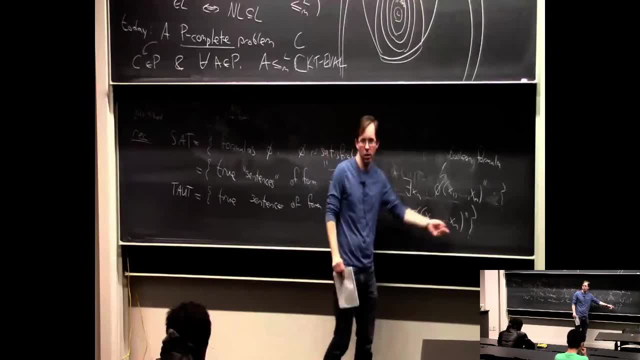 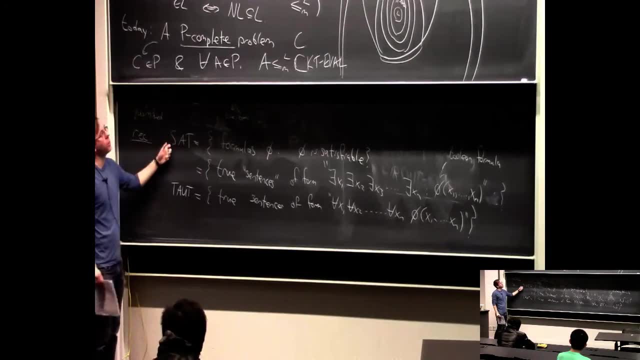 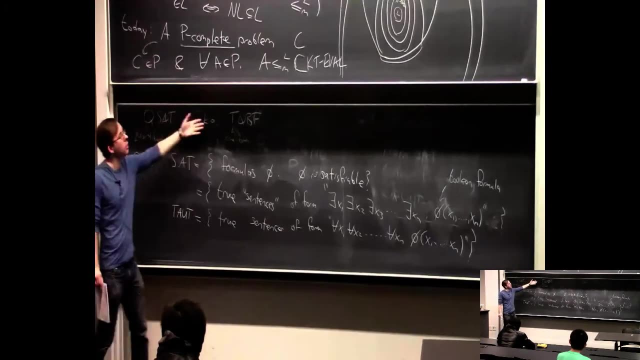 looks like this: It has a bunch of for all quantifiers on its variables and then a propositional formula. You have to decide if that sentence is true or not. And this was complete for NP, This one's complete for co-NP And this QSAT or TQBF problem. 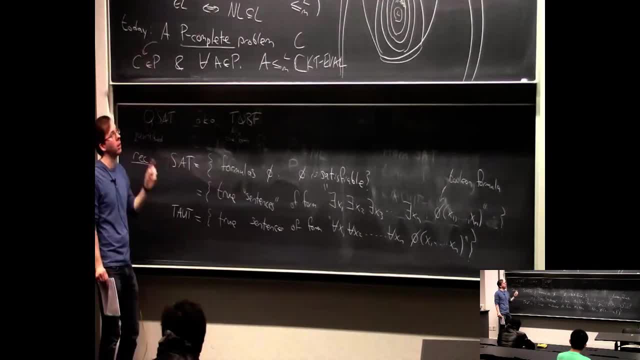 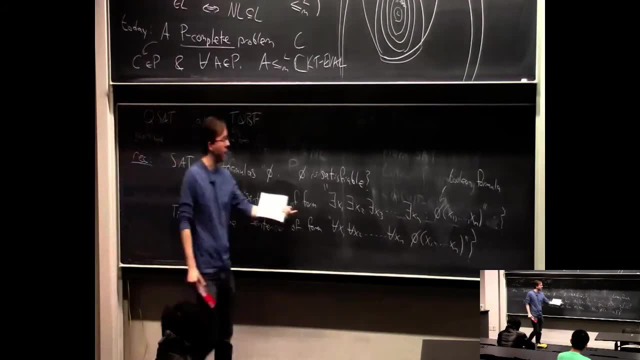 it's going to be a generalization of these two problems. That's complete for the big class: PSPACE: OK, OK, OK. And what generalization is it? It's exactly like this, except you can have any mix of for all, and there exists. 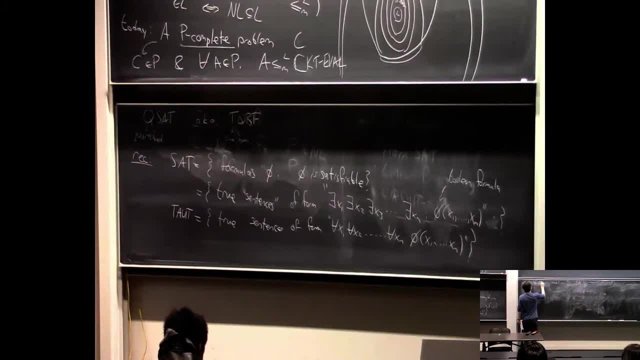 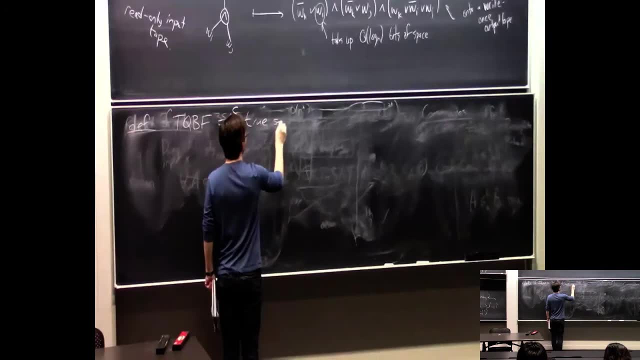 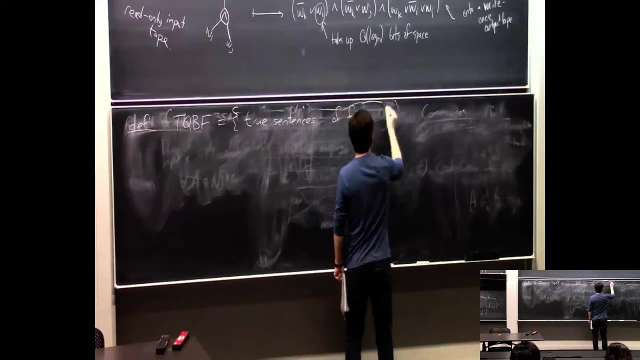 So here's the definition: TQBF is the language of all true sentences, All true sentences of the form, and I'll do it by an example. There exists x1, such that for all x2,, such that for all x3,. 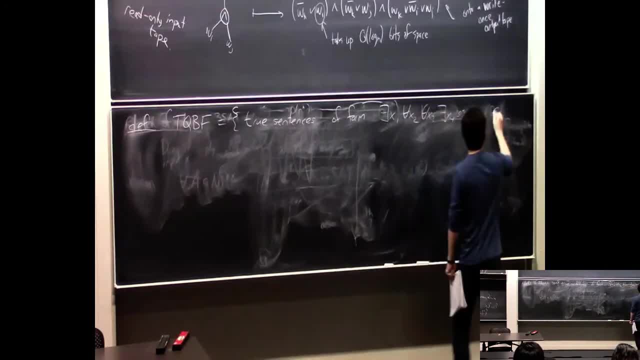 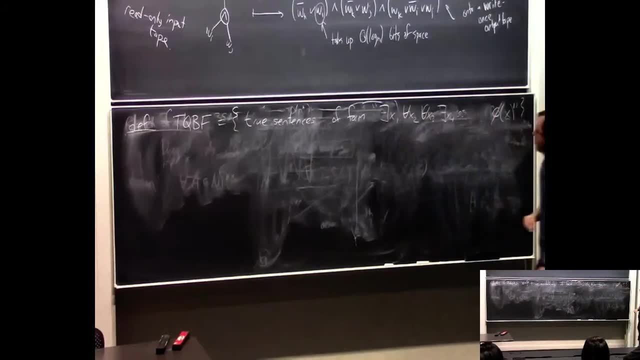 such that there exists x4, et cetera, such that finally, phi of x. OK, And let me just say that the input is really written out. It's like a set of variables, It's like a string in some encoding right. 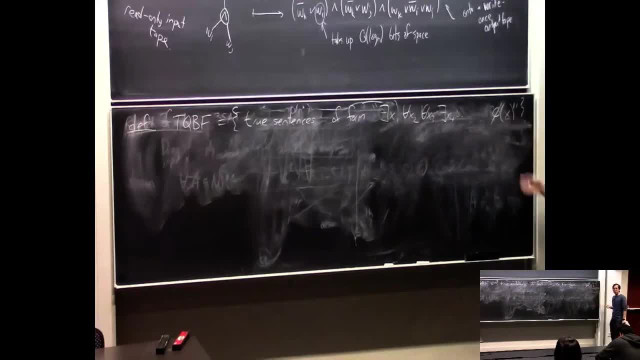 So it really looks like this in some Boolean formula and you just have to decide if it's semantically true. It's true that for every- sorry in this case- that there's some way to set x1 to be either 0 or 1,. 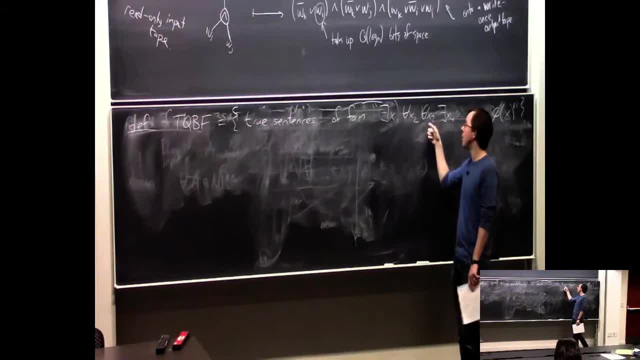 such that, no matter how x2 is set to 0 or 1, and no matter how x3 is set to 0 or 1,, there is a way to set x4 to be 0 or 1, blah, blah, blah, blah. 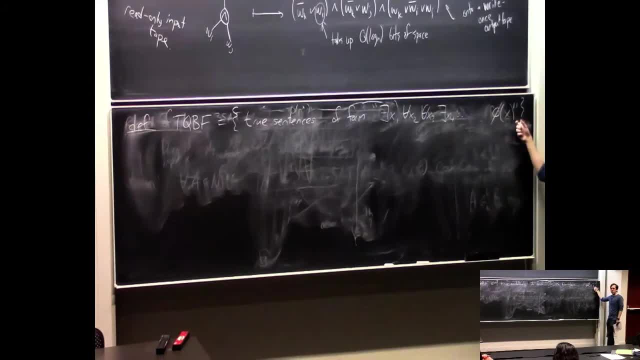 all the way out to xn, such that this propositional formula becomes true. By the way, it's usual to write q for a quantifier where it can stand for for all or exists. So really I should say here each q1, x1,, q2, x2,, et cetera. 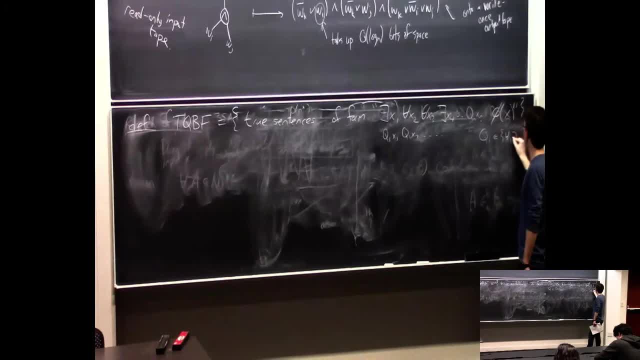 where each qi is either for all or there exists. OK, is the definition OK? So the first thing we're going to do is think about algorithms for this problem. And you see, this problem is at least as hard as SAT because, in particular, you could just use all there exists. 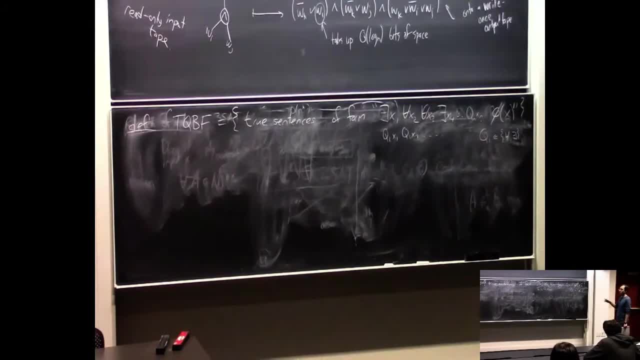 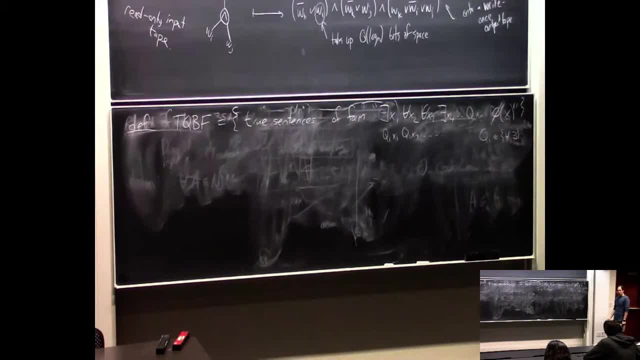 I don't care, that solves this problem. you could do it Right. I mean you could- basically you'd have to actually take a little care in how to write it down, But you can sort of tell that if you tried all possibilities. 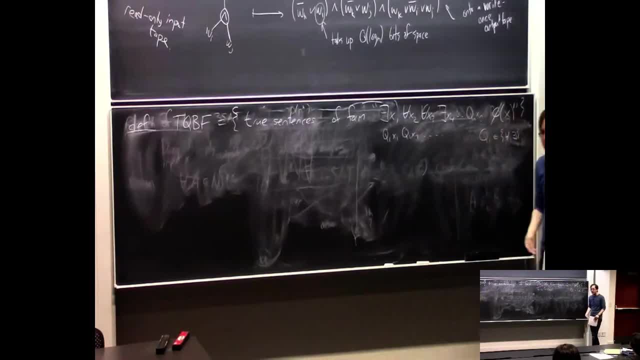 for x1 and tried all possibilities for x2 and all possibilities for x3, and then in each case evaluated whether phi of x was true or not. you would have all the information you would need to decide if the whole thing is true. It would still be a little bit complicated, right. 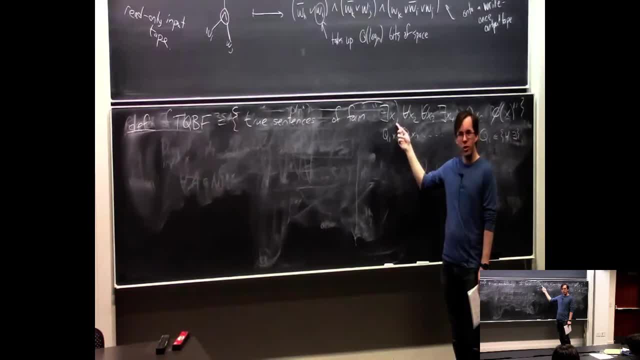 Because you have to do sort of like an implicit or over the two choices for x1 and then kind of an and over the two choices for x2.. But you could imagine doing it. So let me just say it's an exercise for you. 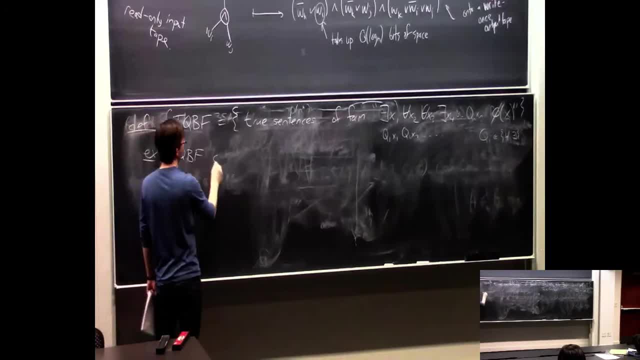 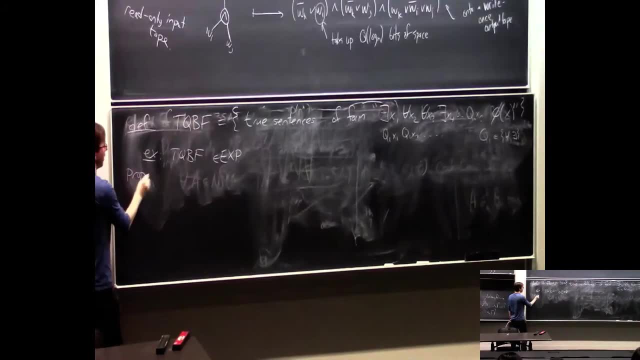 to think about why this problem is in exponential time. Well, you probably may as well not do that exercise, because that'll show an even stronger result that it's in p-space. So the first thing I wanted to do is show you that in fact, you can solve. 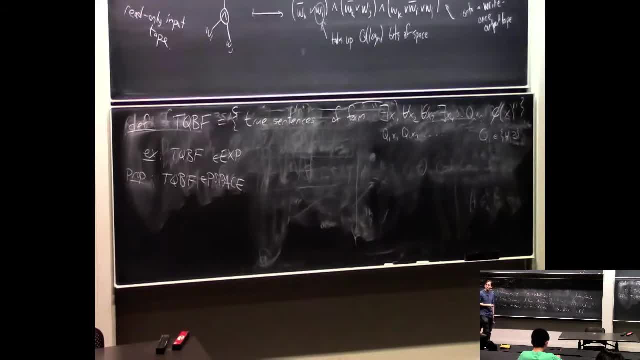 this problem in polynomial space, OK, and in fact this algorithm for solving in polynomial space. sometimes we've seen some algorithms that when we tried to show something was in a space-mounted class. they felt a little bit stupid, Like they really worked hard to use a limited amount of space. 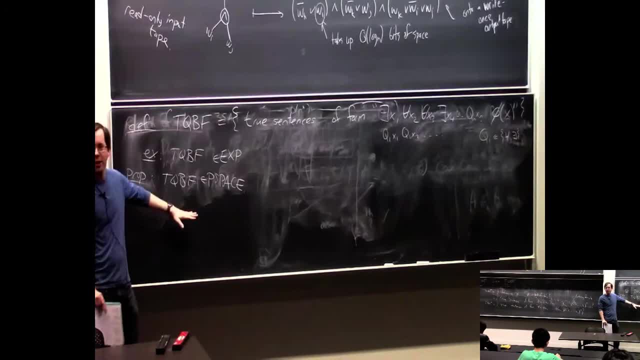 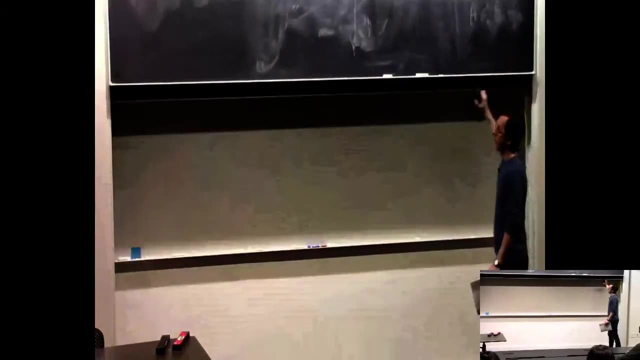 and they did some silly things in terms of time. Actually, that will not be the case here. This will be like a quite reasonable algorithm that you might literally imagine using for this problem. OK, so let me prove that theorem And I'll just write the algorithm. 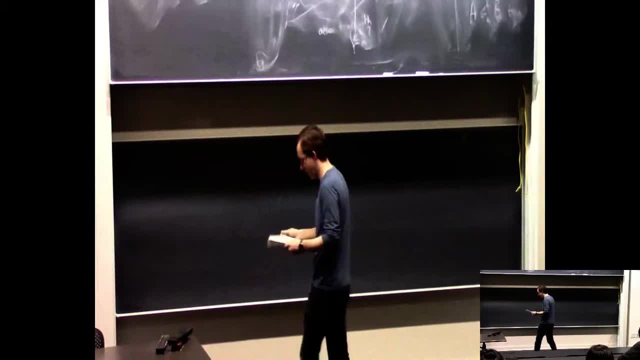 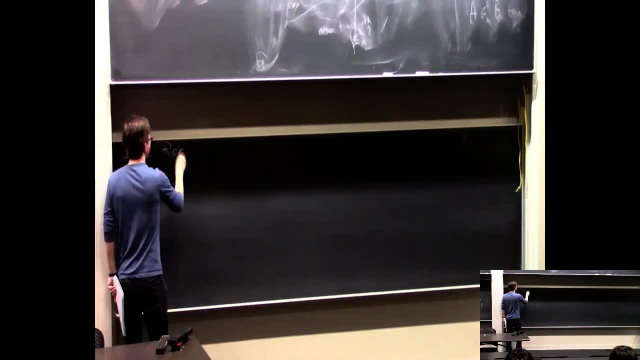 And it's kind of well. it's like an algorithm we've seen before and it's kind of a natural one. So the idea is to do a recursive algorithm And it's kind of well, it's like a very simple algorithm. 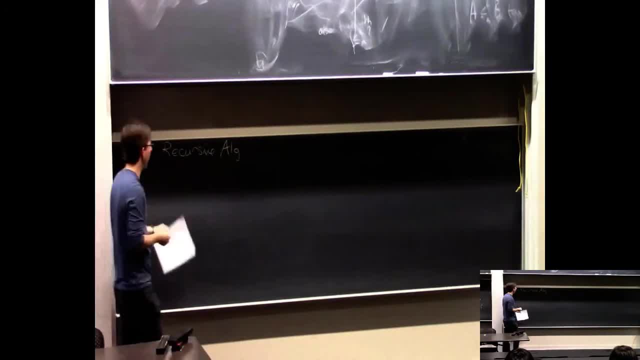 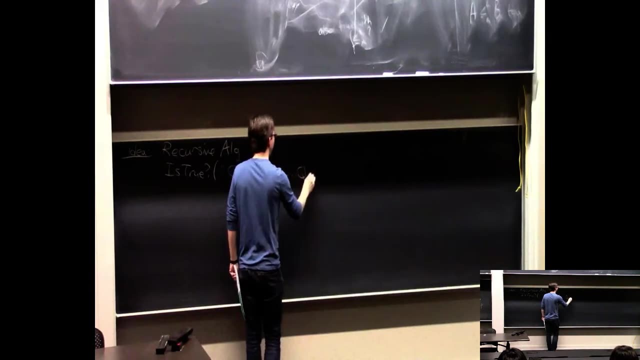 And it's kind of well. it's like a very simple algorithm, OK, and we'll just describe it as is true, and it takes as inputs a sentence that looks like this: Q1, x1,, Q2, x2,, et cetera, Qn, xn, phi of x1 through xn. OK, so we're trying to write, I mean, and then we'll do this. It's just a little bit complicated, but it's all right. It's just a little bit complicated, So we're trying to write, And then we'll do it. 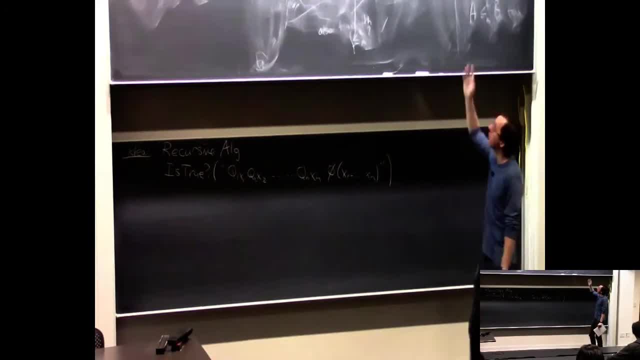 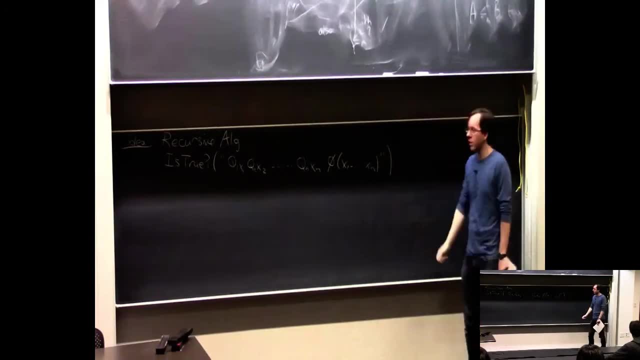 And then we'll do it. So once we have this thing, we'll just. that solves TQBF, OK, and the kind of recursion parameter is going to be n, the number of variables. So let me, before I begin, normally in Boolean formulas: 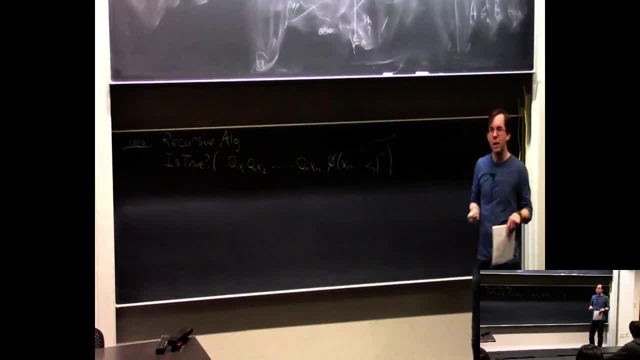 this is a technical point, but normally in Boolean formulas you're just allowed to have variable names, and and and or and not, and I don't know, maybe implies Let's just say we're also going to allow constants. 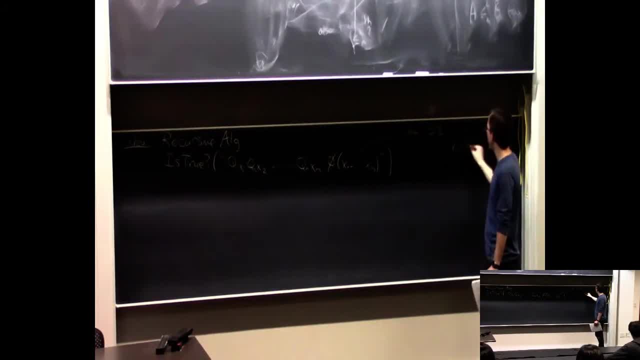 OK, so a formula you know. normally it looks like x1 or x2, and x3 maybe implies x2.. Let me just say our algorithm's even going to be able to handle like if you have a 0, like plugged in. 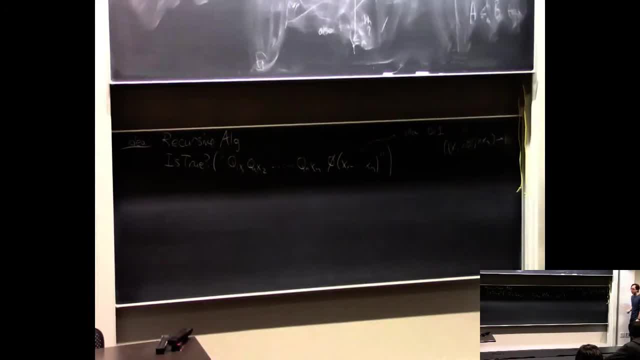 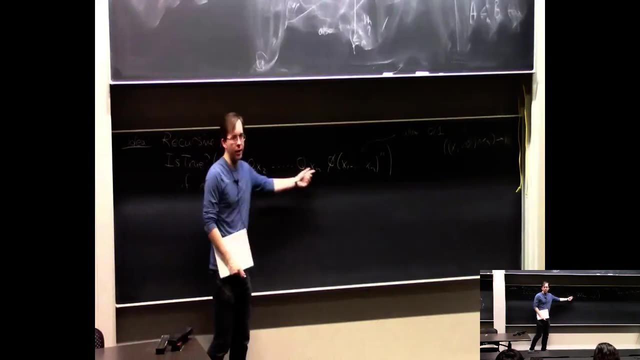 OK, or if, like you, have like a 1 unplugged in, That's going to be fine. OK, so it's a natural algorithm. The base case for the recursion is going to be n equals 0. So if there are no quantifiers and no variables, 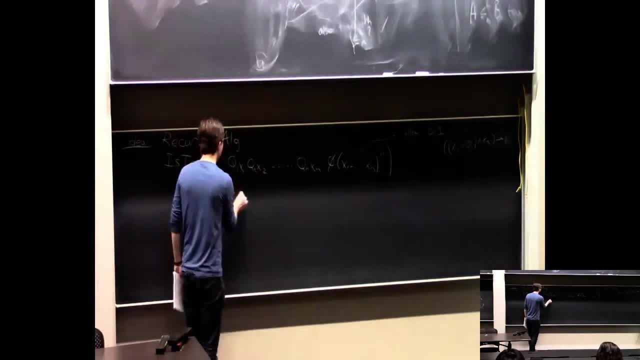 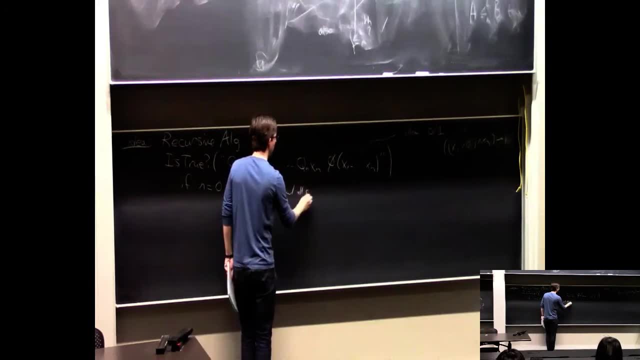 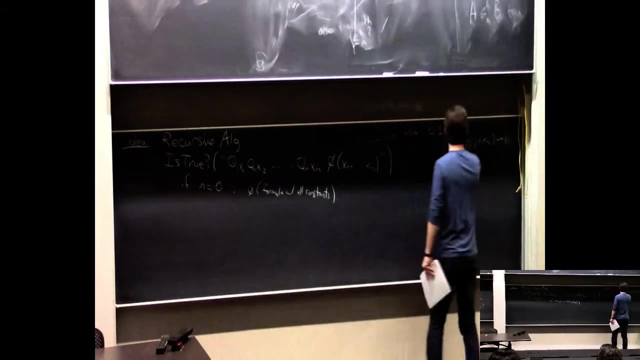 then really you just have phi as just like a formula with all constants in it. You know, some formula looks like this, but like literally everything has been replaced by a constant. OK, and you can certainly like easily evaluate whether 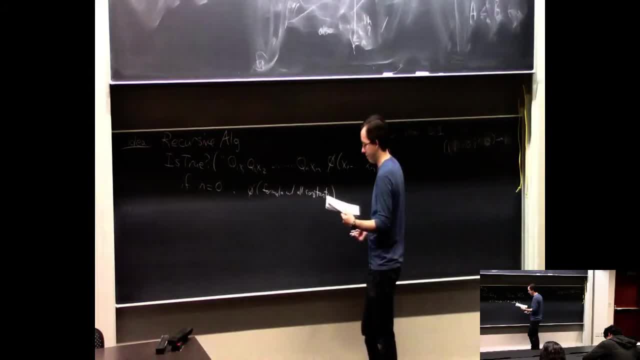 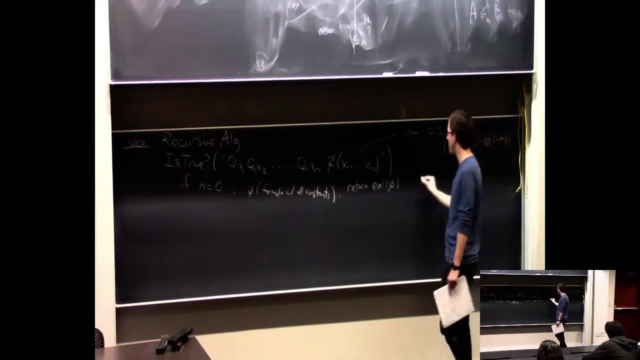 that formula is true or not. OK, so just you know. return the evaluation. OK, so this is the equation of phi, And this you can do in logarithmic space. actually, I mean, you hardly have to do anything, but this is very easy. 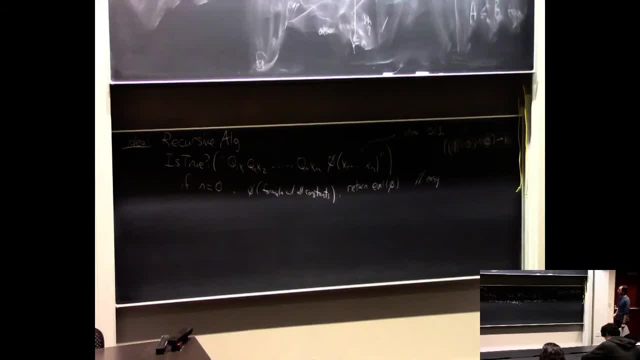 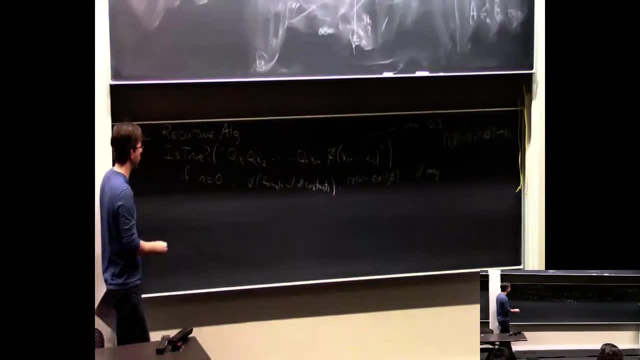 OK, and we'll come to the actual space complexity later, but this is certainly an easy part. OK, otherwise, you have at least one quantifier and what we're going to do is just try everything for the first quantifier, So else, 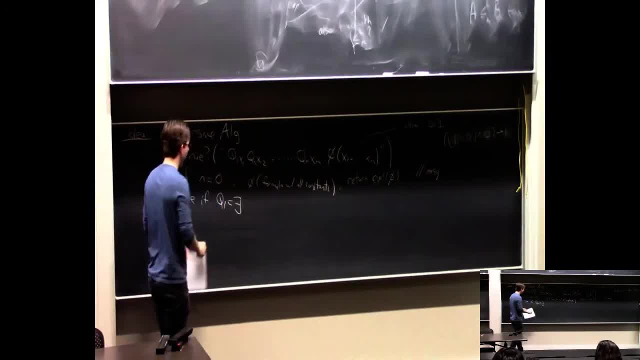 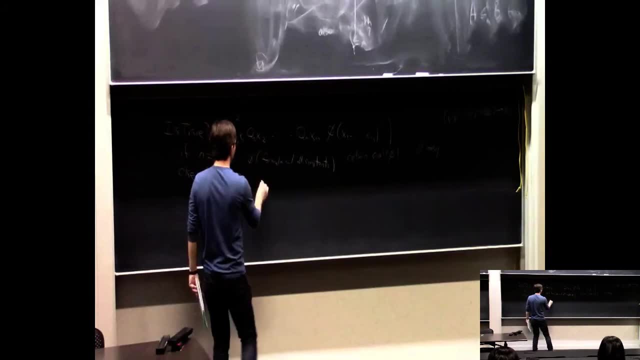 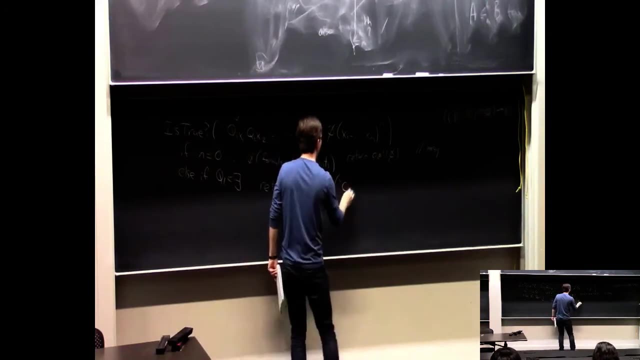 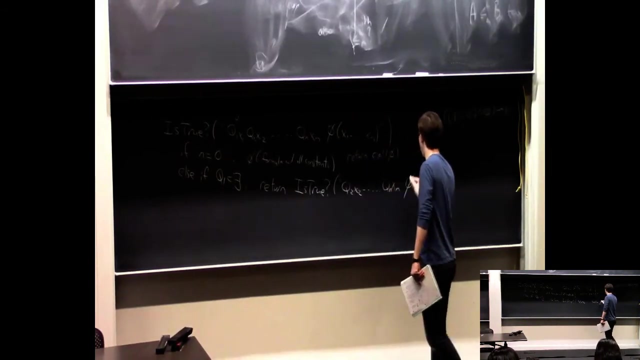 OK, If q1 is 0.. If q1 is there, exists, well, what will we do? Well, I think the correct thing to do is natural. You just return. recursively is true function applied to everything starting from the second quantifier. 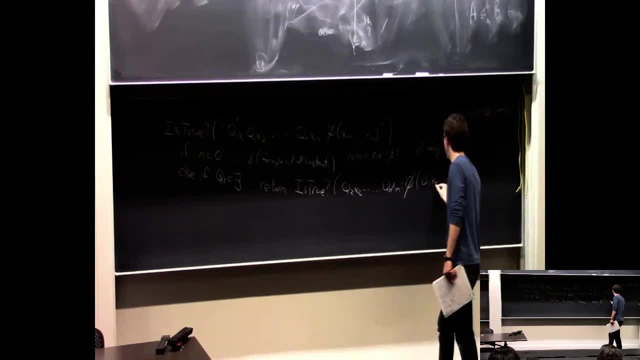 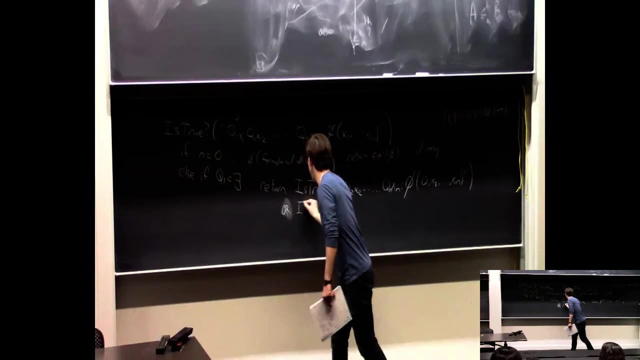 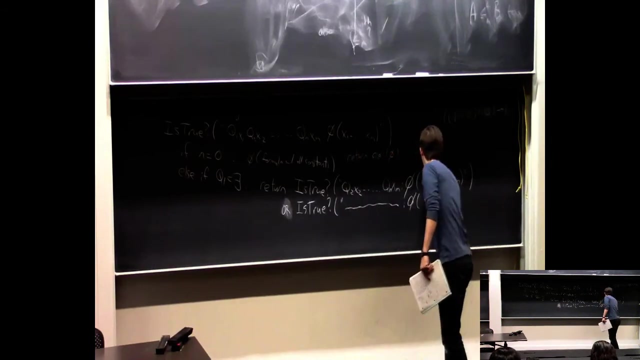 and then phi, with 0 plugged in for x1. So you recursively determine if this is true And then you also recursively rewrite it in words, or the same thing where you plug in 1 for the first variable. OK, and that's correct, right. 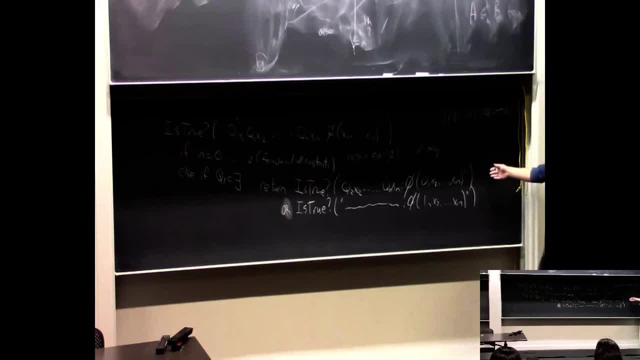 I mean, the whole thing exists at the front. It exists x1, such that this function exists in the first Right. OK, OK. further quantified sentence is true. that holds if, and only if, one of the things you get when you plug in x1 to be 0 or 1 is true, And let me not really write it, but the final: 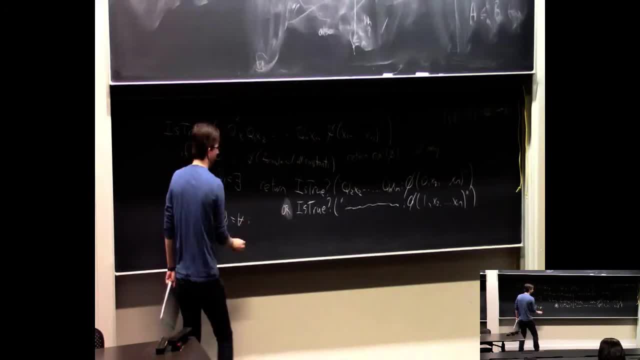 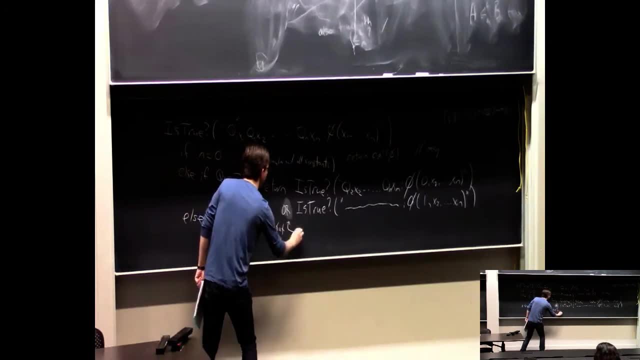 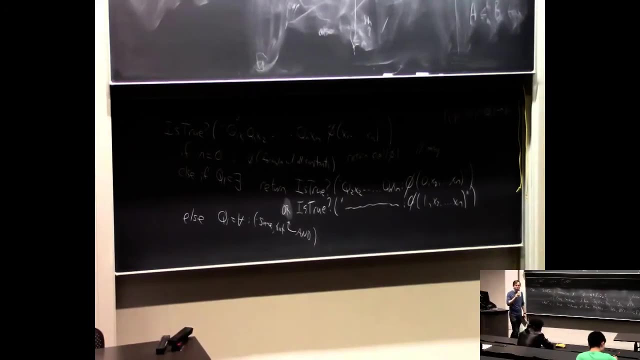 possibility is that q1 is for all, And then let me just say: it's the same thing, but this would become and OK, so I claim this is a correct algorithm for TQBF. Any problems with it? Last time I wrote down like a simple algorithm and just said this is clearly correct. 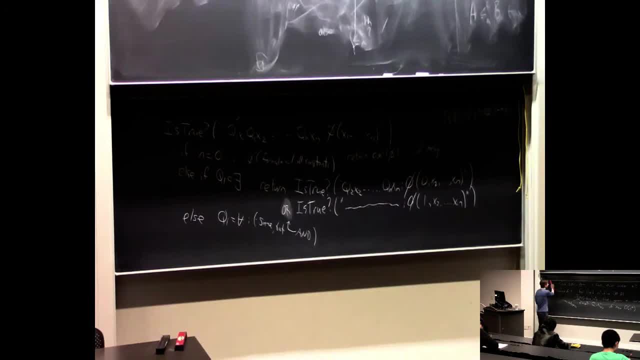 It turned out to be wrong in two places, So it's not like an idle question. I mean, does it look correct? I think it's correct. OK, no objections? All right, it's correct, Great, OK. so space complexity. 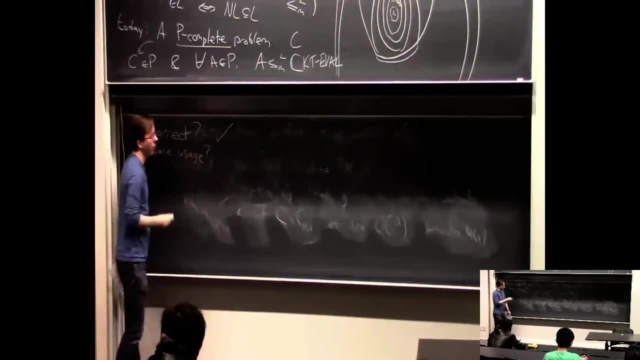 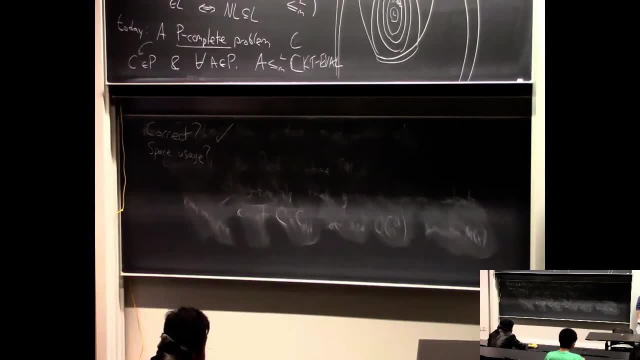 OK, now we have to think a little bit about how much space you use. Oh, I forgot to mention it before, but there's kind of two parameters that you care about here: N, the number of variables, and the literal input size, like literally the number of bits you need to encode. 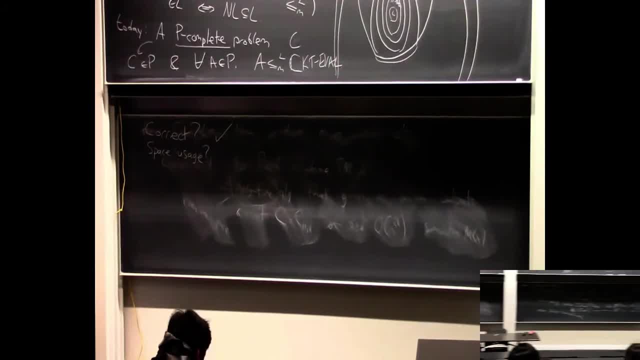 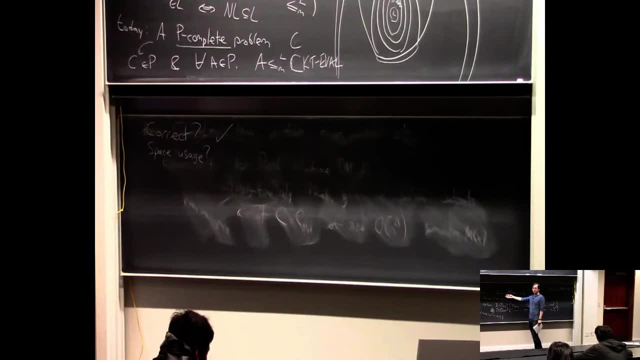 the whole sentence, which maybe you would call m, And you really only have to run in polynomial in m space. That's the definition of polynomial space And, just as an observation, OK n. the number of variables is always bounded above by m, because it takes at least one. 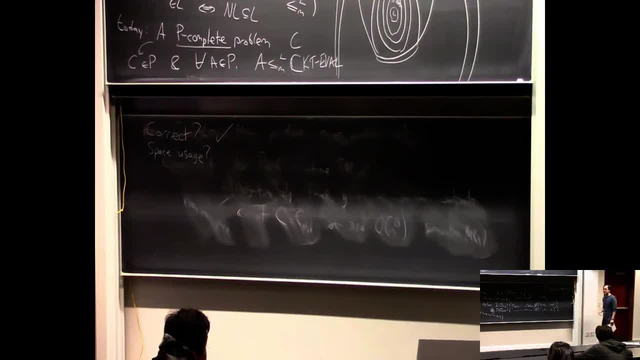 bit to mention any variable. So we're actually going to analyze the space complexity in terms of n, the number of variables, and maybe m, the actual literal size of the strings we're dealing with, And at the end we can just remember that n is at most m. 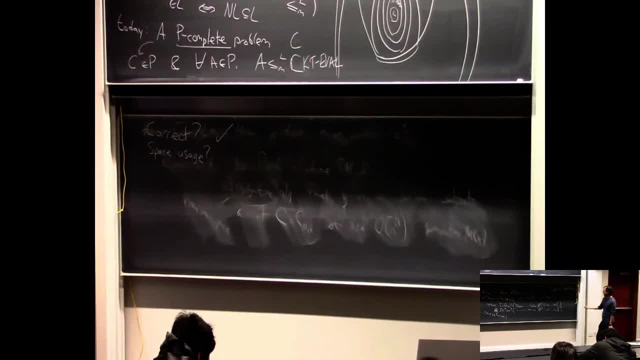 So if you just look at this code here, I mean it looks like it uses hardly any space, like this, I mean it doesn't seem to use a lot of space, It just needs to, let's say, write this whole sentence down on its tape. Let's say it's linear space And it kind of needs. 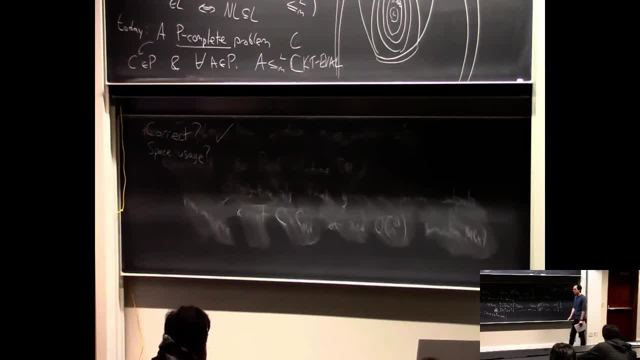 to do that because, I don't know, it has to replace some things with 0s and 1s, But of course you have to account for the recursion. I mean, it doesn't happen by magic. You have to imagine how it's done on a Turing machine. 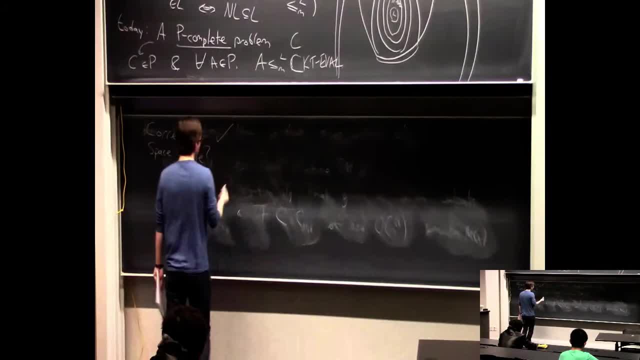 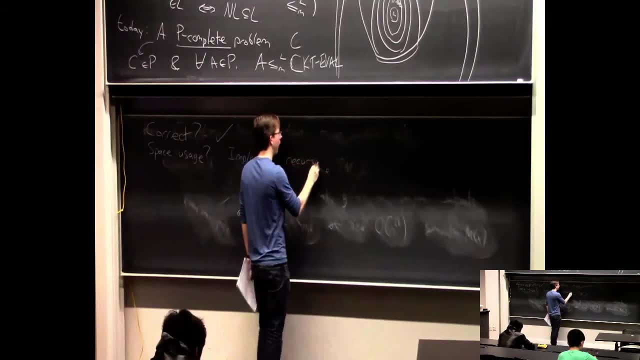 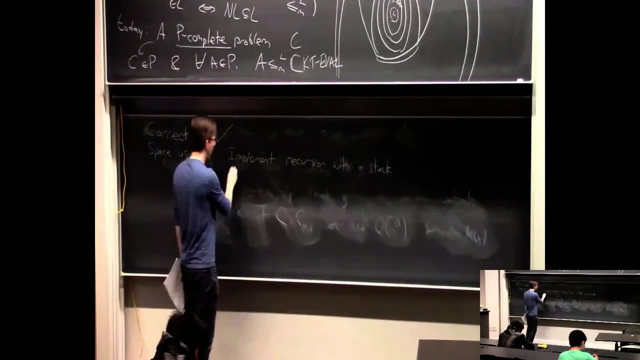 But we talked about this when we studied Savage's theorem. right, So you're going to implement the recursion with a stack And the depth of the recursion, well, it's n. I mean every time you do a recursive call. 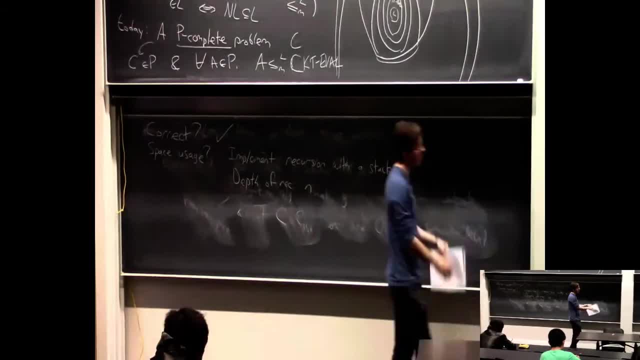 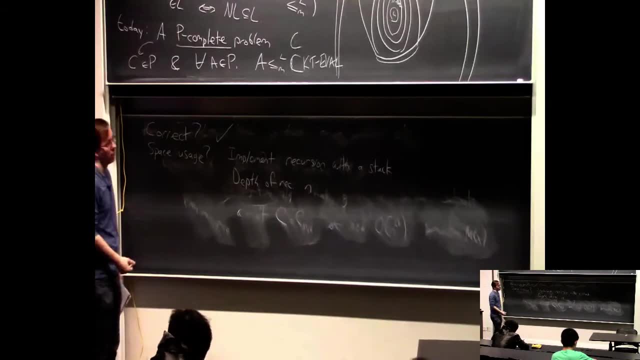 you get rid of one variable. So each call potentially has two branches. So the depth of the recursion is n, The total number of things you might be computing recursively is 2 to the n And of course, when you implement your recursion you're going to reuse space, You're going 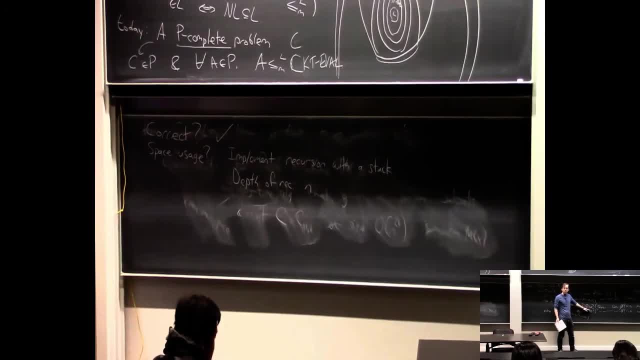 to do this recursive call on some amount of tape And then when you pop back up and come to do the next recursive call, you're going to use that same workspace to implement this call. You're not going to liberally just use new space every time you need to do a new. amount of work. 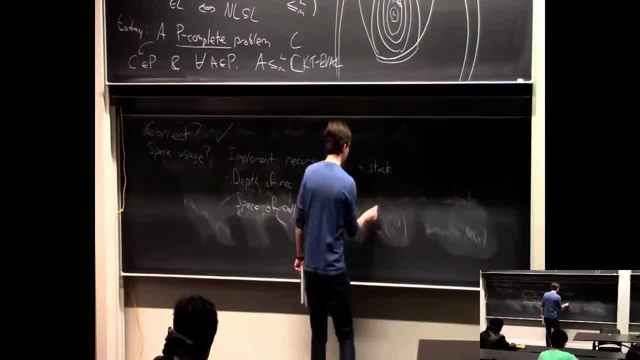 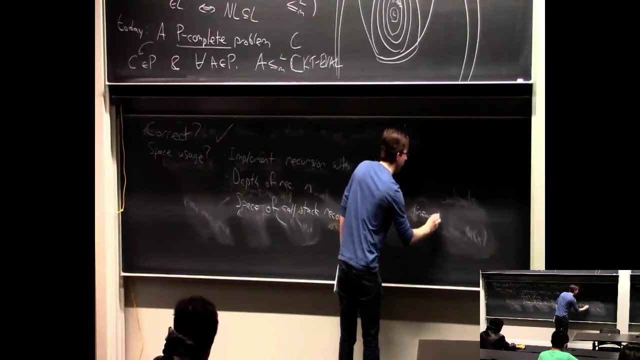 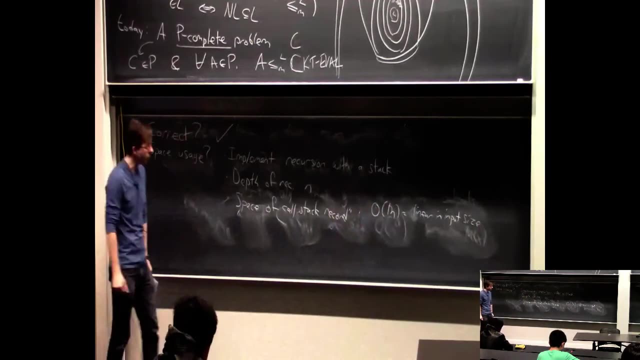 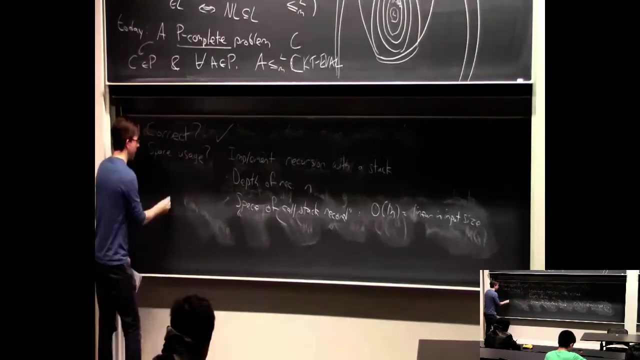 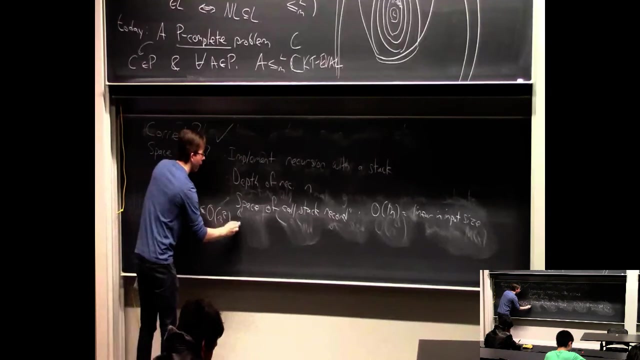 plausible at least. yeah, actually, if you're a bit clever, you can do the whole. 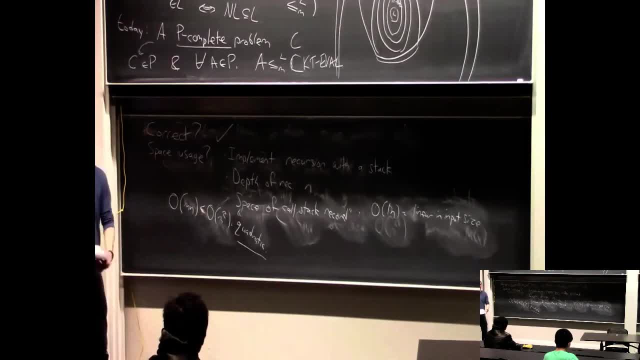 thing in linear space, but don't really care. I mean, polynomial space is good enough for me, great, so okay, so we've shown that you can solve this problem in polynomial space. and it also takes exponential time because in the worst case you might actually have to do all sort of 2 to the n recursive calls. 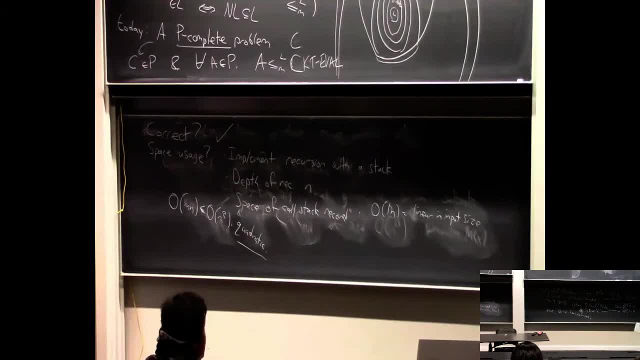 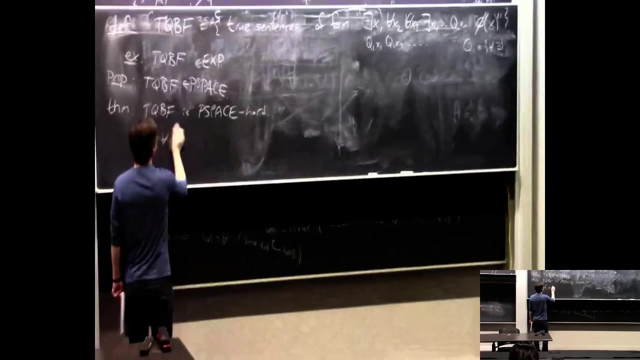 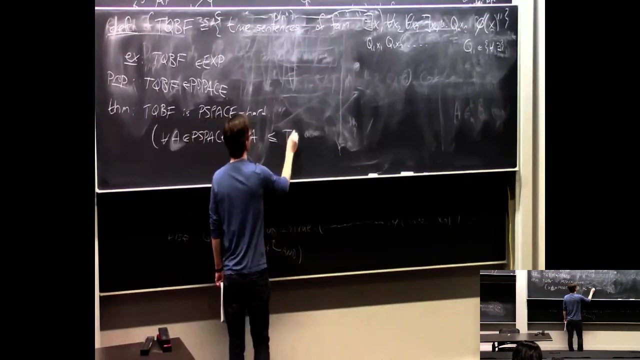 that's life, all right. so the the thing that we want to now show, eventually, is it's piece based hard. what does that mean, you know? for all? al, well, let me say a in pieceACE, a reduced to a for all these values. And now here, actually, we have a choice. 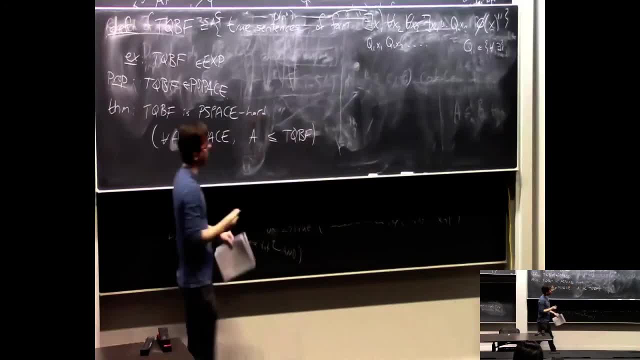 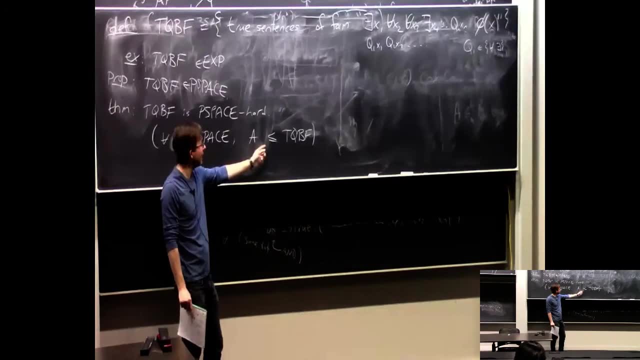 I mean, what do we mean by this? Do we want to put in polynomial time or do we want to put in linear space? And for this case I basically say: I don't care that much, Because if you're studying PSPACE, 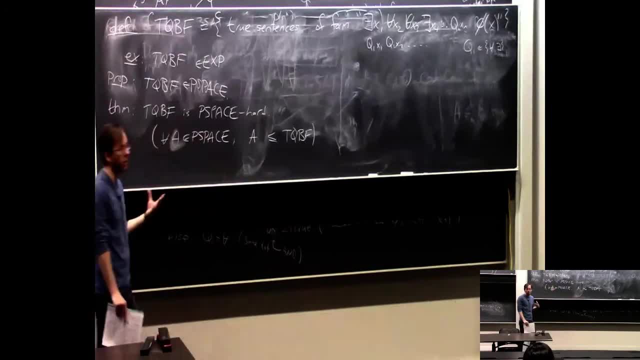 probably polynomial time reductions are fine. You're probably trying to reason about whether some PSPACE problems that you know in PSPACE could actually be in P or something. So polynomial time is fine. You're probably not trying to reason about whether this PSPACE-hard problem is in L, because we have the space. 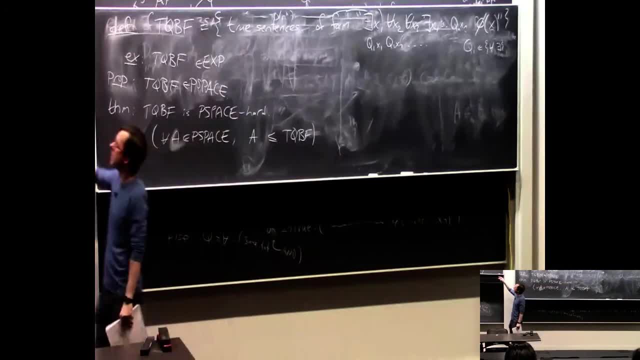 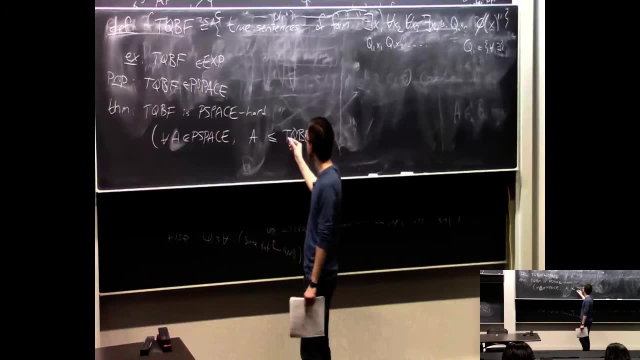 hierarchy theorem. So we know that there are problems in PSPACE that are not in L. I mean, as it happens, if you decide to care and you believe this empirical fact, it actually is in L, log space reduction. I'm not even going to really bother to care about it. 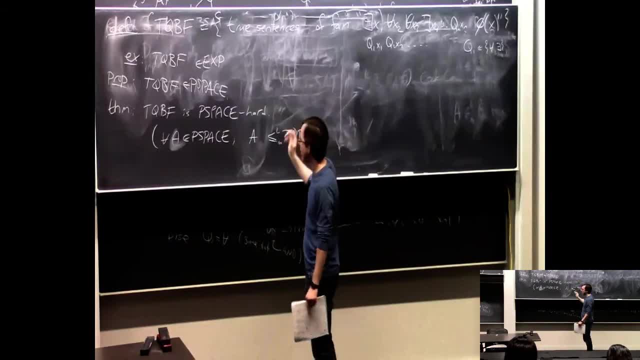 So it's going to be a simple reduction when you see it. So let me just write P. But if you want, you can think a bit more carefully and verify for yourself. So let me just write P And you can think of yourself as even in log space. 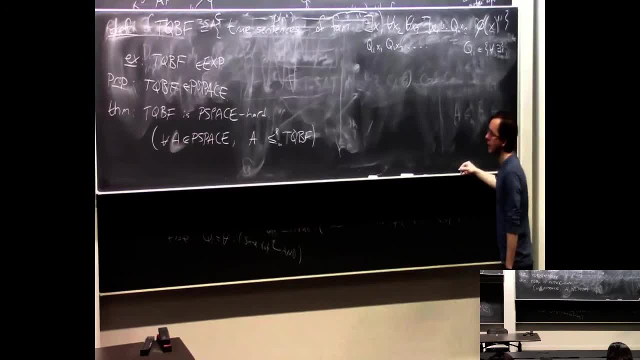 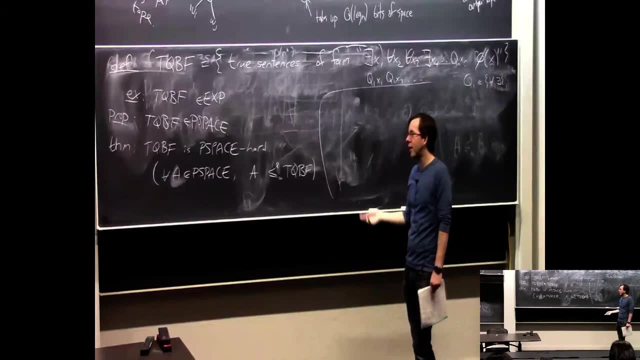 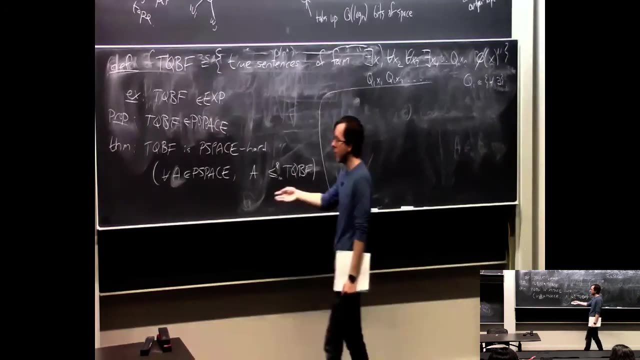 the reduction, OK. And you see, this is kind of going to have a flavor of like a Cook-Levin-type theorem again, something about computational tableaus or configurations or whatnot, Because I mean it's a theorem like this. 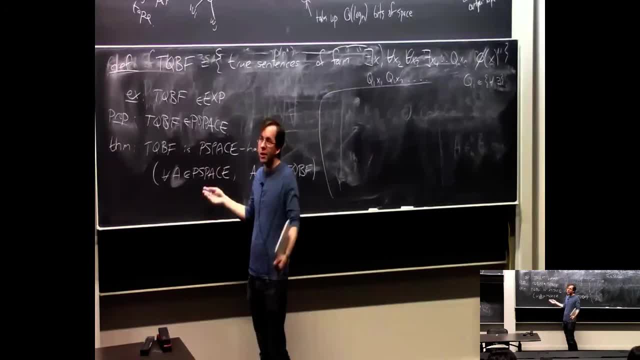 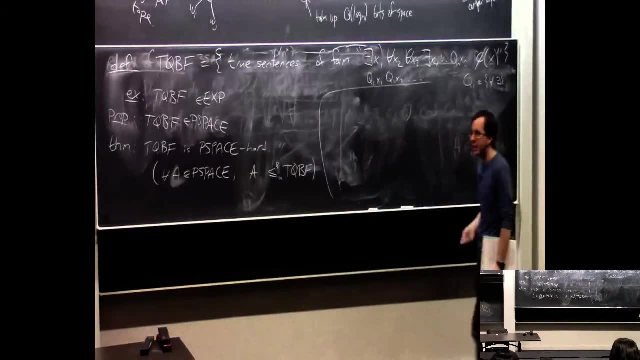 You have to take any old language at all in polynomial space. So basically all that you know about it is there's a polynomial space Turing machine that decides it And you have to convert it to a TQBF problem. So you have to somehow really write down. 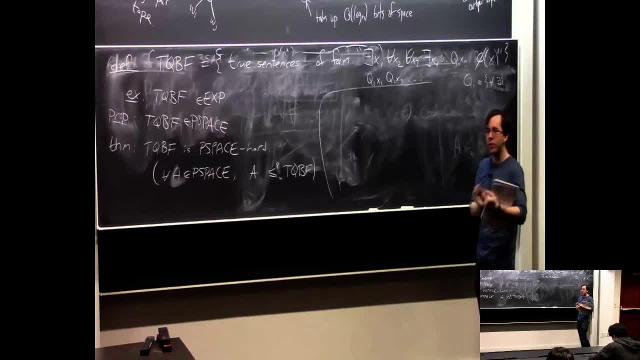 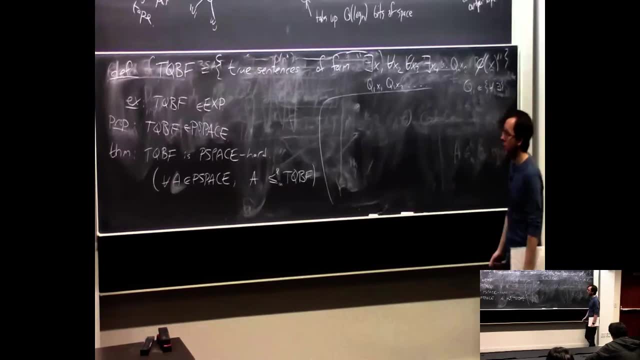 a quantified Boolean formula. that's true if, and only if, a certain Turing machine accepts, And the proof as we'll see. it's kind of like some kind of glorious combination of- like Cook-Levin ideas and the L-nail completeness of path. 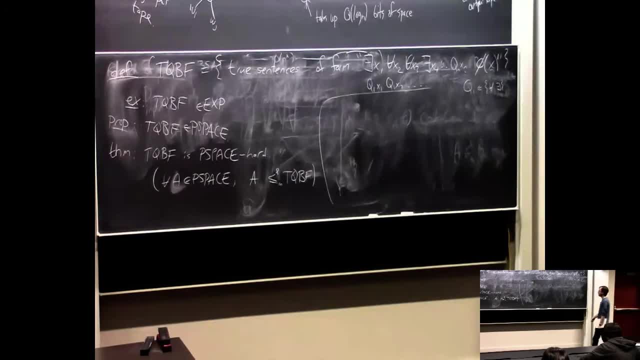 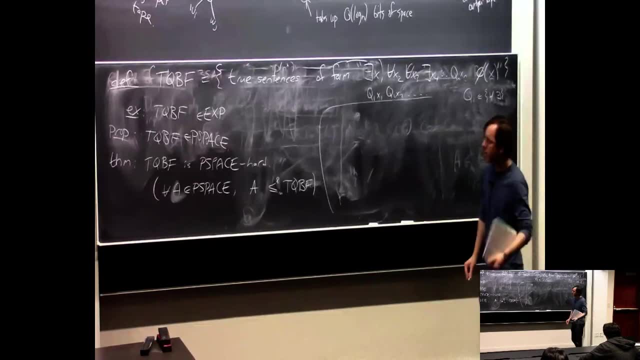 and Savage's theorem all gloriously rolled into one. OK, Actually, just before we get to it- I think I have time to do it like this- Let me say a couple of things about TQBF. This will just be a brief statement. 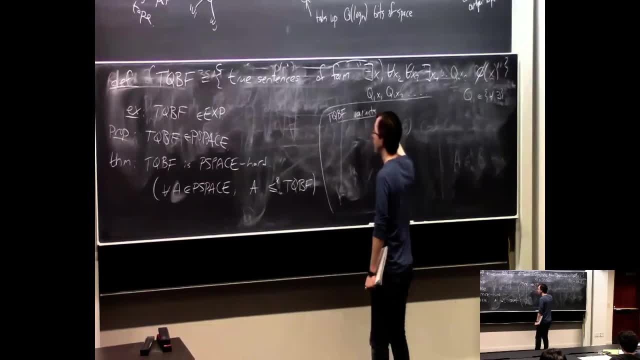 about variance of TQBF. Much like there are many variants of SATs- you know, there's 3SAT and whatever- there's variance also of TQBF And it's a fact which I don't really want to get into, that they're all. 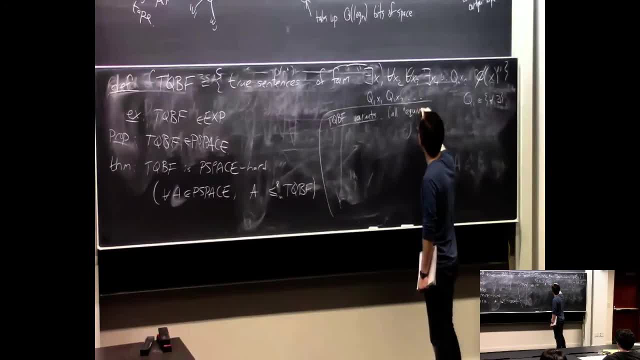 you know, equivalent, And at a high level. what do I mean by equivalent? I mean they're kind of equally hard or easy. Given an instance of this variant, you can easily transform it into an instance of the classic variant, If you really wanted me to pin down what I meant by that. 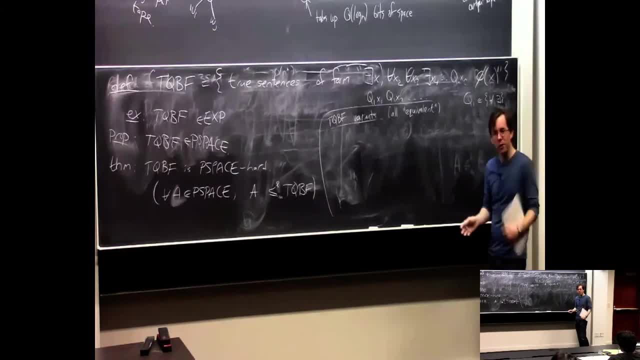 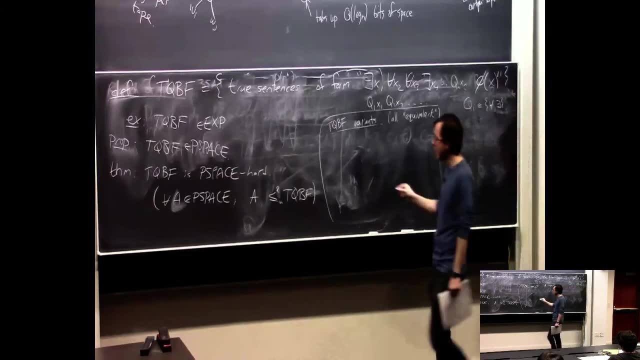 I would say that they're all like log space reducible to each other, or polynomial time reducible to each other, But I think you'll get the picture when I just say what I'm talking about here. For example, one variant of TQBF that's. 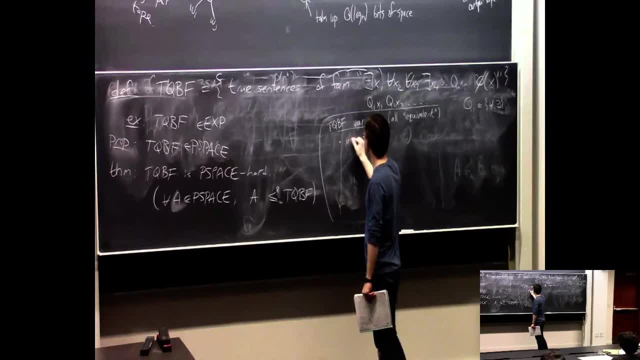 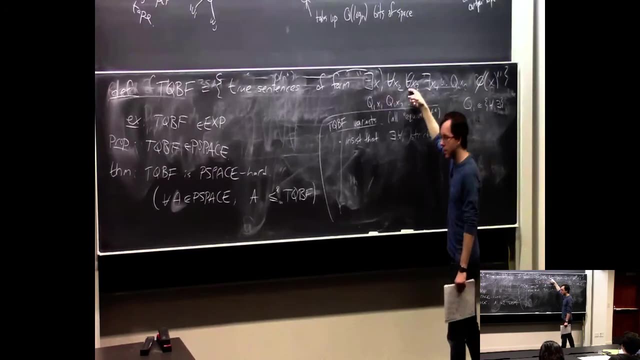 equivalent is like you can insist that the quantifiers that exist for all strictly alternate, So that you're not allowed to have this. It has to be: there exists x1 for all x2,, there exists x3 for all x4, et cetera. 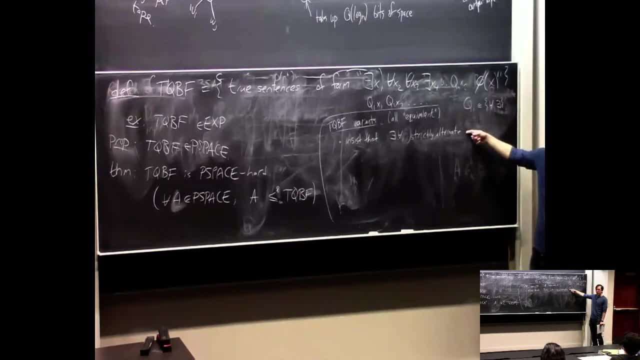 So this is actually like a special case of TQBF, the case where, like all the quantifiers have to alternate. But I just want to tell you it's not especially it's not an easier special case, Really, Because if you want to get that, 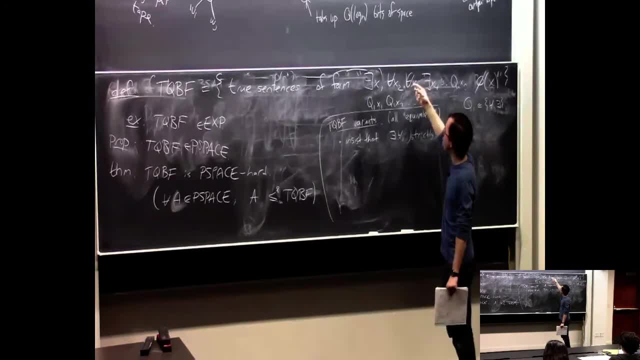 you can just artificially insert dummy variables. You can just here, you can say: oh, there exists x2.5.. And then just like, never mention x2.5 here, So it has the same satisfiability status because the phi doesn't care about this x2.5. 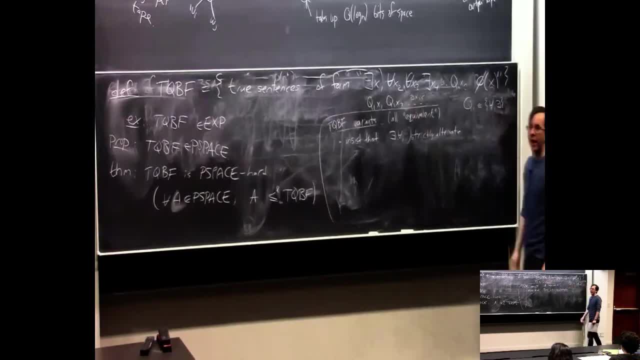 You artificially made it start to alternate And the most number of dummy variables you'll have to add is n more. So maybe you'll go from n variables to 2n variables. That's hardly a big problem. So like you know this, I guess technically I should say: 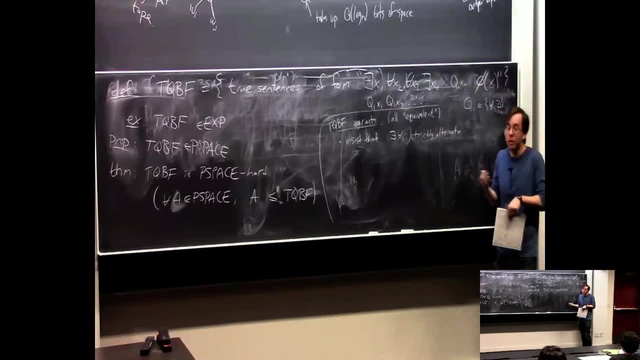 this reduction where you insert dummy variables, can be carried. it's like really a reduction that can be carried out in polynomial time or log space or whatever. But I think you get the gist that it's a simple equivalent problem. So that's a special case which is still equivalent. 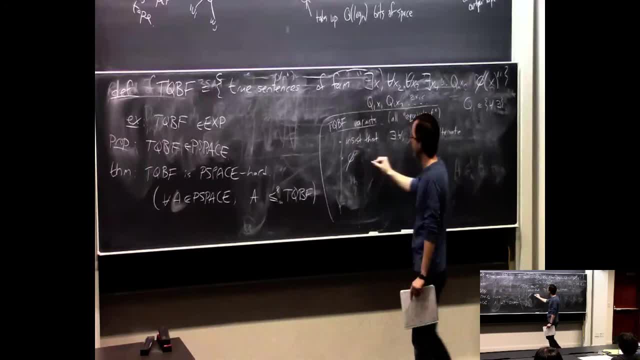 You know there's also slight variance about what you allow in phi, Like on one hand you can be like more liberal and you can allow. you know some people will just say, oh, you only get and or and not. 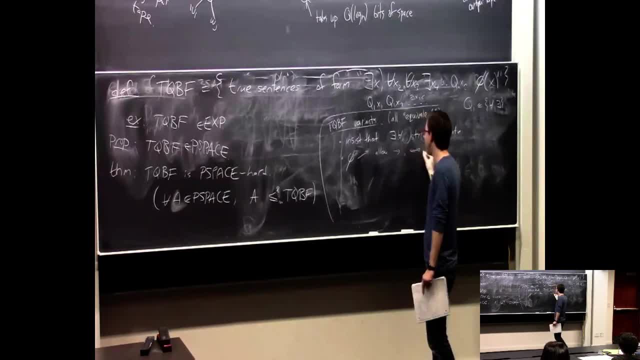 But you know you can also allow implies or if and only if, or you know whatever, Or you can also insist. so this makes it technically more general, but not really, because we know you can convert this to ands and ors and nots. 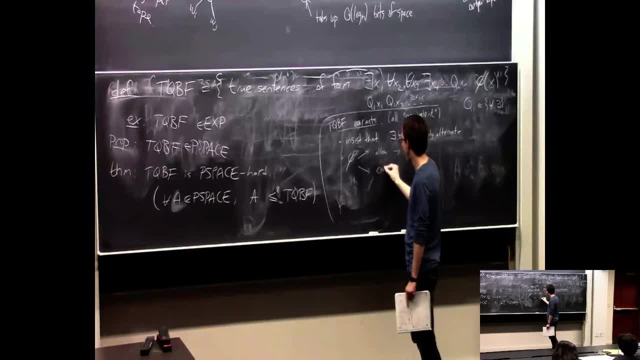 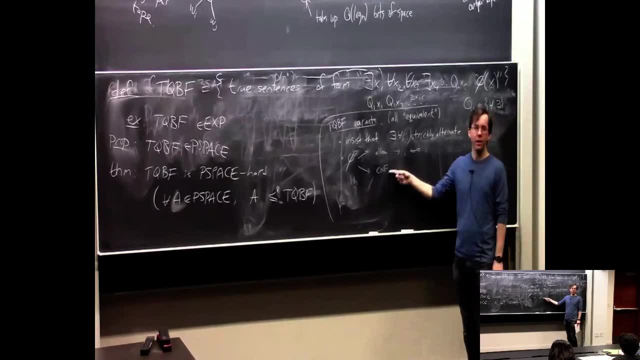 You can also insist that it's phi is a CNF. That's a special case. It takes a tiny bit of thought to realize that it's actually not any easier when phi is a CNF. But I won't even really use that fact. 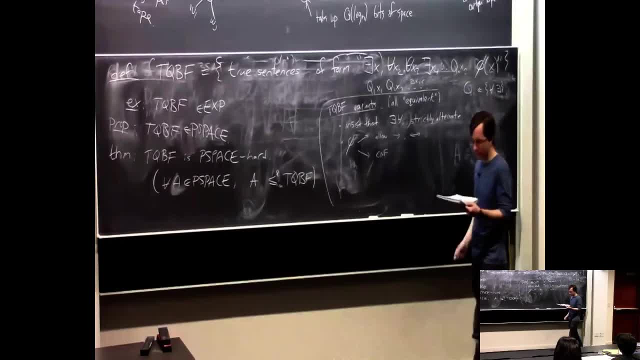 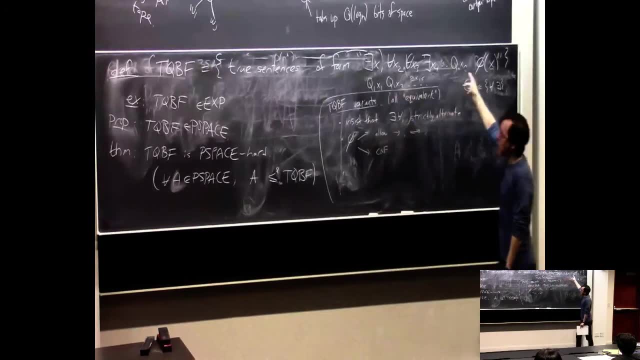 I just wanted to tell it to you that it's not really any easier if phi has to be a CNF. This one is a little bit important to mention. You see the sentences I talked about in TQBF. in our original definition they have all the quantifiers. 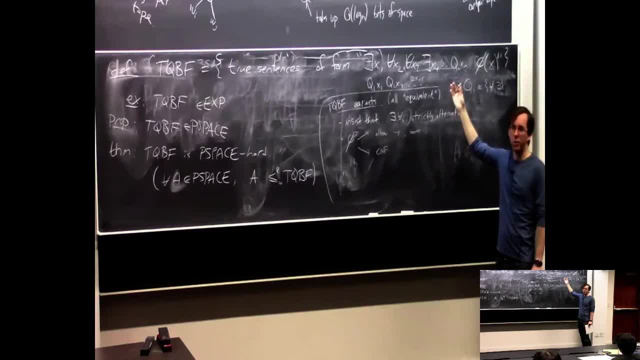 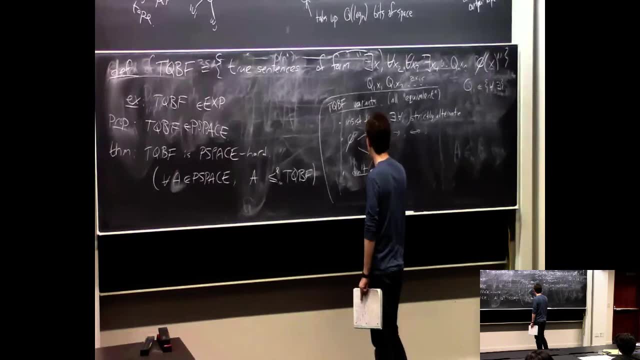 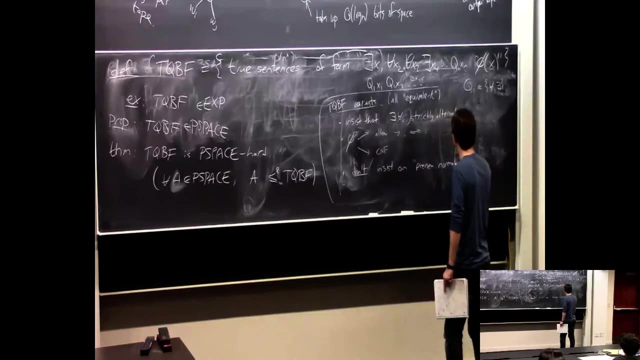 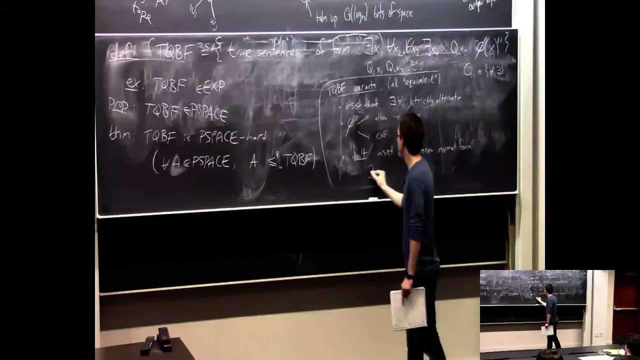 at the front. This is called pre-next normal form by logicians And it's equivalent, even if you don't insist on that. Okay, so you could imagine a variant of TQBF where you're allowed to do things like: oh, there exists x1, such that for all x2,. 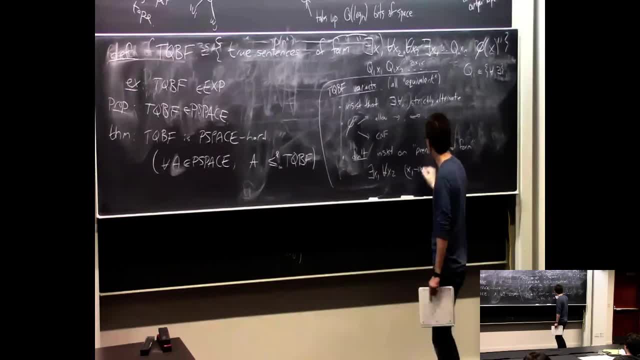 you know x1 implies x2, and there exists x3, such that you know x3, or I don't know there exists x4, such that blah, blah blah. So you have, like the exists and the for alls. 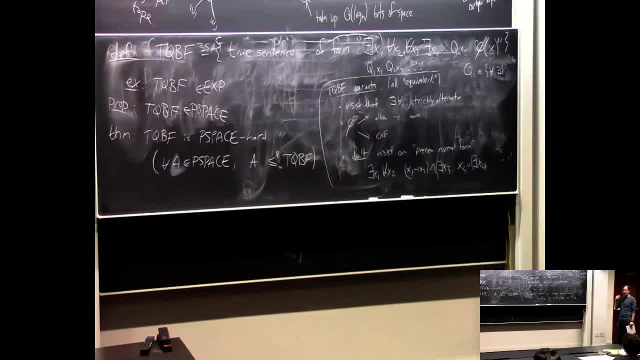 like strewn in the inside of the formula as well. Okay, Maybe you have like negations in here and stuff. Let me say, suffice it to say, even though that's a more general looking problem, it's like well known in like logic and computer science. 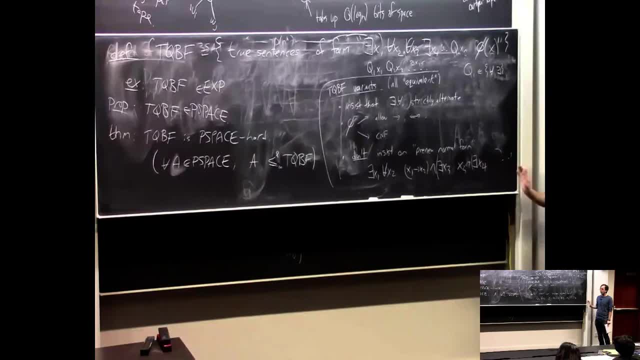 that you can easily convert it to an equivalent formula that has all the quantifiers at the front. So you can look this up on Wikipedia if you want. or it's the same as showing that if you have like a circuit, you can move all the not gates to the bottom. 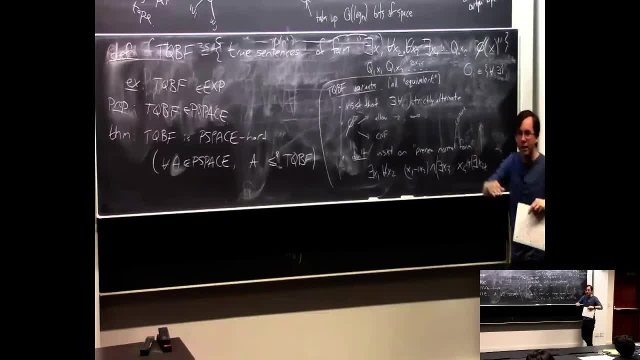 and you can assume that, like all the not gates and all the ors and and gates alternate. That's like the same fact. But you can convert anything that has for alls and exists in the middle to pre-next normal form by using rules like there exists not. 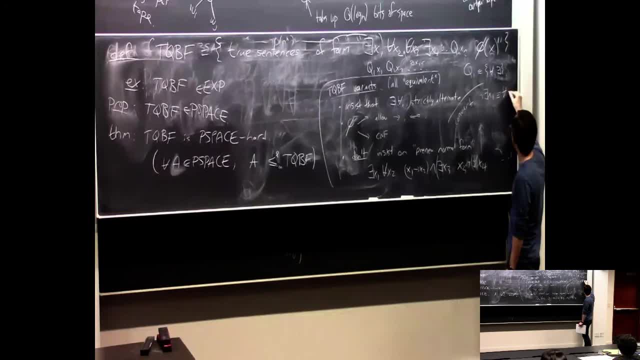 there exists, x1 is the same as for all x1 of phi, not phi. you know that's De Morgan's law, So that you know, gets the nots to the inside and the quantifier to the outside. And if you have things like you know, 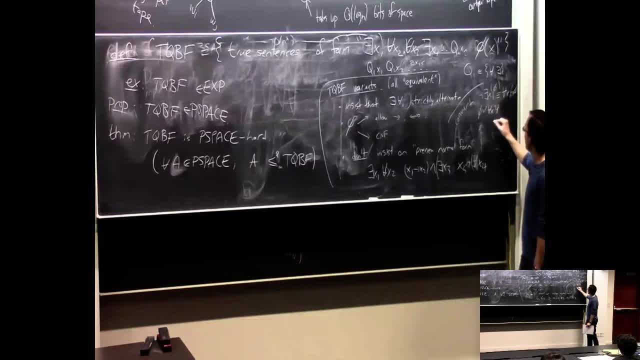 for all psi and for all x psi, that's equivalent to for all x, or this should be an- and I don't know- phi and psi. Okay, let me turn this into a logic class. Suffice it to say there's an easy transformation. 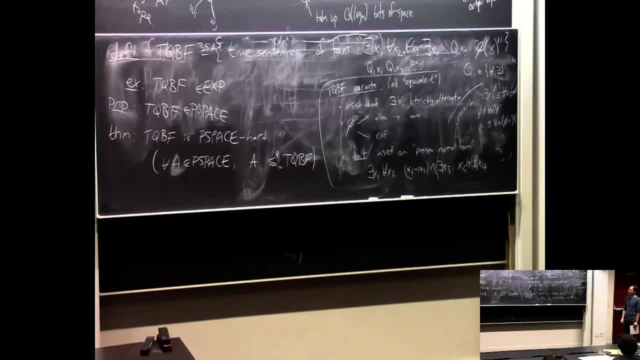 that moves all the quantifiers to the outside, And this one I bring up because I'm going to show you this reduction that takes reduces any problem in p space to an instance of TQBF And the quantified SAT formulas that this reduction 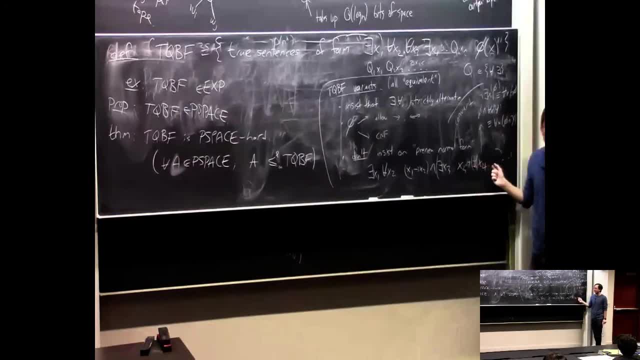 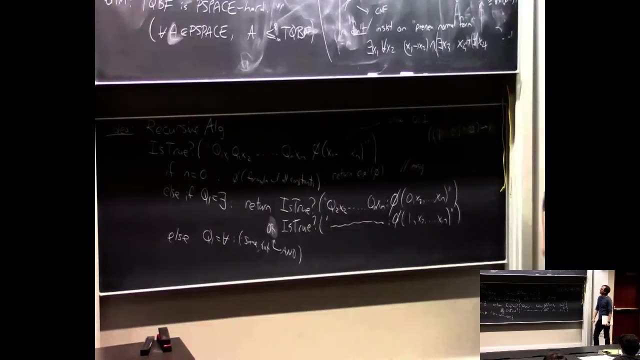 will produce will actually have quantifiers on the inside, like not all on the outside. So I'm just warning you now you can also easily stick on some stuff at the end that moves them to the outside. Okay, any questions about TQBF? 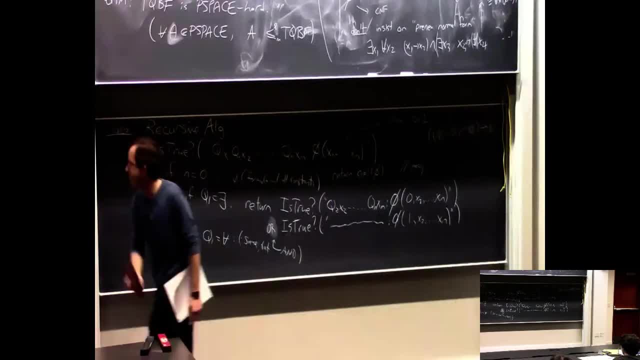 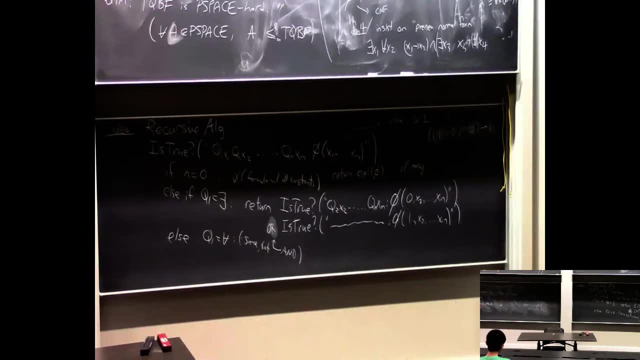 Okay, it's quite a technical lecture today. You know a lot of Cook-Levin stuff which is very technical, but we'll have a very satisfying picture at the end. Okay, so now I'm going to prove that TQBF is p space hard. 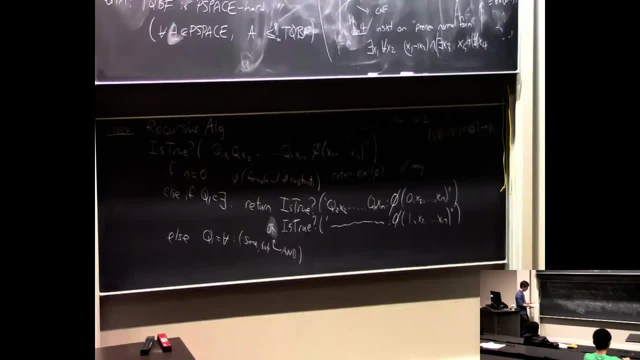 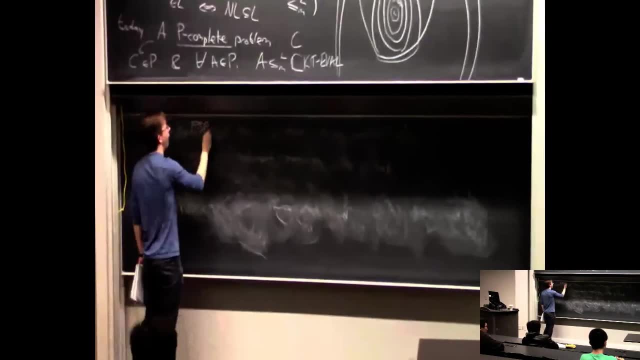 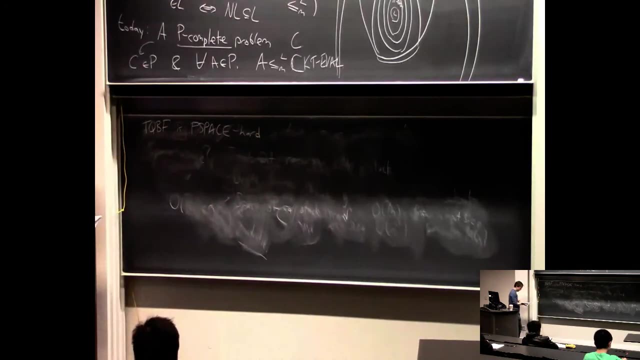 In the last. ooh, see how it goes. Don't have too much time left Now. I'm not going to finish this in time. Let me sketch the idea and then we'll finish it at the beginning of the next lecture. So what is the idea? 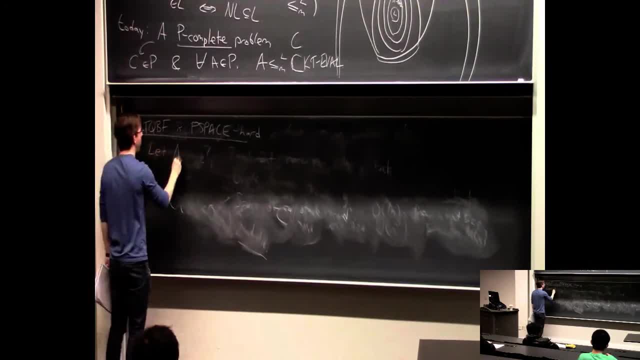 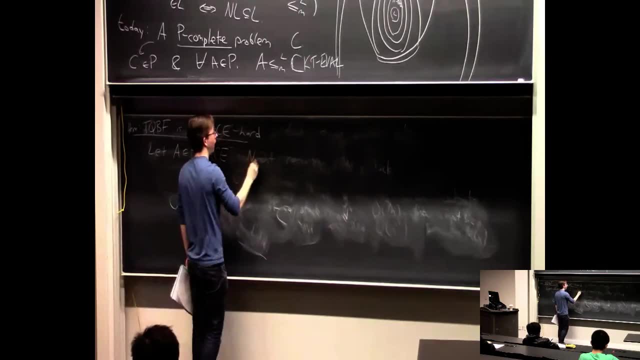 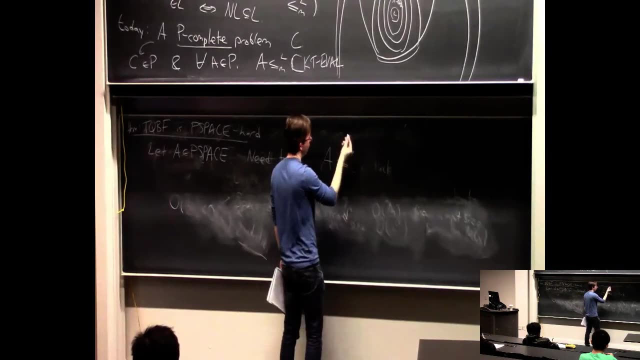 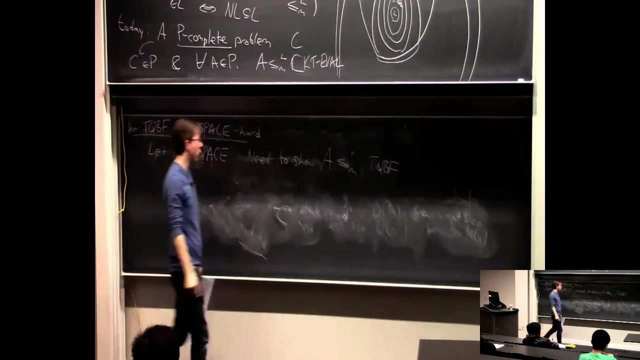 Okay, we have to prove this theorem. You know, let A be in polynomial space. We need to show A reduces in polynomial time. let's say It's also going to be true with log space to TQBF. Okay, so really, I mean the first few lines of the proof. 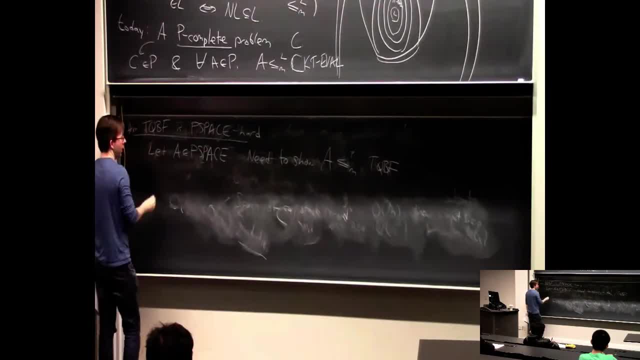 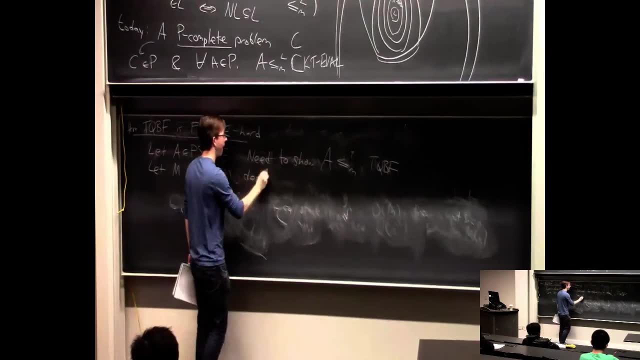 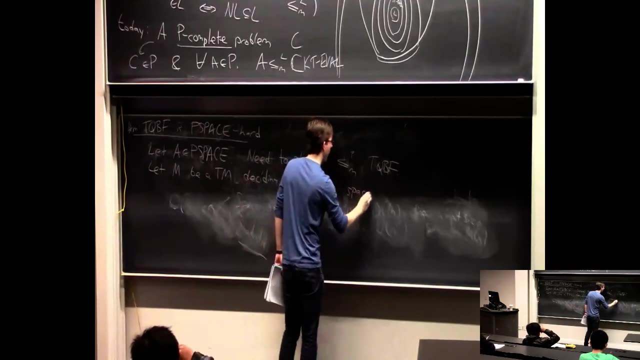 almost write themselves. We have to show this. So you know, let M be a Turing machine, a deterministic Turing machine deciding A in, maybe n to the little a space. Okay, maybe I should write A times n to the a or order n to the a. 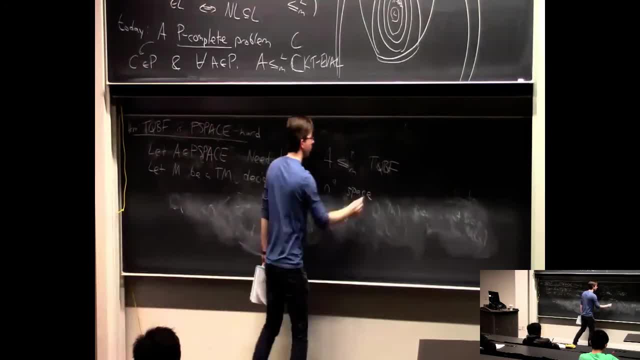 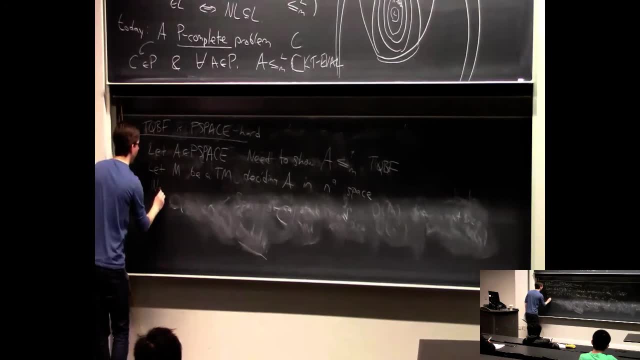 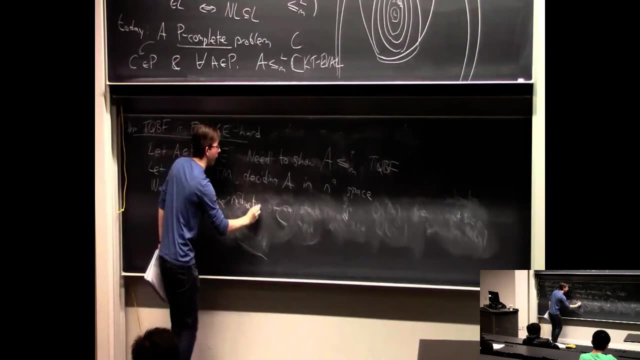 but let me just write n to the a space. Okay, so now we need to build a polynomial time reduction, So let's have a sequence of R, Or if we're really ambitious and cared, we could make it log space, but never mind. 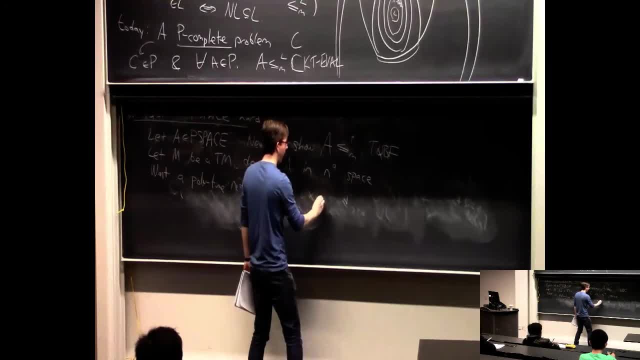 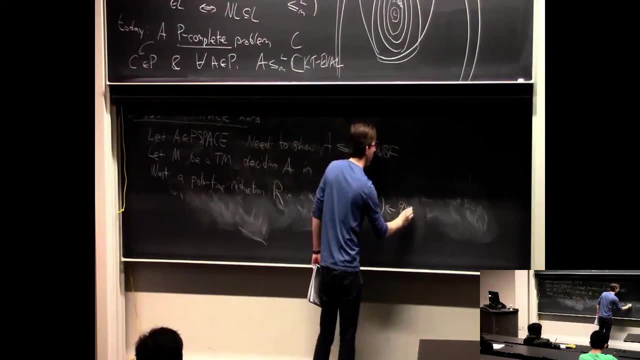 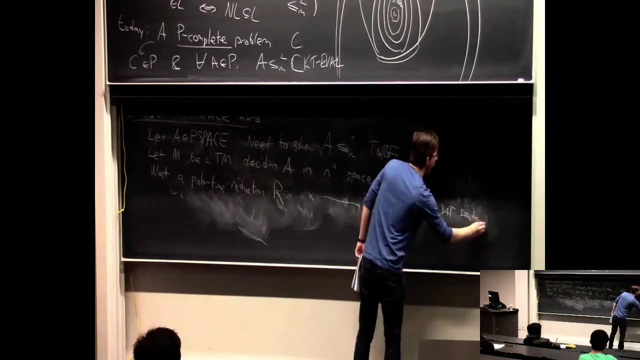 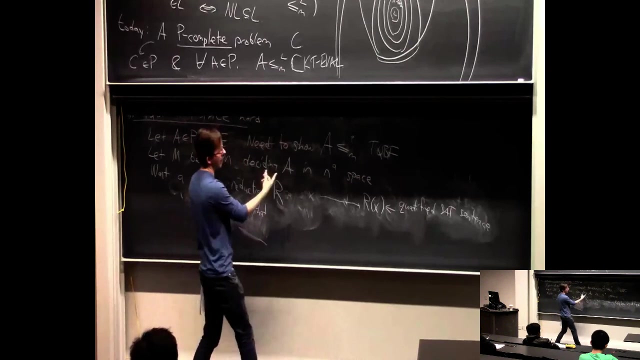 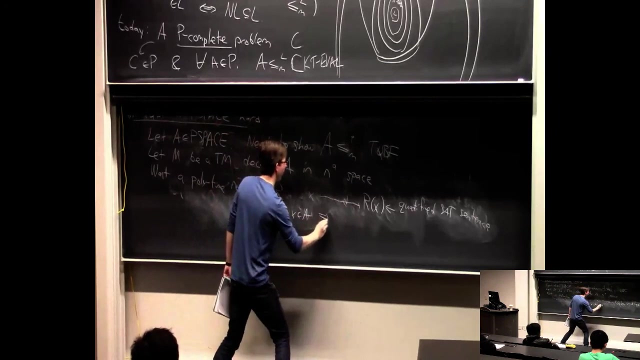 That takes a string x and maps it to some R of x And this is a quantified Boolean formula. Okay, such that, okay, x is in A if and only if, this formula is true is true. This is something with like a bunch of for alls and exists. 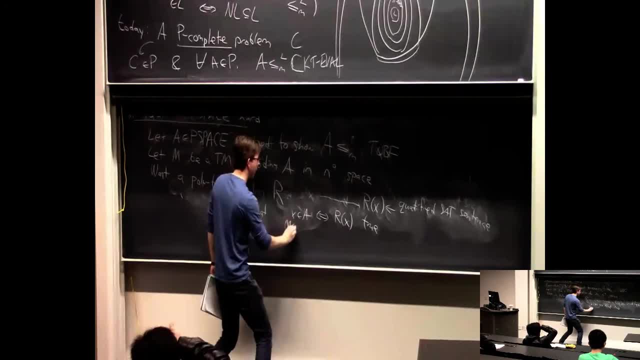 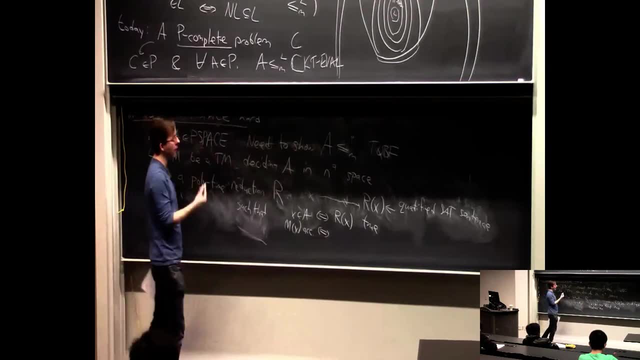 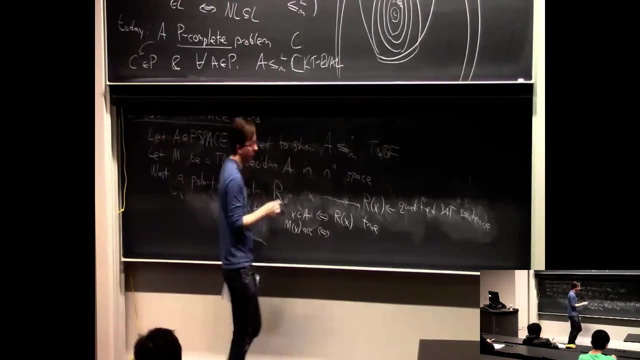 Okay. in other words, M of x accepts if, and only if, R of x is true. Okay, and R. here M is fixed. so this reduction R will depend on M. You can think of this reduction algorithm R as knowing M. so the unknown thing is x. 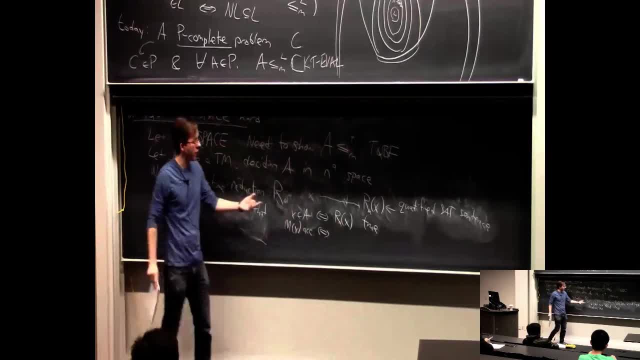 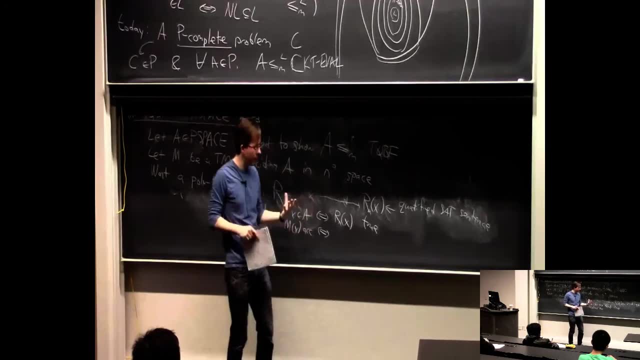 Okay, so it's going to take some string x and it's going to spit out like a very long sentence like with: for all exists, for all exists, for all exists. But okay, Itself depends on x. It's a little confusing, I guess, because you usually think of x as variable names. 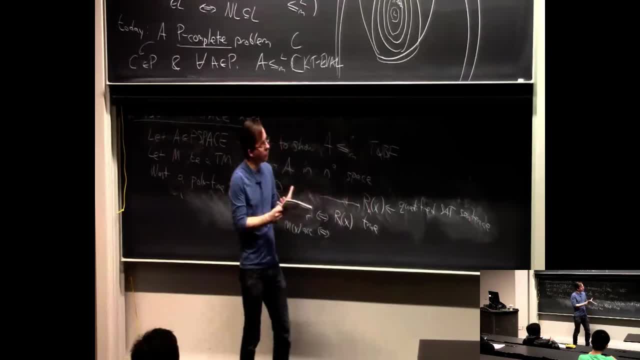 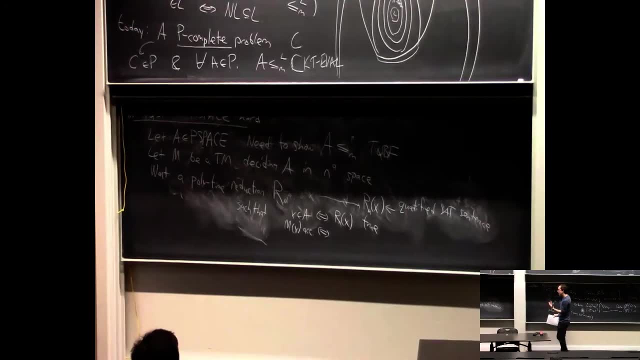 but anyway, And that sentence like for all exists, for all exists, et cetera, is going to be true if, and only if, the Turing machine M would accept when run on x. So this sentence has to like encode stuff about the computation of M on x. 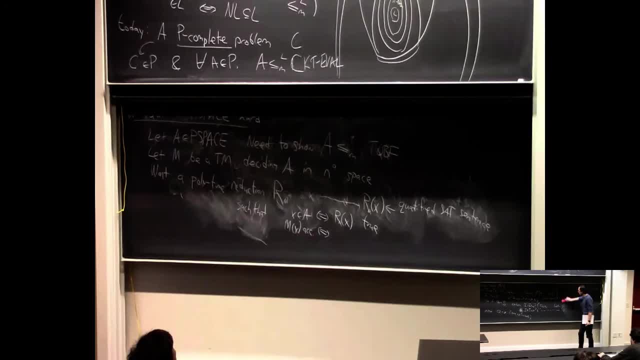 And that's not too crazy, right? I mean, that's what goes on in Cook-Levin, You know. you basically build a formula or a circuit that encodes the computation of a Turing machine on a string, and we're going to do something similar here. 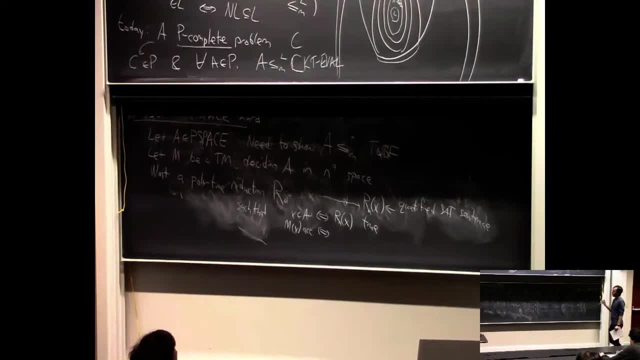 And it'll actually even be good to think about it kind of like the way we thought about it when we proved that ST path problem was NL complete. So you know, Let me just draw a picture here, Given M and also x. M has running on, x has some configurations. 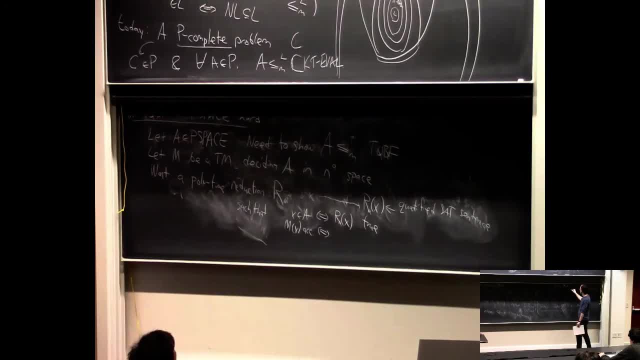 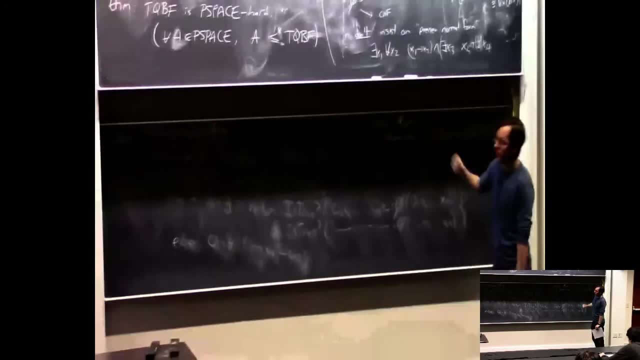 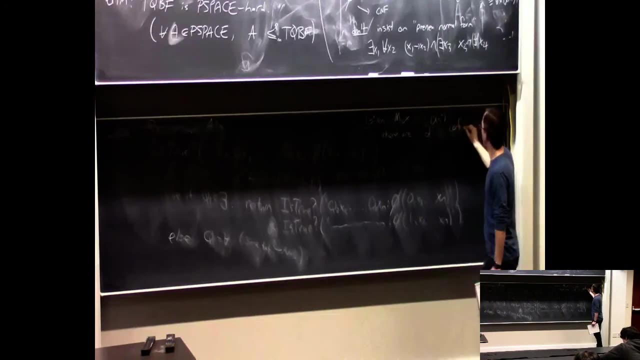 Remember, you know, back to space-bound computation and configurations. there are exponential in the space usage of M many configurations. So two to the order, NA Okay, And they really just basically all possible work tape, contents of which there are like: 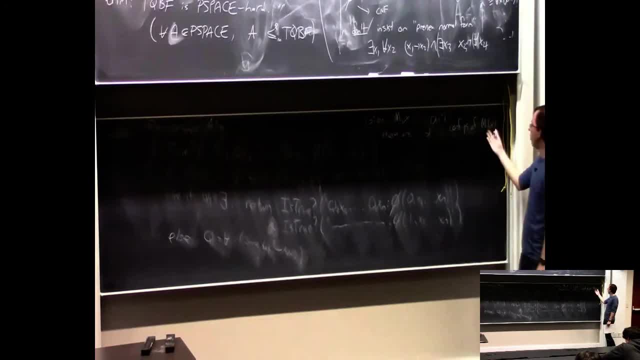 two, to the N, to the A, and maybe a little bit more information about what state M is in and where the head is pointing. And you know one is called C, start. You know this is the one that looks like Q, zero, and then x. 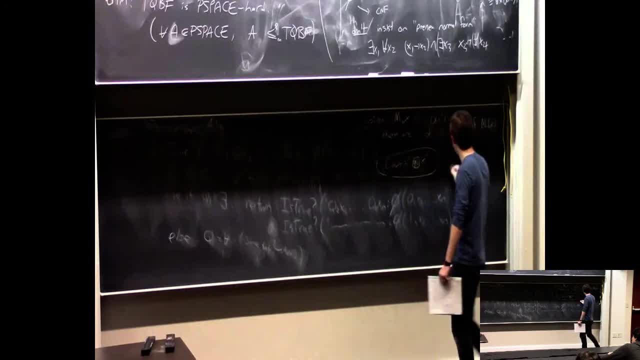 Okay, And then you know there are exponentially many configurations And actually M is a deterministic machine, So things are particularly easy, Like each configuration just leads to a next configuration under M. You know, this is really if this is C prime. this is like you know. 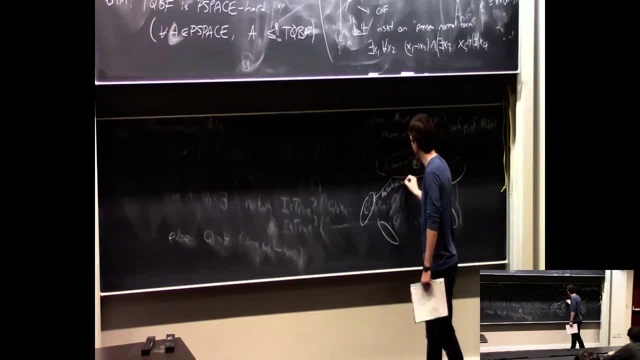 just the next configuration applied to C: start when you're running on M. Okay, So you can imagine this configuration graph And it's even easier. It's even easier than the one like when we were studying a non-deterministic Turing. 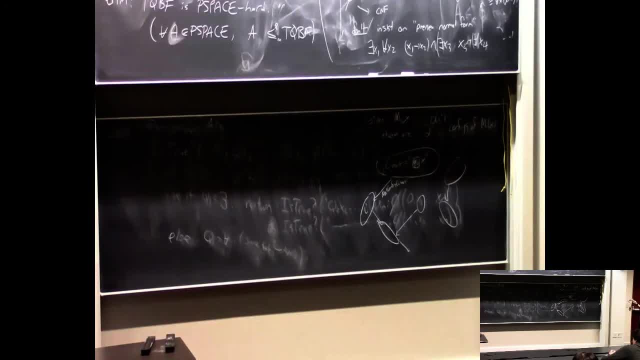 machine There, like every configuration, had two possible outcoming configurations. Here it's, you know it's deterministic, so it just has one. So we can imagine this configuration graph again: G, depending on M and x, has exponentially. 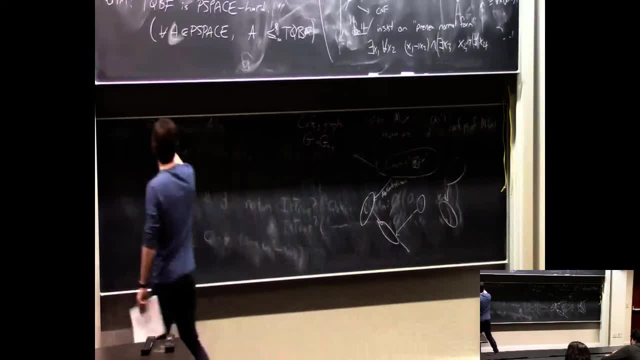 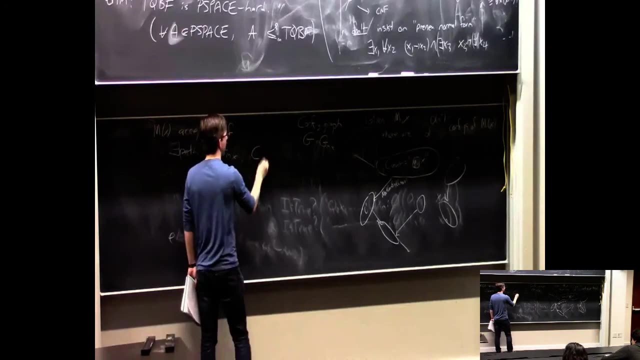 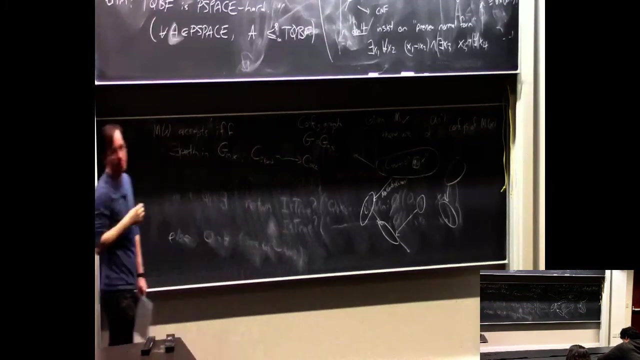 many vertices Okay. But again, M of x accepts if, and only if, there's a path in this configuration graph from C start to well, let me write: C accept. So actually just in that same as the proof, that path is NL complete, we can assume without 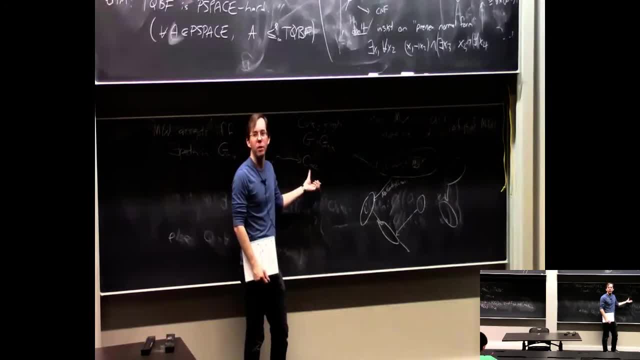 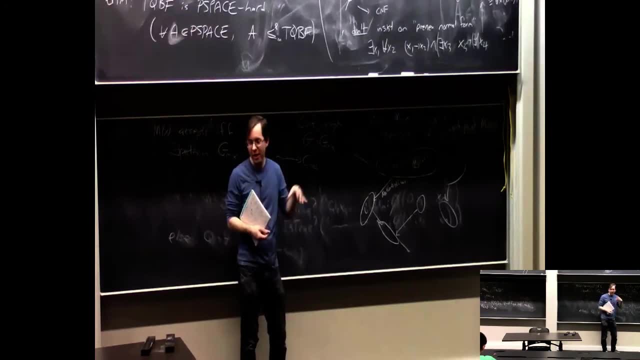 loss of generality that there's a unique exception. Okay, There's a unique accepting configuration of M on x. Okay, So we can insist that whatever M is first, we'll like fix it up a little bit so that just before it's going to accept it like cleans off the whole tape, moves the head. 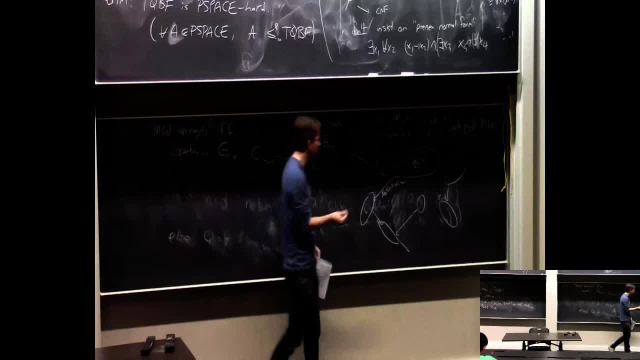 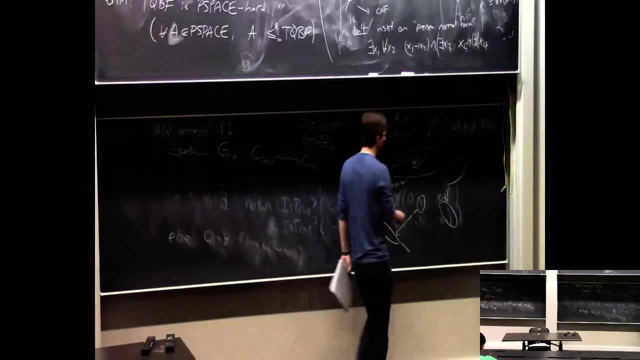 back to the beginning of the tape and then accepts. So we can assume that doesn't really change the space usage of M, nor does it change what language M decides. So just as before, we can assume there's like a unique configuration called C- accept. 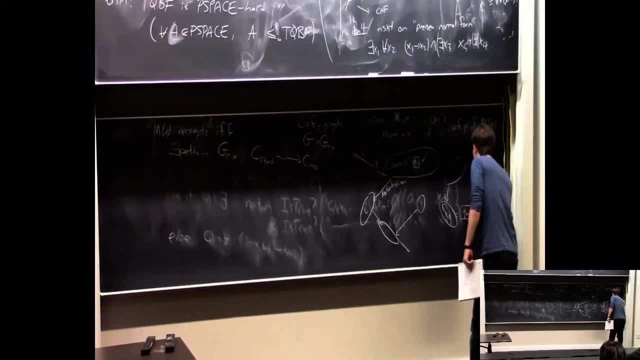 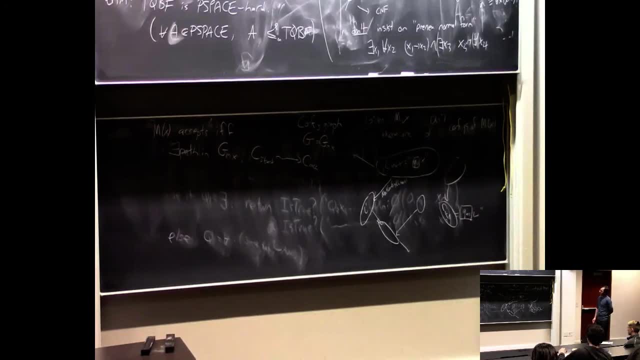 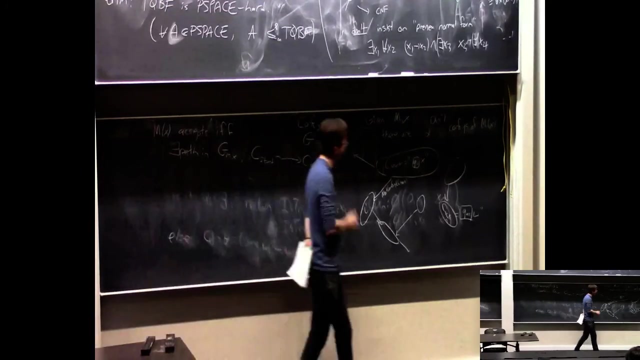 which looks like just the accepting state, Okay, And then a blank tape, Okay, So like, just like in that you know NL completeness of ST path. this reduction algorithm R knows M and it gets x as input, So we can sort of imagine this graph. 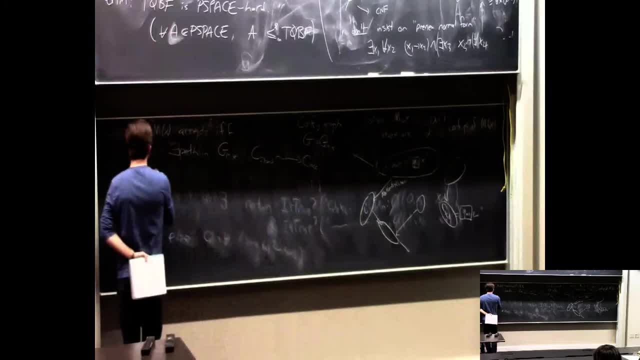 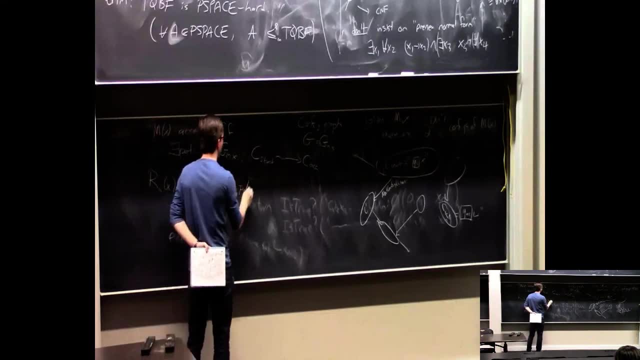 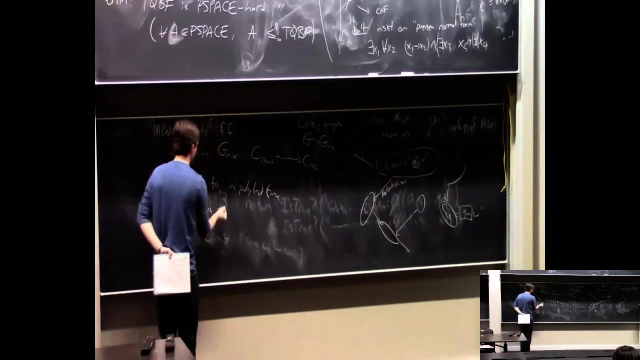 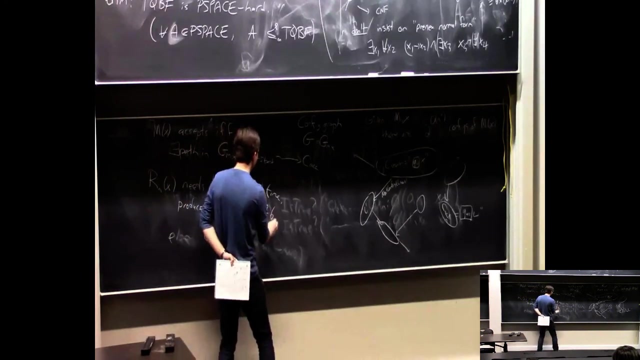 But now R of x. what it needs to do is: Okay, Okay, Okay, Okay, Okay Okay, In poly N time, produce a formula, In fact one of these quantified formulas. It's going to look like there exists, I don't know. B1 for all, B2.. 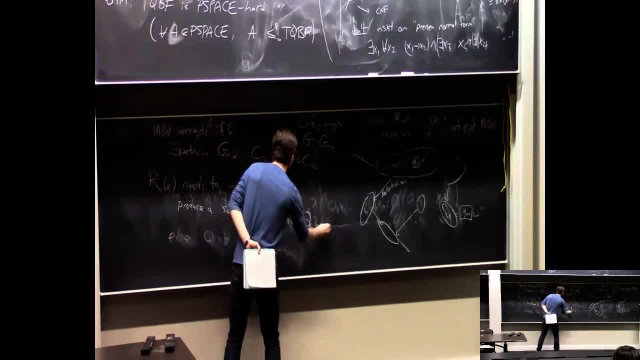 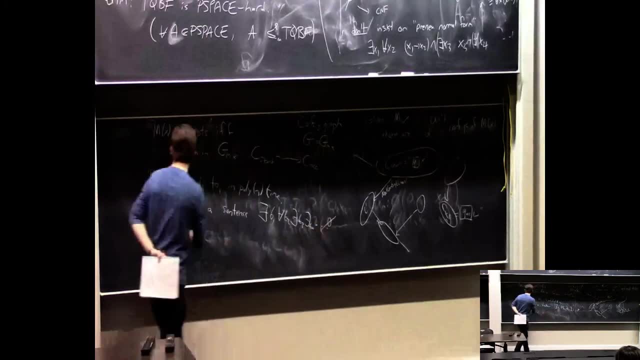 There exists B3.. There exists B4. Okay, This is going to have length, probably order n to the a, And then it's going to have length, probably order n to the a, and then some formula which is true if, and only if, there exists such a path: the 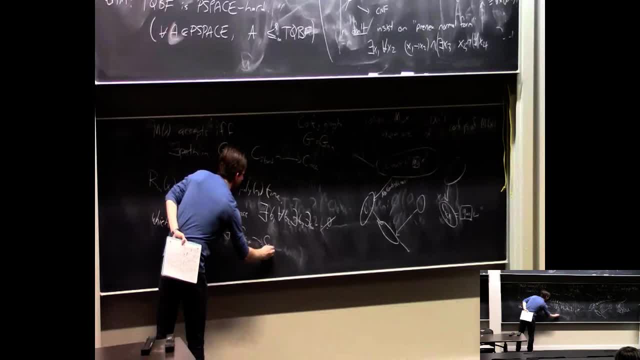 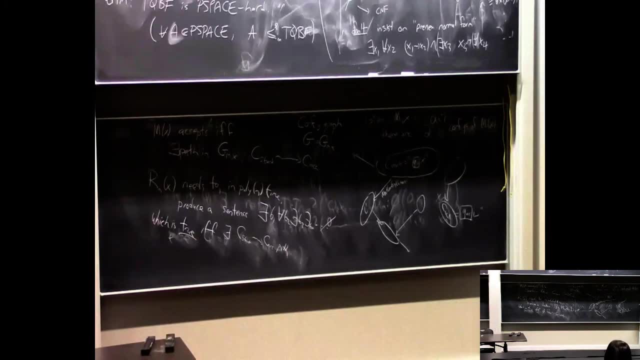 C start to C accept path, and the idea of how to make this formula is exactly like the idea in savages theorem for st path. the idea of a path exists if, and only if, there's some midpoint configuration such that you can get from C start to the midpoint in half your allotted space time. sorry, number of steps bound. and from. 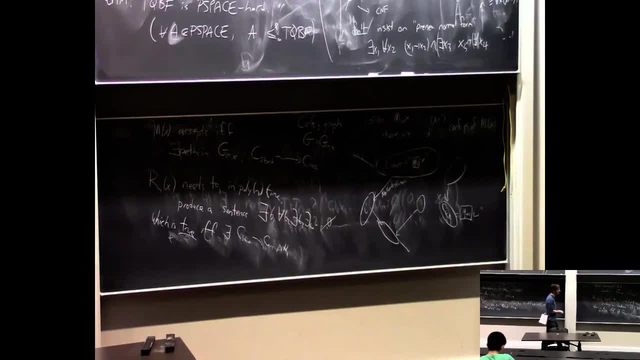 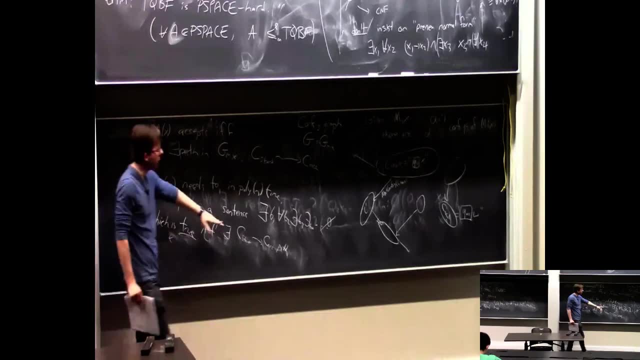 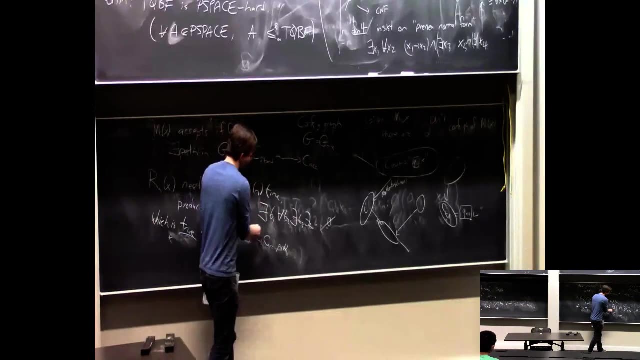 the midpoint to the end states and half the allotted distance. so this formula it's gonna have variables and these variables are gonna be bits that encode configurations. so eventually you're gonna think of: you know these exists and for all the same things, like there exists a configuration, C min.